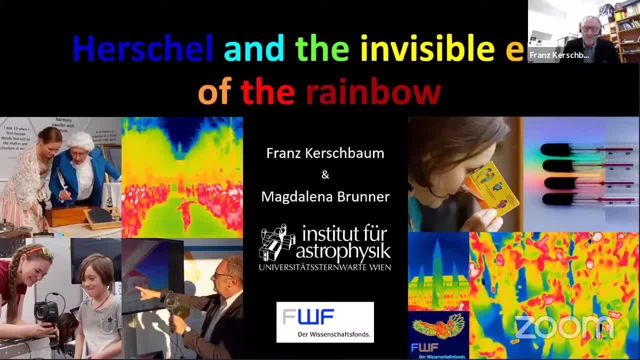 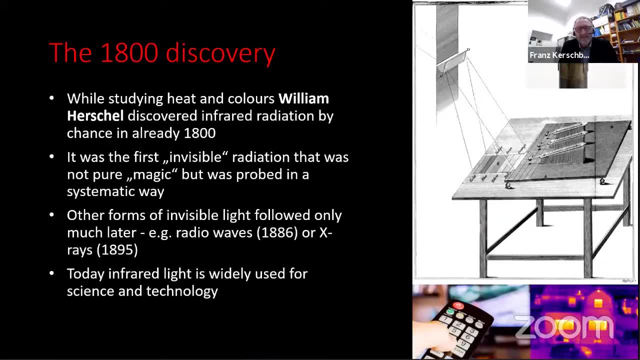 Let's start with some history. In 1800, something very special happened. While studying the heat and colors of the sun, William Herschel discovered, more or less by chance, infrared radiation with his spectroscopic experiment already in 1800,, as I said, So in principle he was measuring with simple thermometers. 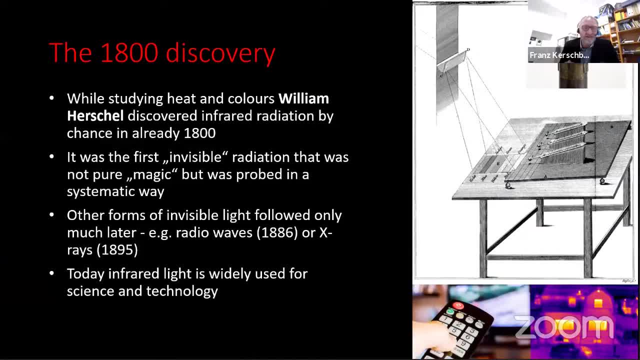 how much heat is within certain color ranges. So he was measuring the temperature of areas on the ground or on tables for the temperature And He, of course, was comparing these temperature with regions on the table that was not illuminated by light to have a comparison temperature temperature. and more or less by chance, as I said, he pointed the thermometer to a region next to the red, which was dark, not illuminated, and it was clear, obvious and obvious for him that this region was hotter than the other. so there must be something invisible. 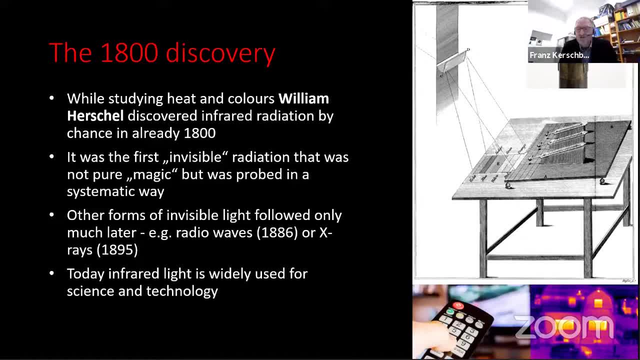 But, And, And, And. This was the first invisible radiation that was not pure magic, as all the things before, but could be probed in a very systematic way. He did optical experiments, reflections and so on. This finding was only followed much later by other kinds of invisible light, namely, for instance, radio waves in 1886 or X-rays in 1895.. 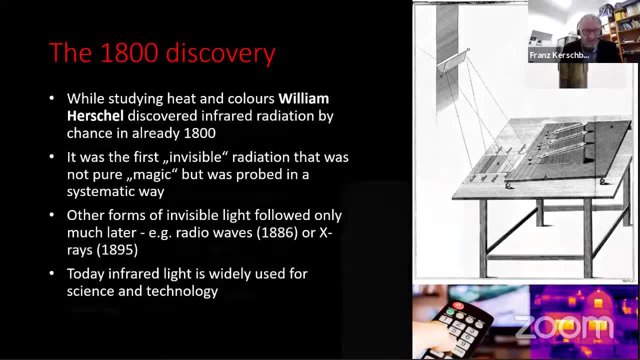 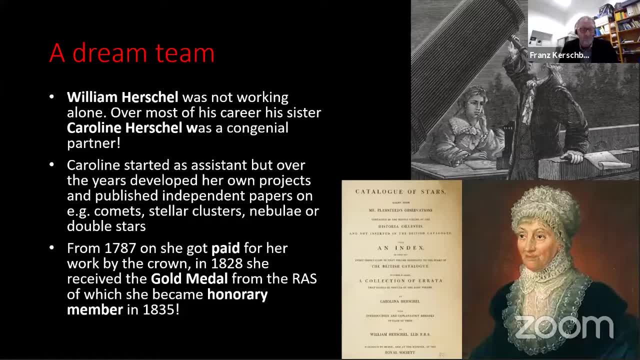 Today, infrared light is widely used and, of course, in technology and science. Herschel was not working alone, but he was working in a team together with his sister Caroline. She was starting as his assistant, but later on she published independent papers and comments to the clusters. 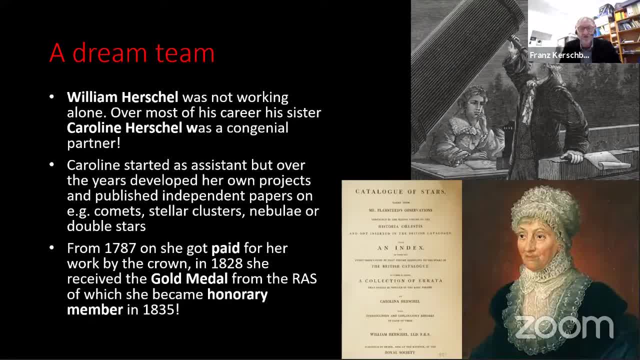 And from 1787 on she got even paid and she was the first female researcher getting paid. For example, she was the first female researcher to get paid for her research. And from 1787 on she got even paid and she was the first female researcher getting paid for her research. 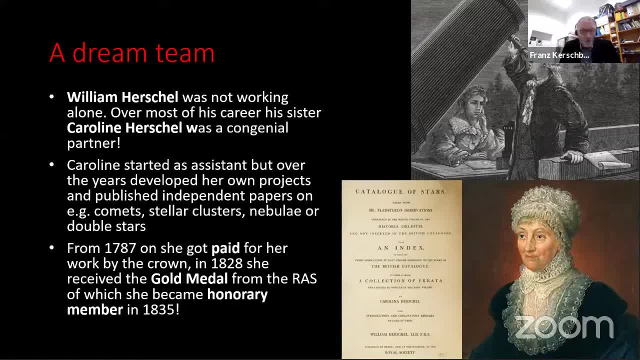 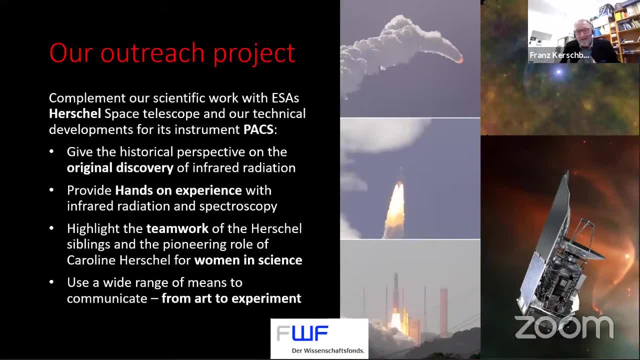 For example, she was the first female researcher to get paid for her work by the crown In 1828,. she received a gold medal by the Royal Astronomy Society and even became a honorary member. later. Our outreach project was thought to complement our research done with ESA's Herschel Space Telescope. 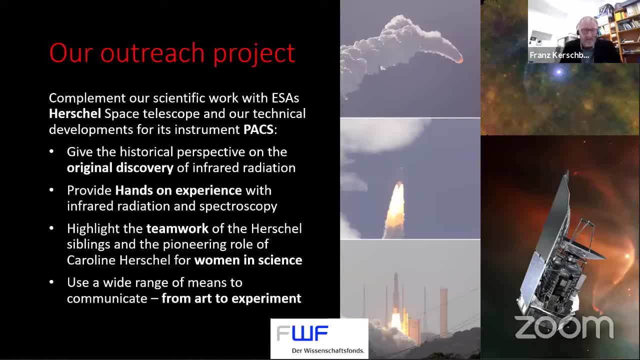 where we contributed science and also technical components to one of the instruments And we thought a historical perspective on this discovery is something good For outreach and education. we wanted to show also experiments And- very important- we planned to feature Caroline Herschel's role as a role model for women in science. 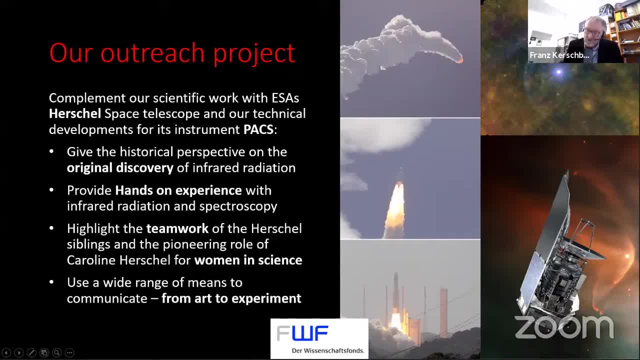 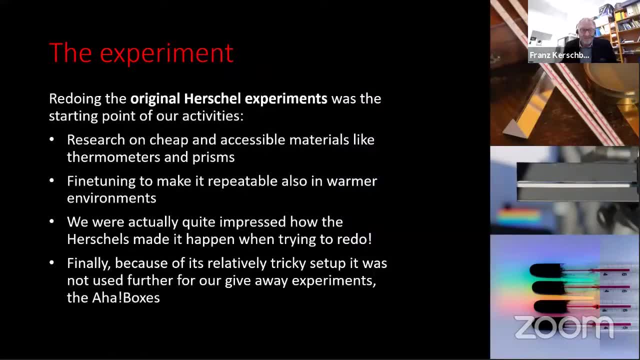 and also to show that teamwork is important, And we have chosen a quite broad range of means to communicate, from art to experiment. So the first step was, of course, to redo the experiment itself. It turned out to be quite complex. It was not really easy to repeat it because the changes in temperature, with such a simple setup. 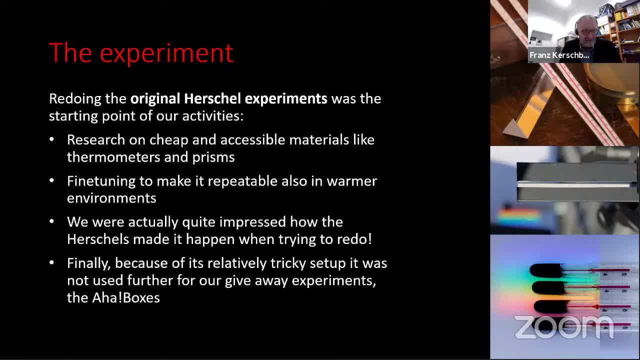 are only a few tenths of a degree Celsius And that's not that easy to measure. So we were quite impressed what the Herschels achieved that long ago. First we thought we will use this experiment as a giveaway experiment to kids, for instance. 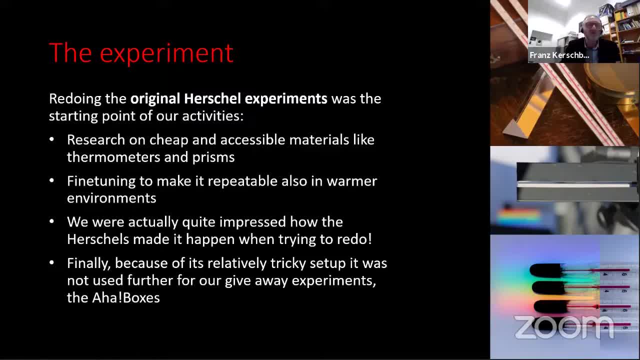 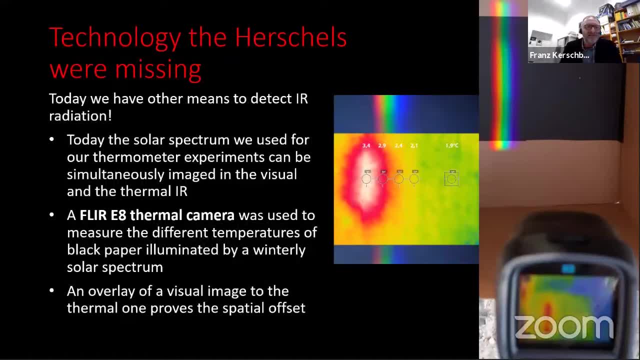 but it turned out to be complex, Too complex and not too easy to reproduce. We were successful, but it was not that easy. So what did the Herschels miss at that time? Today we have modern infrared cameras, So we also did experiments with an infrared camera that we can use, for instance, in school outreach. 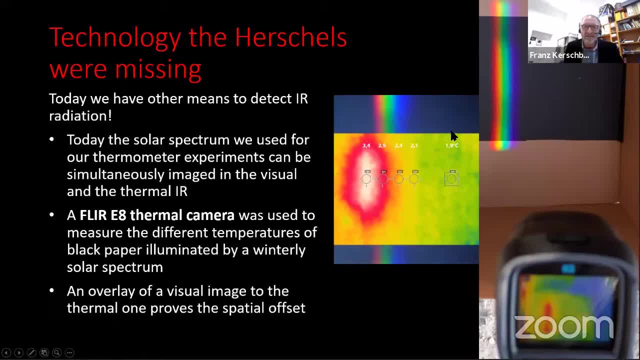 And we made these pictures where you see the rainbow of the norma from the spectrum of the sun. And if you overlay this, this image of the rainbow produced by the prism with a thermal image, you see immediately that the temperatures are higher in the dark area next to the red part of the spectrum. 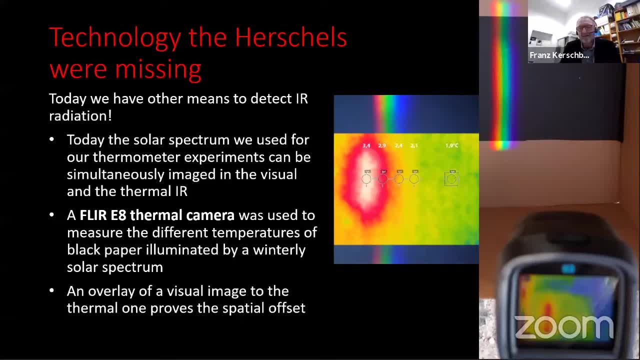 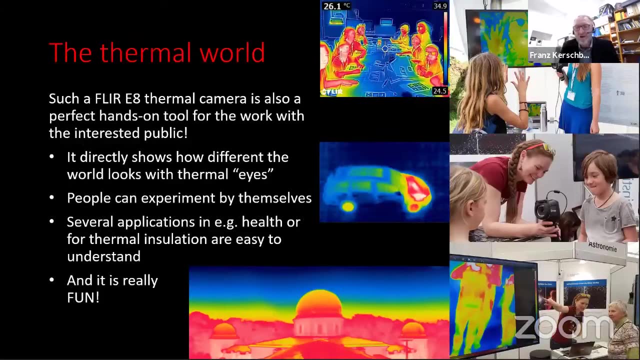 So nowadays it's very easy to show that the significant part of the energy that we receive and is split up by prism is in the infrared region and can be imbedded in the spectrum. So we use this camera a lot with our work with kids and at science fairs and show them how different the world looks with thermal eyes. 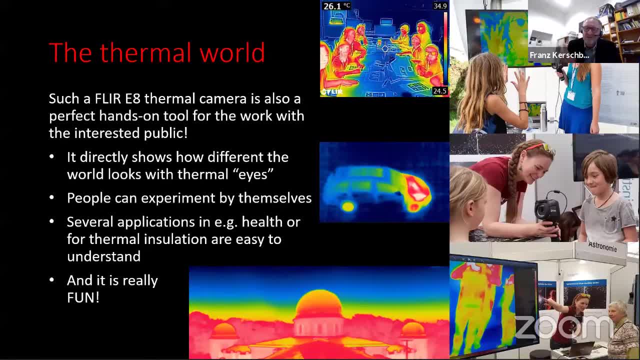 You see here a car or the kids standing and doing their work And you see Magdalena giving the camera to kids and they experiment themselves and see how different the world looks like. It's really fun and motivating to do your own research. But that was not everything. 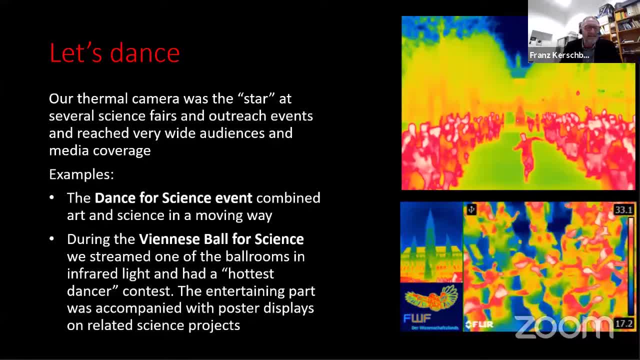 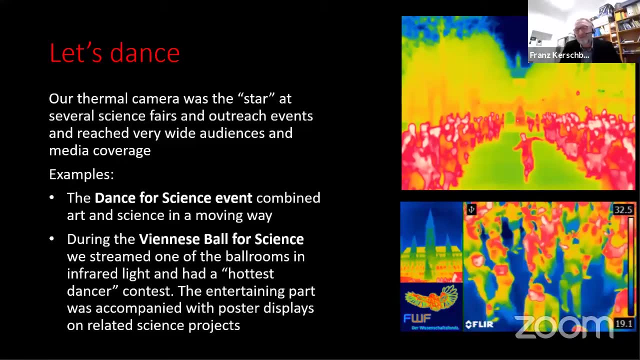 We use this camera also as the star in several science fairs and outreach events, For instance, in the course of the Dance for Science event. it was a worldwide event. during the March for Science, We streamed the dancing events in the infrared And also, of course, I'm coming from Vienna. 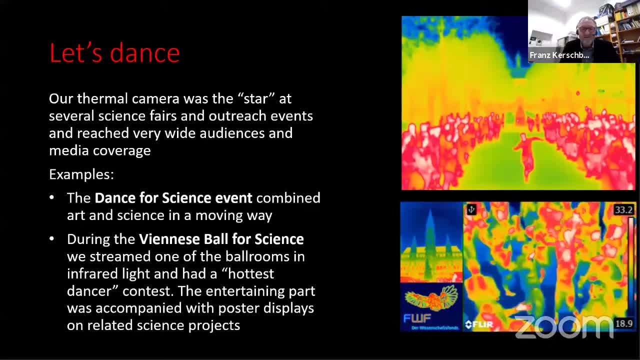 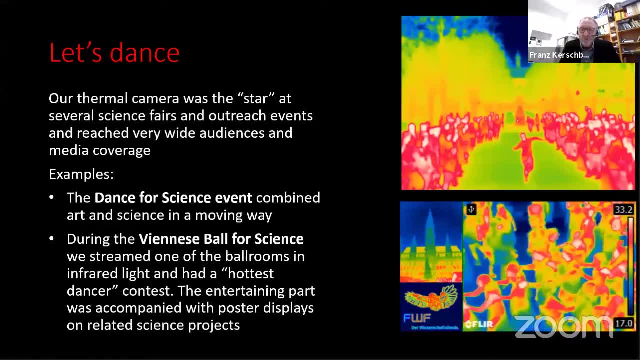 We have balls. The Viennese ball for science was also used to communicate Infrared research and we streamed out of one of the ballrooms and you see the dancers here building a line And we had a hottest dancer contest where we could communicate how interesting infrared radiation is. 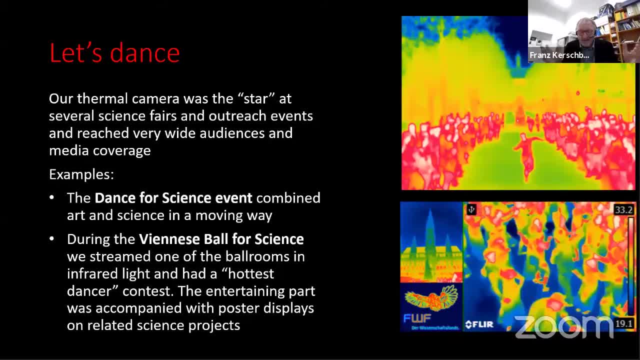 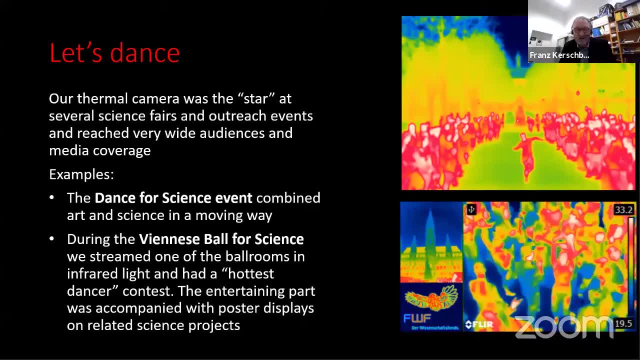 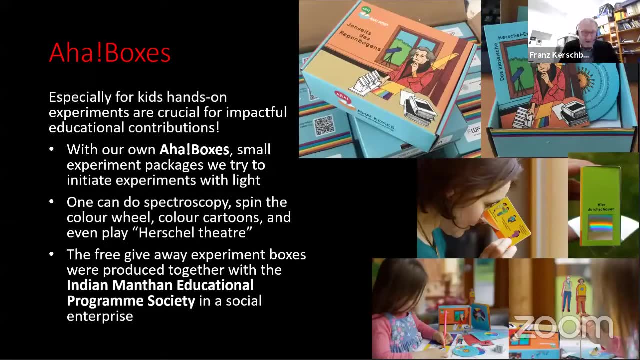 And, of course, next to these ballrooms we had some displays where we showed the science that can be done with infrared radiation. So an interesting mixture. So We started at the beginning to have some hands-on experiments- I told you already- with spectroscopy and so on. 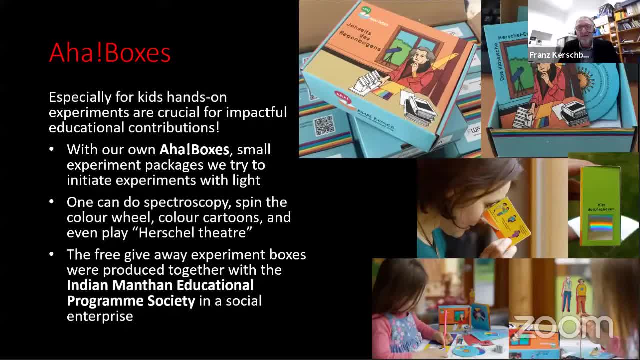 And we built aha boxes called Jenseits des Rainbows- So next to the rainbow, with cartoons inside. You can do hand spectroscopy, You can do spectroscopy in the sun. You can build everything yourself. You can color books. You can spin a clock. 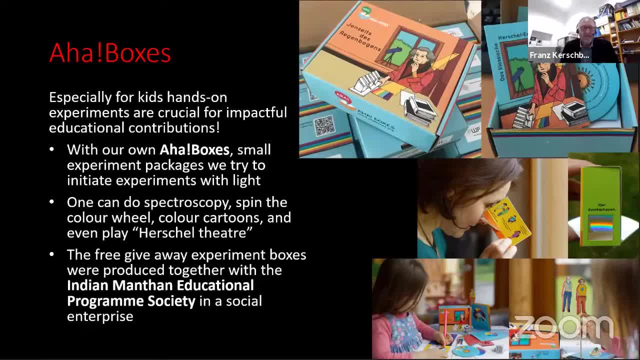 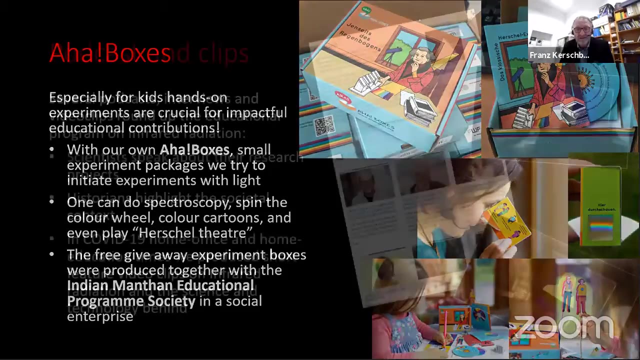 You can spin a color wheel. And we developed these experiment boxes in Vienna And they were produced together with our partners, the Indian Mantan Educational Program Society in a social enterprise in India. So this has also this side component And these boxes are available both in German and English as all our outreach and educational material. 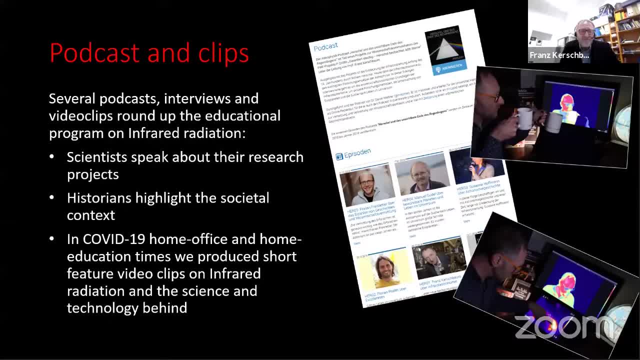 We produced several podcasts, clips, movies. Now in COVID-19 home office and home education times we produced little videos. Teachers can show to the kids online how infrared radiation works, How you can, for instance, measure the temperature of two glasses filled with different temperature fluids, and so on. 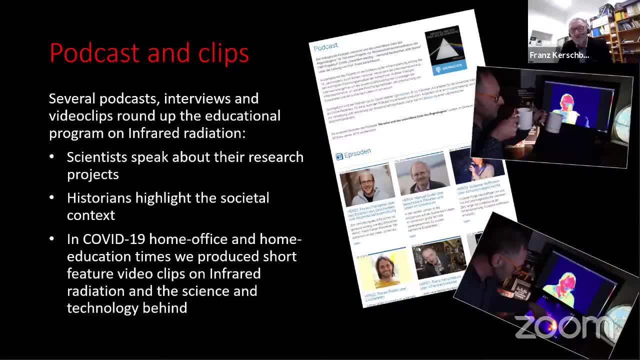 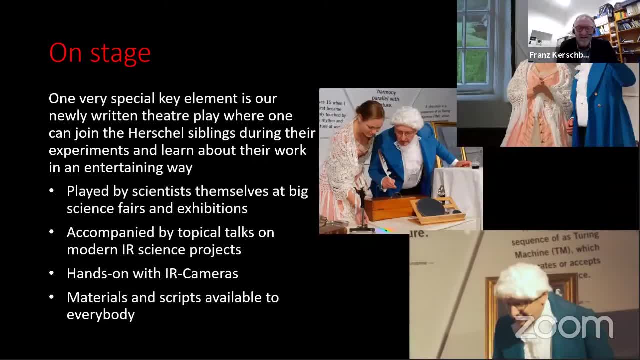 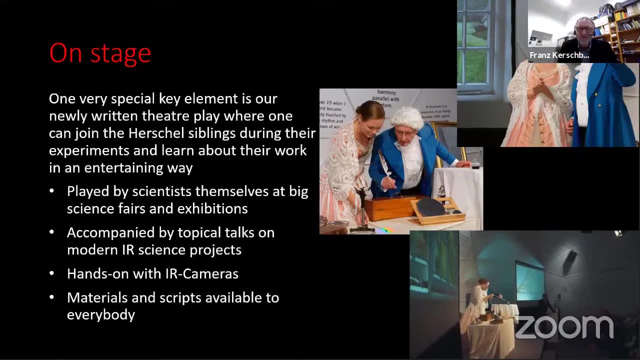 So this was quite interesting And you have many downloads available on our next website, On our websites. I will tell you later on, Of course, the highlight- I would say the outreach highlight- of our educational project was a theater play. We wrote, together with some authors, a theater play on the Herschel experiments. 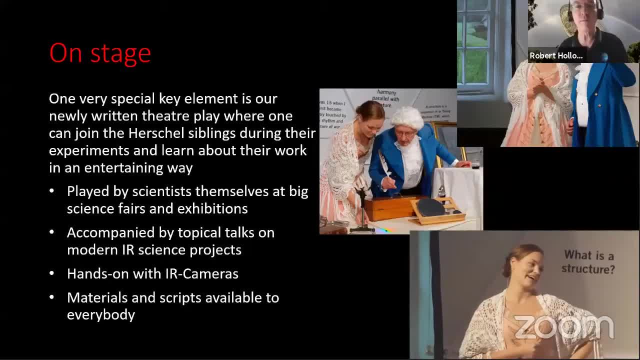 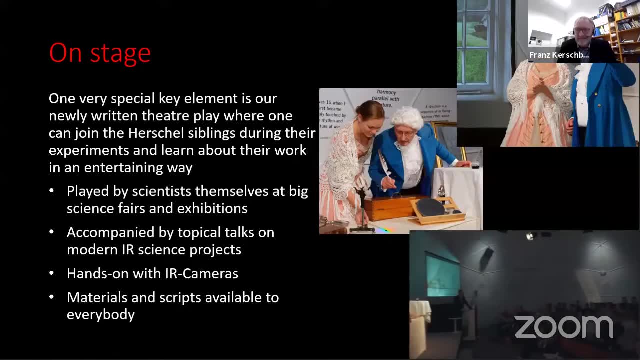 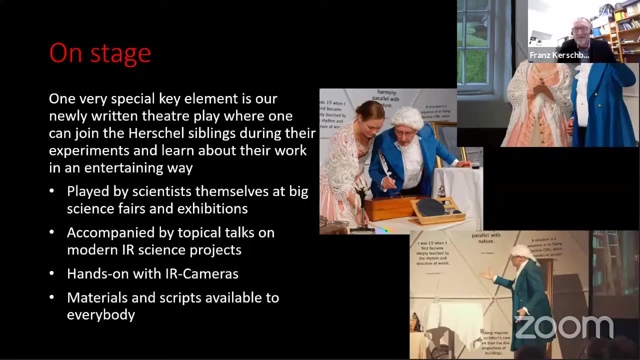 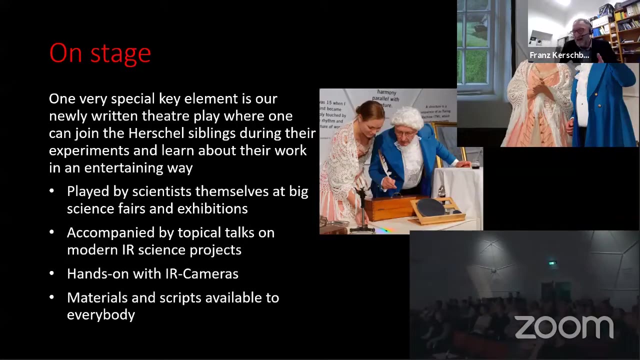 Two minutes, Franz. Yeah, On the Herschel experiments. It's quite entertaining And the play is done in a way that the scientists themselves can play it. Yeah, We did it at big science fairs and exhibitions And you see here, Magdalena and myself costumes as the Herschel siblings and playing this. 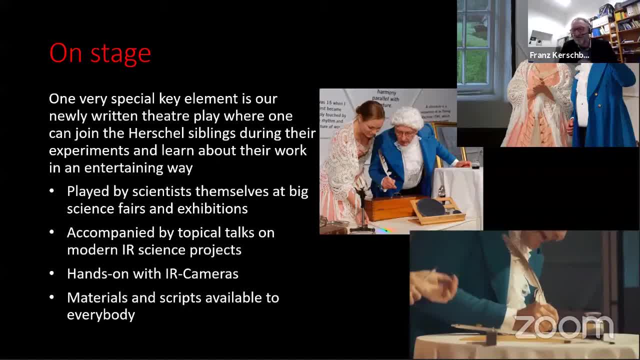 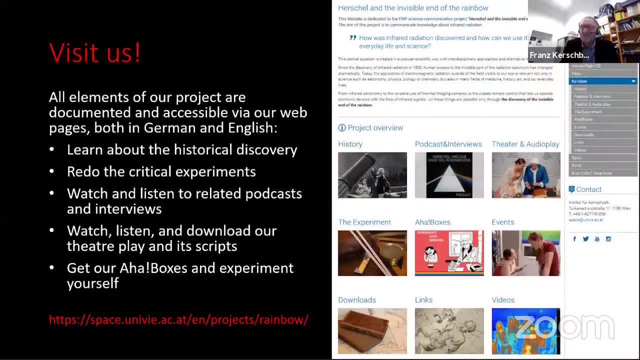 And after this we gave some talks on infrared radiation, used the infrared cameras for the kids and the other audience to experiment. You can visit us, You can download all these materials, For instance the theater script, Also in English and German. 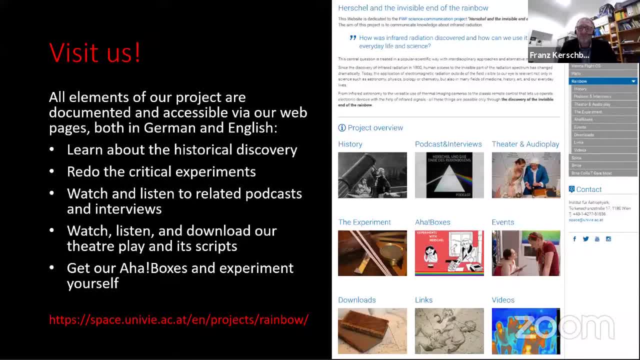 From our web pages. You can contact us if you're interested in the hard boxes. Our Indian partners are happy to help you in this regard. You can build your own hard boxes. They turned out to be quite nice as a giveaway. They turned out to be quite nice to give it to school classes. 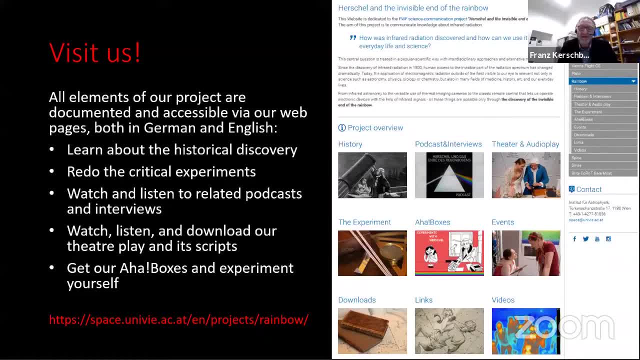 The teachers are very happy to use them for experiments, And in the meantime, we have such boxes also for other topics, For instance in biology or the moon landings and so on, Astronomy experiments and so on. So visit our web page. 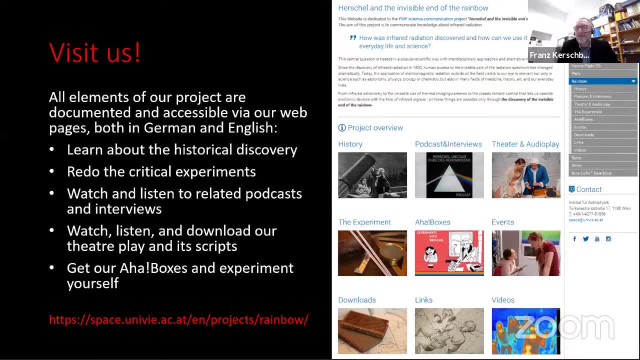 We are happy to inform you And thanks for listening to my talk. Thank you very much, Franz. Perfect timing. So we'll move on to our next speaker now And we have a question And we have Sarah Ricciardi. I hope I pronounced that correctly. 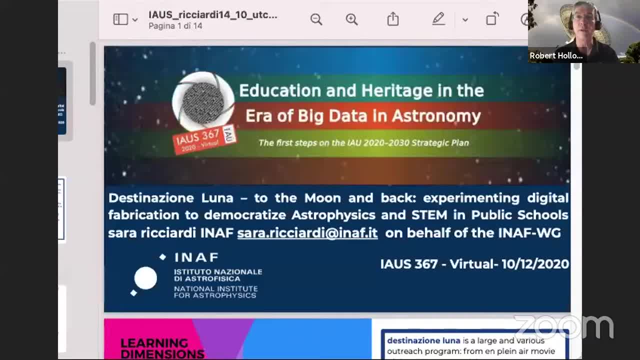 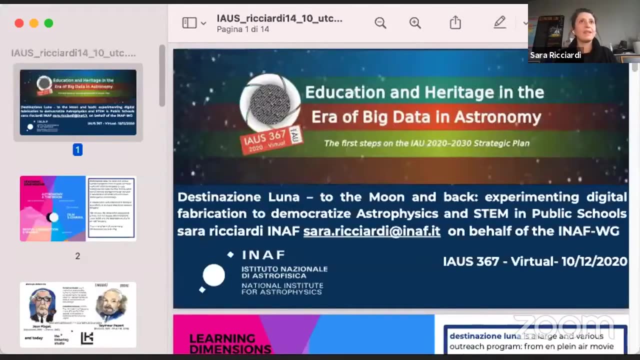 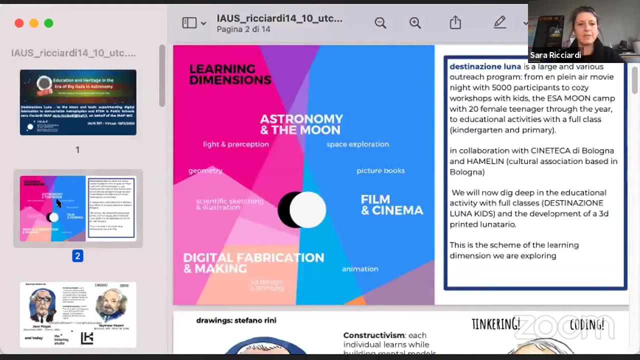 From INAF in Italy. So, Sarah, if you're there, Do you see my screen? We do, Yes, Okay, Great So, Oh, Okay. So I'm going to talk about Destinazione Luna. I'm working at INAF, actually. 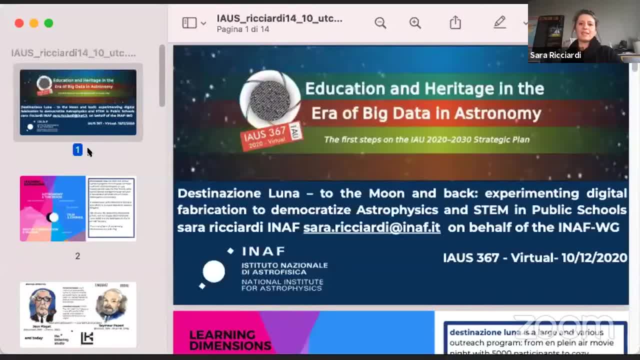 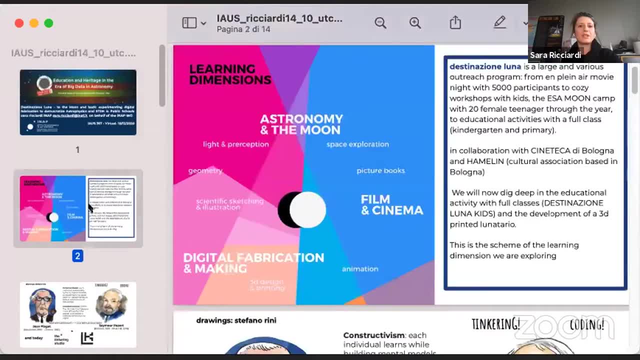 I didn't see that In Italy And the talk is it's on behalf of actually a large group of people that I need to acknowledge. So Destinazione Luna is a large and various outreach program, from a movie night with 5,000 participants to cozy workshop with kids. 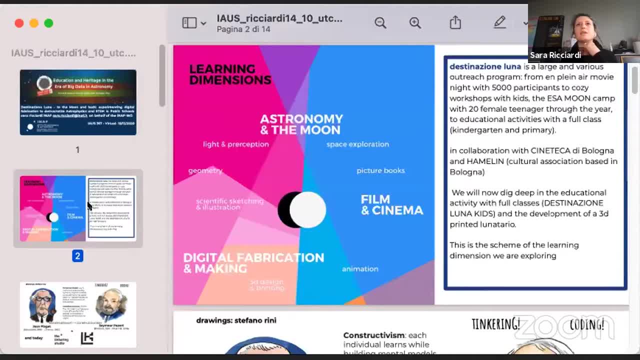 And we're doing the five-day camp, We're doing the summer camp that we run with 20 female teenagers through the year, And educational activity with full classes. So kindergarten children and primary. And everything was done in collaboration with And the Amelin, that's a cultural association based in Bologna. 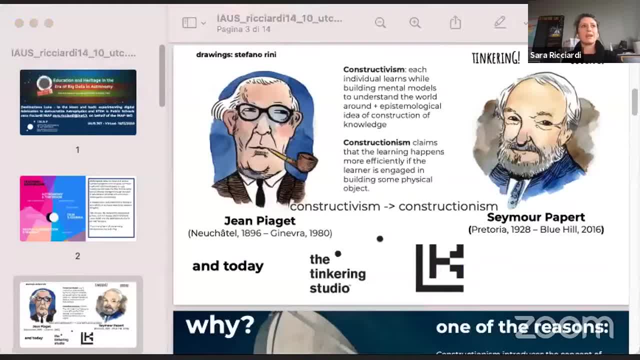 And now I will talk just about Destinazione Luna kids. So the educational activity with full classes. I'm just going to flash this slide to let you know our models in the past and people that we look at today. so, for example, the tinkering studio in at the exploratory in san francisco and the lifelong 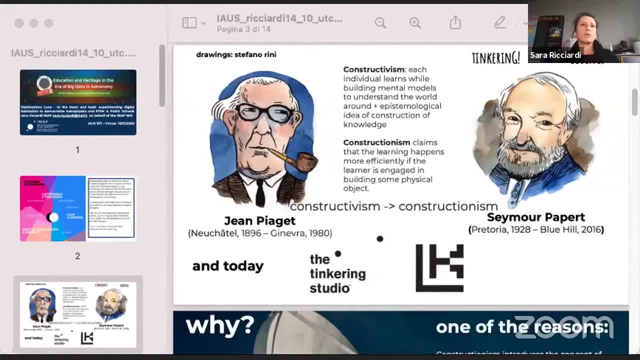 kindergarten group and for us it's very important of, of course, the work of seymour papert that, as is as constructive, is centered the attention on the learner and this process, but also claim that the learning happens more efficiently if the learner is engaged in building some 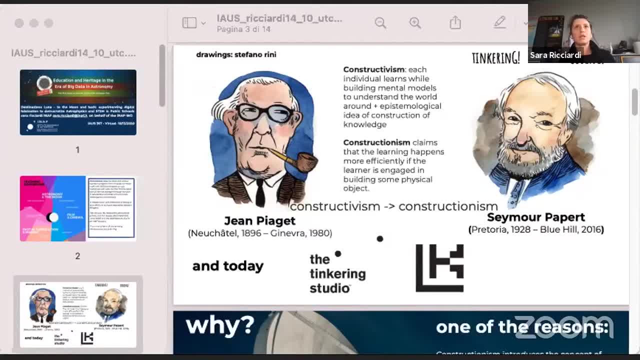 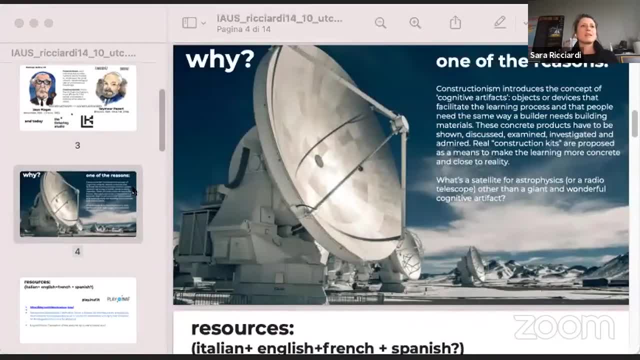 physical objects that can be physical, physical or virtual. so okay, so of course, this, uh, this idea resonates on me as a scientist also because introduce the concept of cognitive artifacts that are objects or devices that facilitate the learning process and that people need. the same way a builder needs building material, so 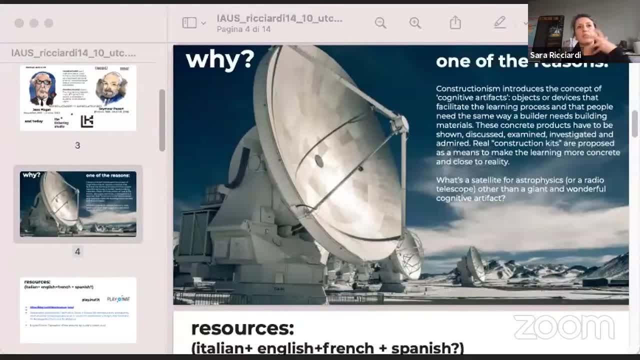 those concrete products of, of, of be designed, shown, discussed, examined, investigated and also admired. And I'm wondering: what's? what? is a satellite for astrophysics? or, for example, a radio telescope? This one is the antenna of ALMA, and actually I really love this picture because we are also building a band 2 plus 3. 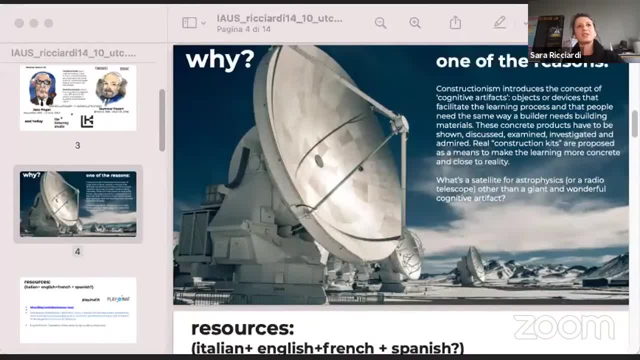 receiver right now. so, but all this stuff are just a giant and wonderful cognitive artifact that actually we use to understand our world. So this pedagogy really resonates with me as a scientist, not just as an educator, because our community works like that and I really 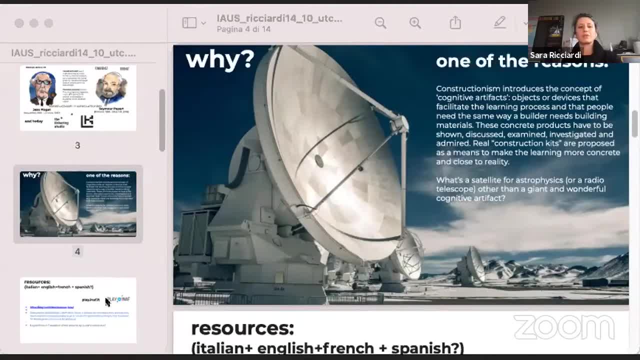 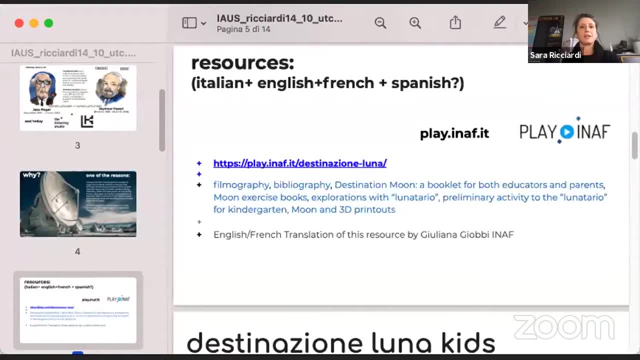 hope to give, to provide the chance to, to let kids understand also how our community works, not just you know the literacy related to that. So all the resources are are online and actually the resources natively are in Italian and then, together with other people, Latina- Juliana Giobbi, for example- we translated in English and French and I think this is the 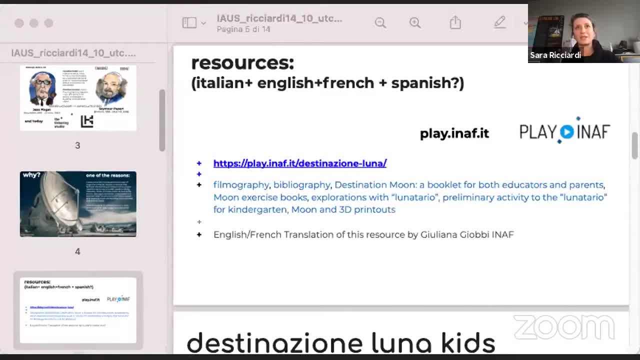 perfect audience to ask if someone wants to translate in Spanish. of course I will be happy to provide everything, because it would be super nice to have it in Spanish too and also other languages. and we got filmography, bibliography, a booklet for both educators and parents, some activity about drawing the moon on exercise book, some exploration with the. 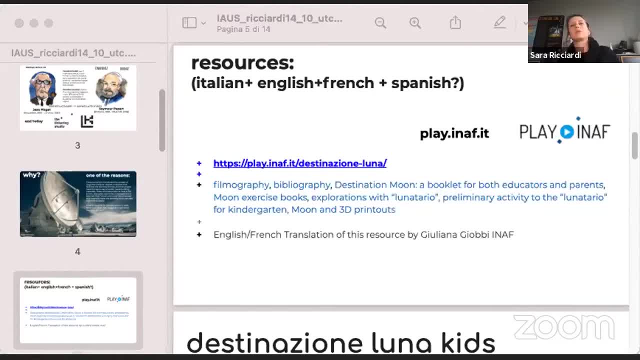 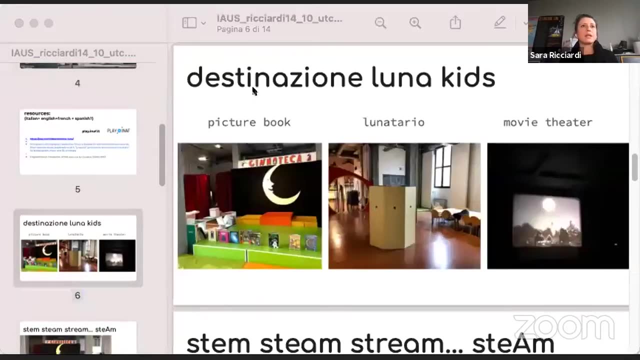 Lunatario, some preliminary activity we designed together with the kindergarten teacher that has preliminary for, you know, for very young children, and then also the moon and 3D printouts for the 3D printer. So Destinazione Luna Kids is organized in three moments. so a first and welcoming. 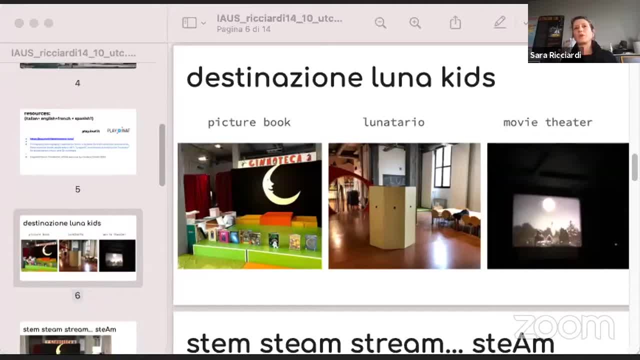 approach with the picture book and we read the. we read the book and we chat with children, then the Lunatario exploration and finally the movie theater experience. Depending on the age and number of pupils, we split the class into group, half working at the Lunatario and half working at. 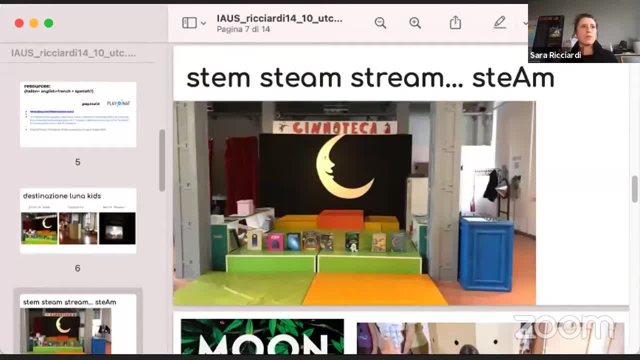 and half watching the animation. So the classical definition of STEM as a science, technology, engineering and math used to group together those considered the hard science has been often by the acronyms STEAM. So A is for artists. basically represent the need to use those. 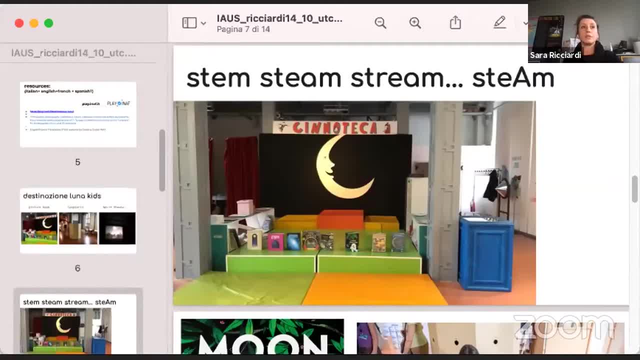 disciplines as a true form of self-expression and so self-determination in your own learning. I believe science itself can be a powerful way to express yourself, but definitely expressive languages are less rigidly coded and are more immediate, so they help. Another reason why not to segregate STEM discipline from art is the audience. Children are still not so affected. 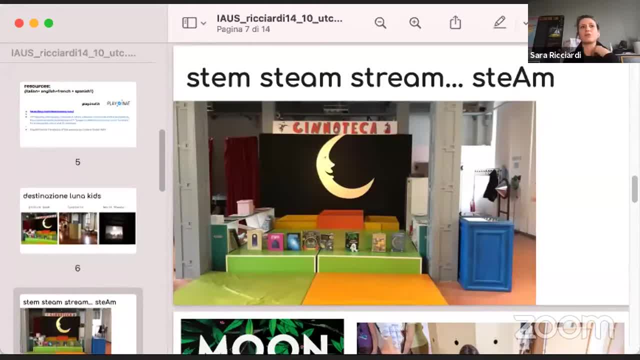 by the useless atomization of knowledge in disciplines, and they often learn in a learner desk fashion without worrying too much about discipline. So recently, with the proposal of STEM, we had one more layer. so R is for reading and writing, and advocates of STEM see literacy as 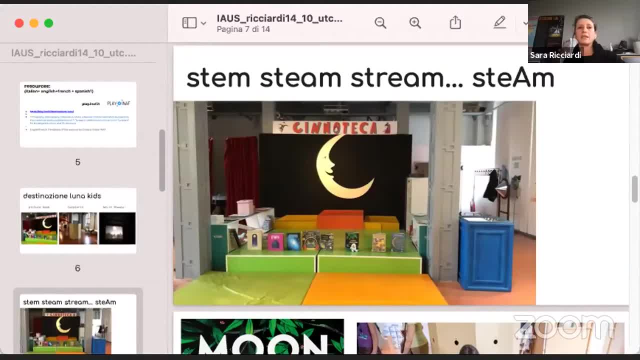 an essential part of our well-rounded curriculum, as it requires critical thinking as well as creativity. This, of course, may be true, but we connected STEM and reading for other reasons, because in our previous experience we found that using a familiar object such as a picture book can. 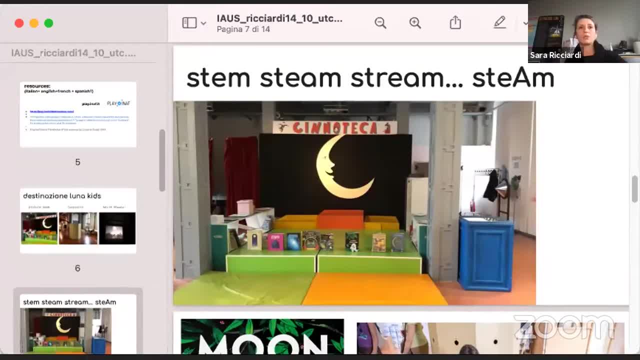 spark the initial interest through a familiar and well-known object and also will help to keep a very short psychological distance between the children and the scientists or the educator. So the picture book is, in our opinion, the perfect object of transition from a familiar and protected world to the realm of STEM. that, for someone, can be intimidating We want to definitely avoid. 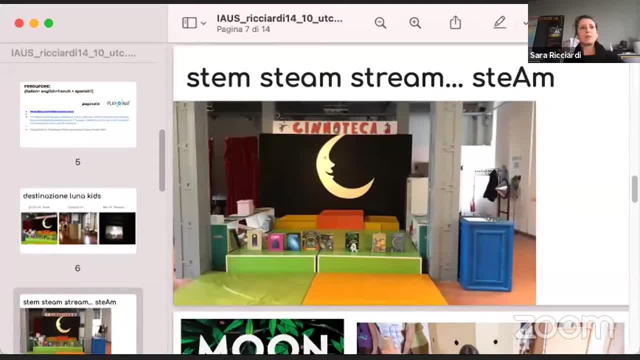 the feeling or wonder of excitement that happens when people get to explore astrophysics will become a sort of psychological border. We believe, in fact, that this wonder is something that is not always positive for everyone in the classroom, not because those feelings are negative per se, but because children could feel they are. 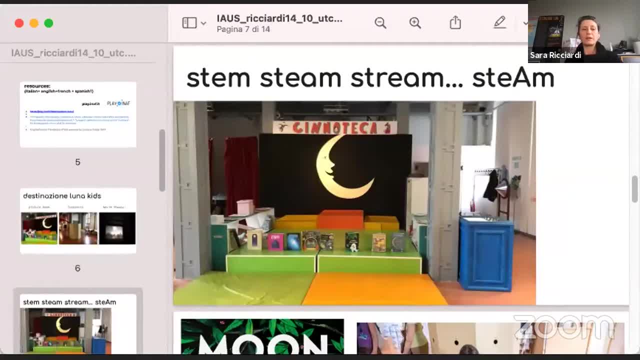 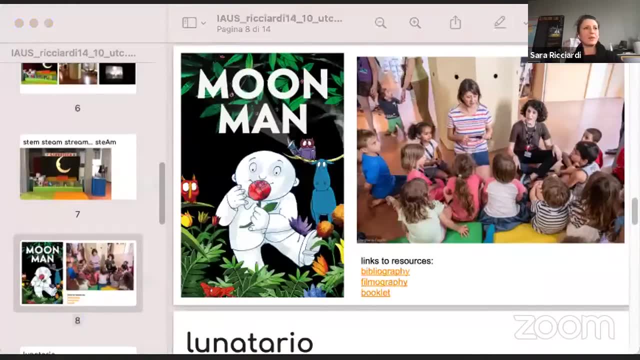 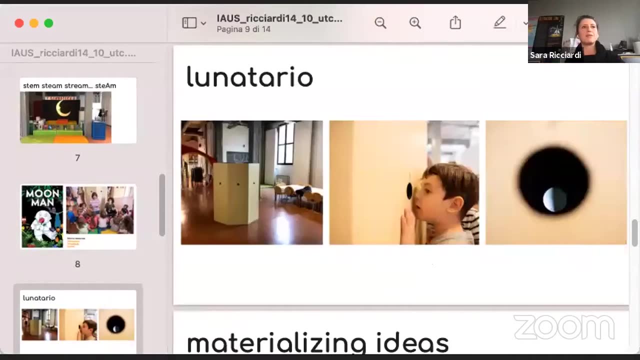 not smart enough to be involved in such a wonderful but maybe distant idea. So, okay, I just I think I will flash this slide because I don't have time, and I'll show you the picture. So this is the Lunatario itself. The Lunatario is a big octagonal wooden box with 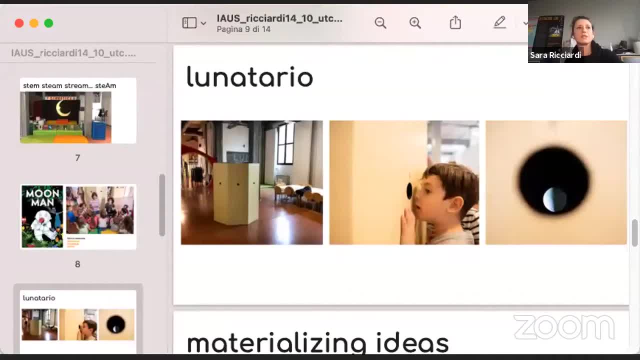 eight peeping holes to visually explore a 3D printed white moon fixed on the ceiling with a fishing string, so in the dark it would appear suspended. The facilitation of this activity is very light, playful, child-centered, to allow a personal and meaningful discovery. 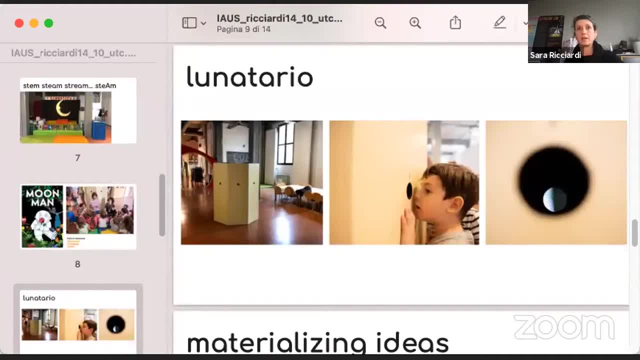 and is based on the idea of building a micro learning community where children can learn also from peers, With enough time for exploration, and this is actually really needed. the children will be able to see the distance of the relative position between the sun, the torch and the. 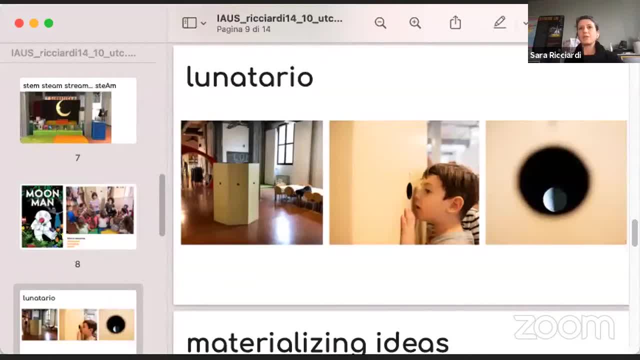 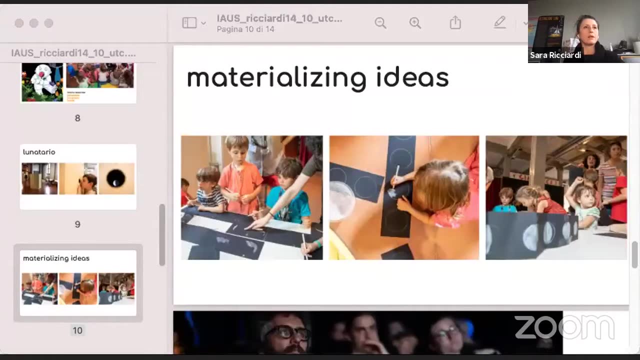 observer. We dig deep in this concept, allowing different solid figures in the Lunatario when we prototype a 3D printed version of the Lunatario. And also- sorry, I'm a bit in trouble, You can, Okay. So we used some craft materials to materialize the concept and think a bit away from the box. 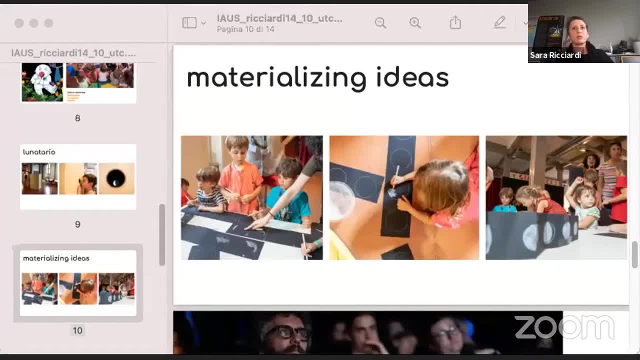 For this purpose, we provided black cards and white pencils so the children could choose to reproduce one or more moon faces, and this reflexive gesture was integrated, as needed, with new observation of light. drawing with an eye on the Lunatario and an eye on the drawing. 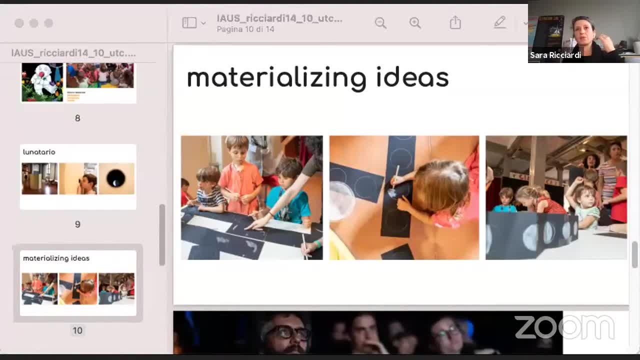 With the youngest. I'm talking about four years old, five years old children. this was very important because the concept of right, right, left, up down dark light might be not yet consolidated, So we observed that. Two minutes, Sarah. 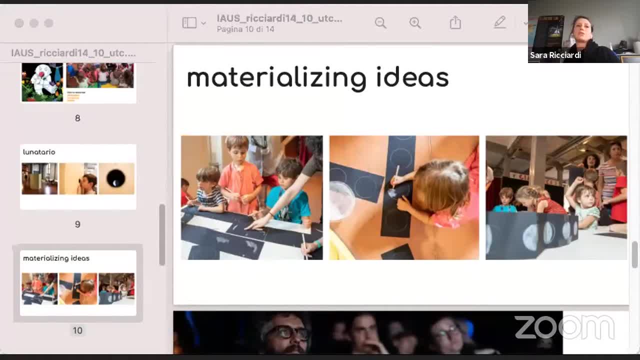 Okay, The small moon sparkled new curiosity in children that immediately recall episode of moon observation and they expressed the desire to observe the real moon again. Exploration of the Lunatario should be done together with exploration of the sky through, for example, life drawing or drawing a moon journal, And then finally, 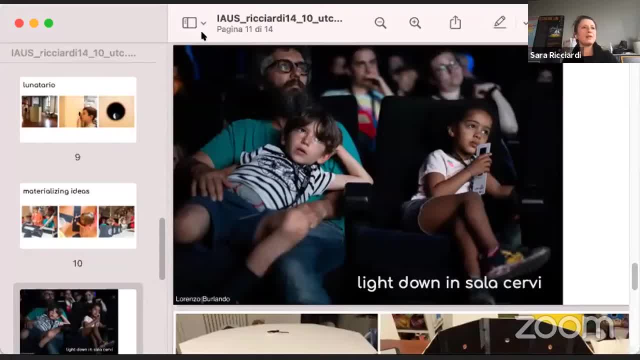 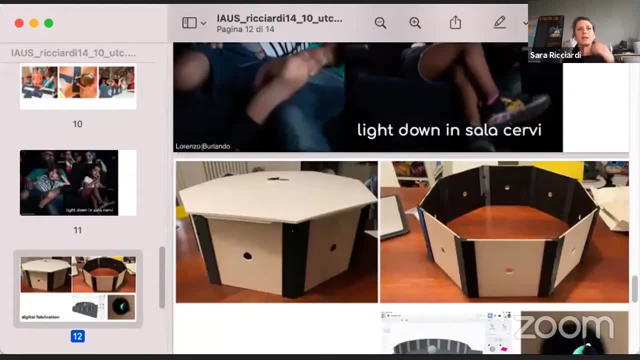 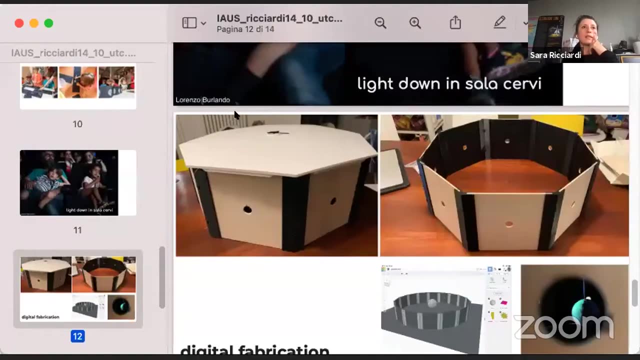 Okay, I don't have time for this one now about the experience in the theater. It's everything I said before about the picture book apply also for this idea, And the 3D printer Lunatario is a good solution to bring this idea in school, because it's portable. 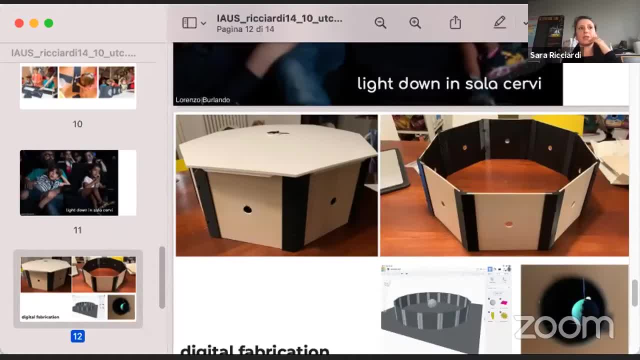 cheap and kids can make by themselves. They can explore with touch. They can explore different geometries. You can do the same with cardboard or light wood. And we chose 3D printing because in Italy, and particularly in our local community, we have a bunch of school equipped with this 3D printer And the variety of teacher training. 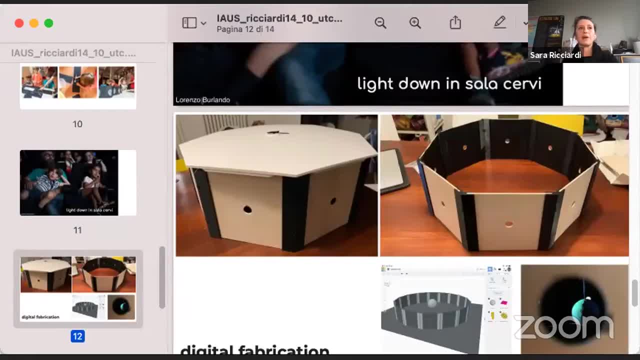 is currently available, where the technical information of 3D printer is provided, but less resources and training is provided instead to illustrate the pedagogical possibility of 3D printing. So opening up this new technology could serve to construct knowledge and own it. 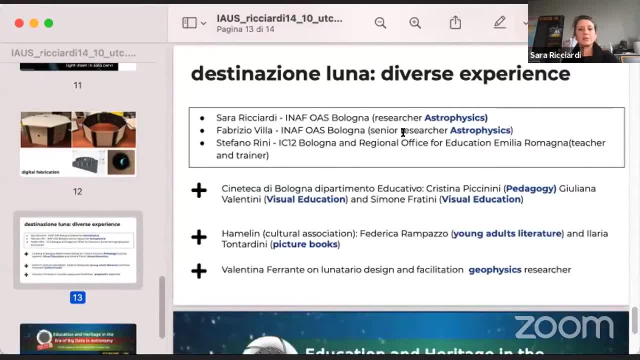 So this is a slide with all the people involved, also because I think it's very important to highlight the different expertise, not just astrophysics, but we got a lot of teachers helping us and also people that are in visual education and young adults literature and picture. 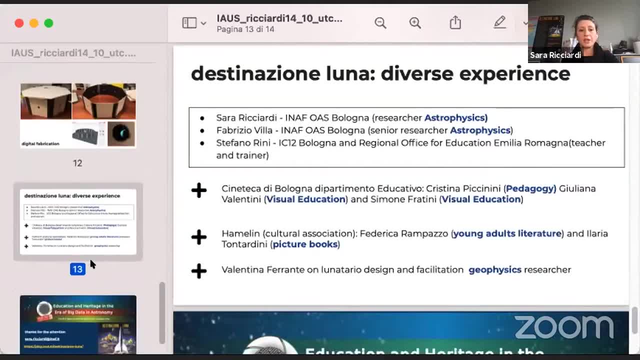 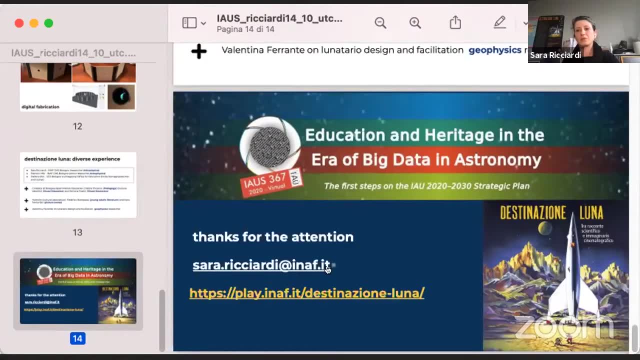 books and pedagogy, And actually I think this is very important. And then again my email, in case you want to have an update or you want to, Okay, Okay, If you need more information, and the website where you can find everything from the print. 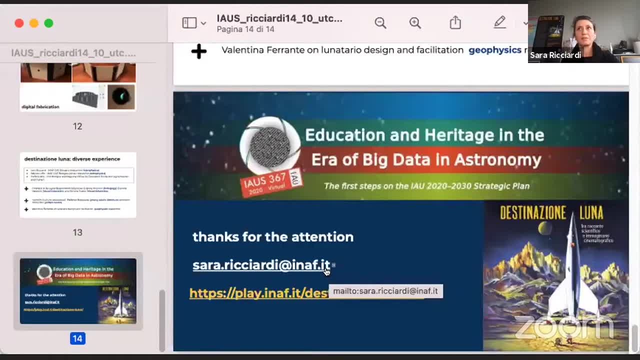 file to all the documentation of the project. Thank you very much, Sarah Bang on time. Okay, So now our next speaker is supposed to be Basilio Solis Castillo. I don't see Basilio. Oh no, Hasn't shown up. 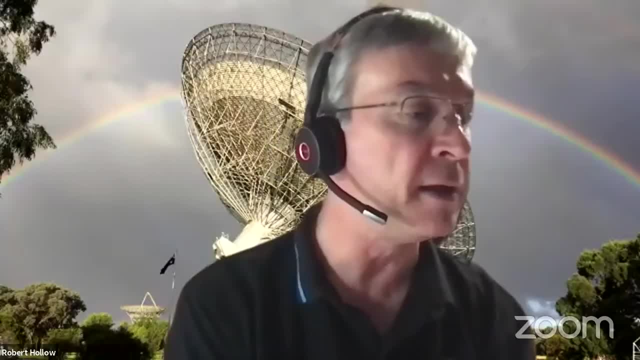 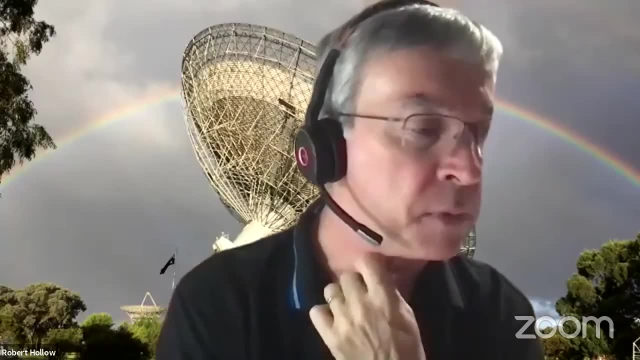 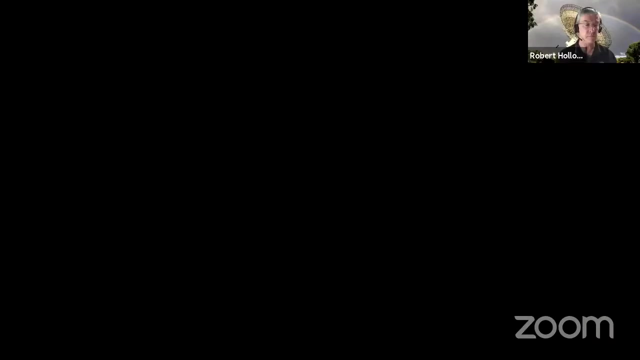 He's not here, so go Right, So we will move straight on To out to our speaker. fourth speaker then, Gary Hemming, from the European Gravitational Observatory. So over to you, Gary. Thanks very much. just show my screen, Can you see that okay? 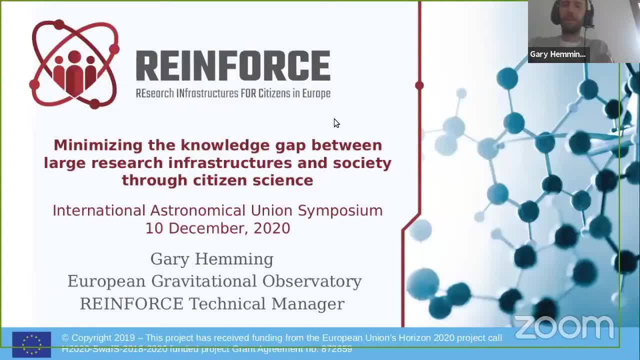 Yes, we can. Great Okay, so nice to be speaking to you all here today. I'm a British-Italian software developer. European Gravitational Observatory, correct? I am Great Okay, So great to be talking to you two at a VERY fast pace And, yeah, I do have an honours. 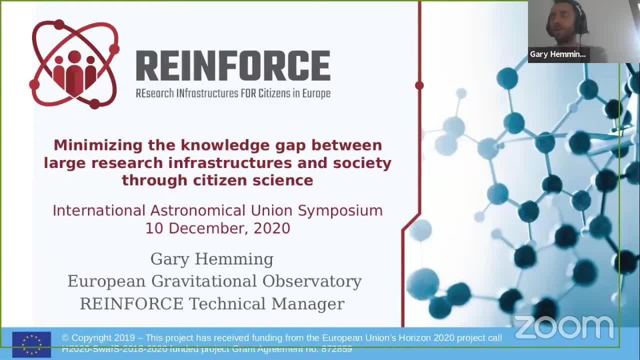 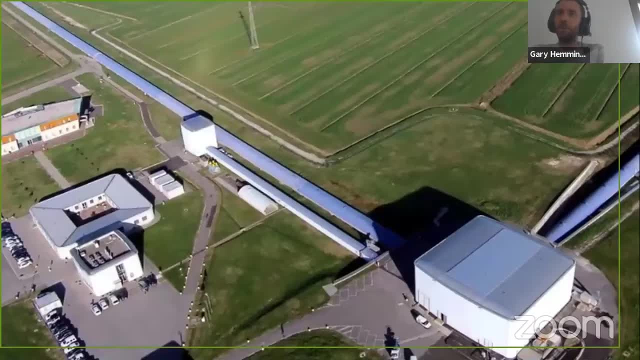 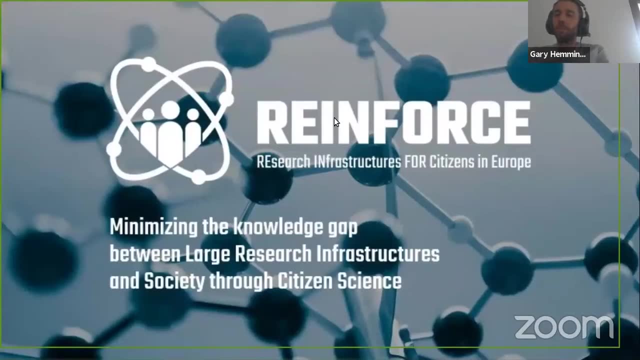 and a member of the Virgo Collaboration, and I'm also the technical manager there's. there's Virgo at the, at the observatory in all its glory, and I'm also the technical manager of the Reinforce project, of which I'm going to to talk to you today. So what is Reinforce, Basically? 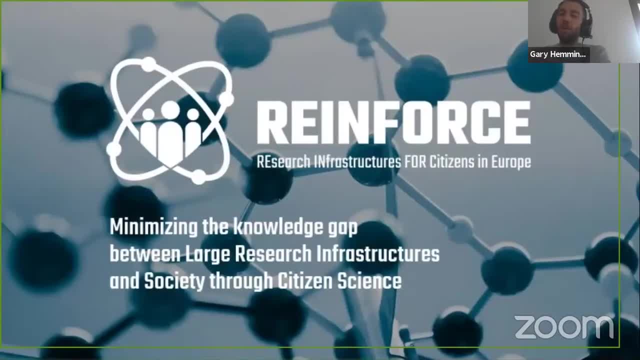 it's a project that receives funding from the European Union within the Horizon 2020 framework, under the auspices of the auspices of the the science with and for society program, and it's been designed with the intention of of bringing large-scale research infrastructures and society. 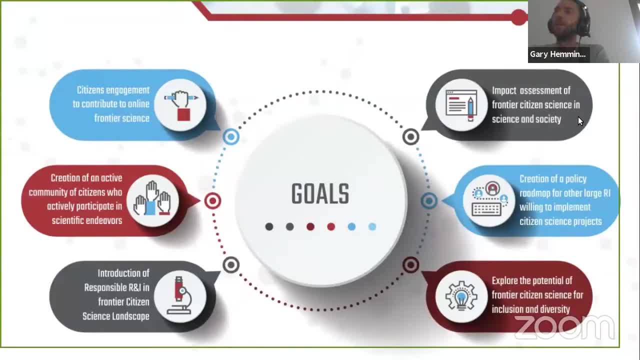 closer through the means of citizen science. It has these, these goals, quite a broad set of goals. with the, it aims to build a community of practice. to undertake an impact assessment of the of the whole citizen science online procedure. to to develop a policy roadmap for for research infrastructures in the future. 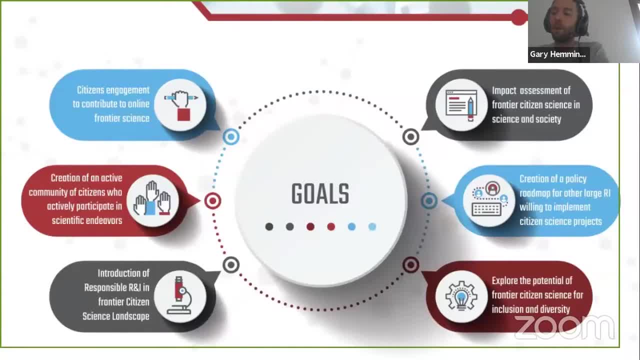 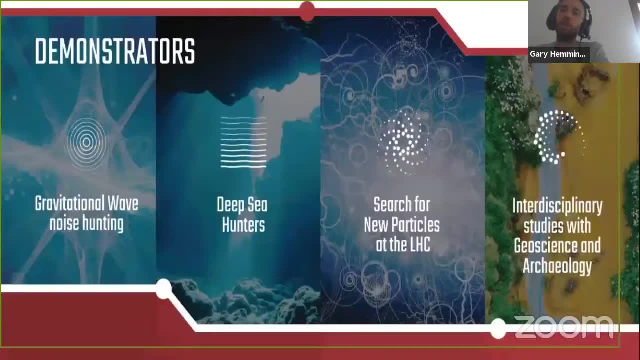 and to do so by concentrating on on on key groups and working in in an interdisciplinary way. Now, uh, the this, this, uh the this goal will be will be reached through uh four demons online demonstrator uh projects, each in a different area of uh of uh frontier science. so we've got. 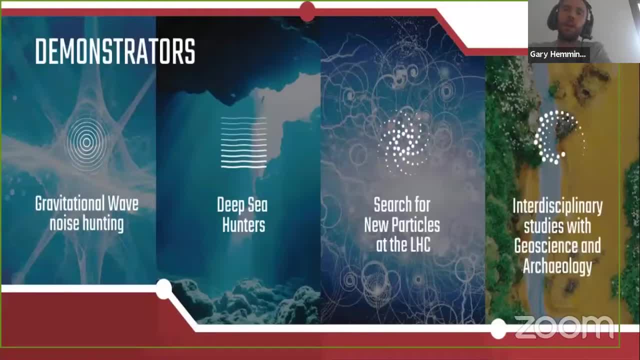 gravitational waves, uh neutrinos where by the, the, the kn3 net uh detector and collaboration search for new particles at the LHC uh, which uses data from the atlas detector, And uh a muography, uh a demonstrator. uh based on uh. the use of uh muography to to understand uh. 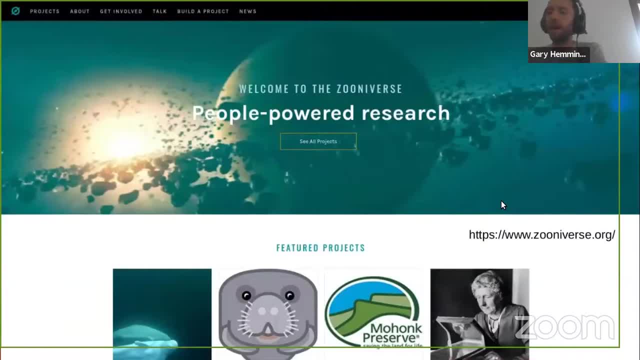 geophysical structures, And we have a big advantage in that we are one of the partners in the project. is is Zooniverse, which which is, of course, a very well-known uh online citizen science platform, and they are, they are embedded directly in in the uh, in in the project itself. Now, um, on top of the Zooniverse, uh we, we have the, the Sono Uno. 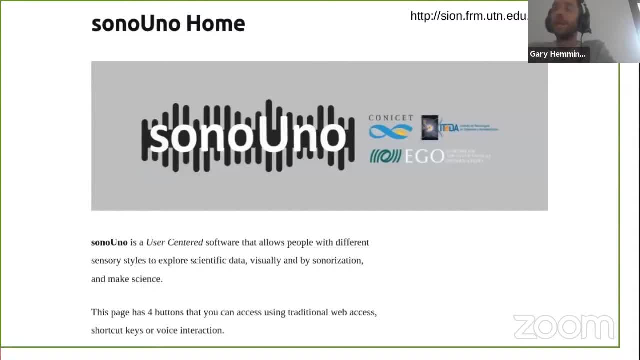 uh team who are led by Beatrice uh there at Koneset and uh they are handling the, the whole uh sonification aspect of the the project be, because one of the the key aims of reinforce is to, to, to make our, our work as widely accessible uh as possible now accessible. 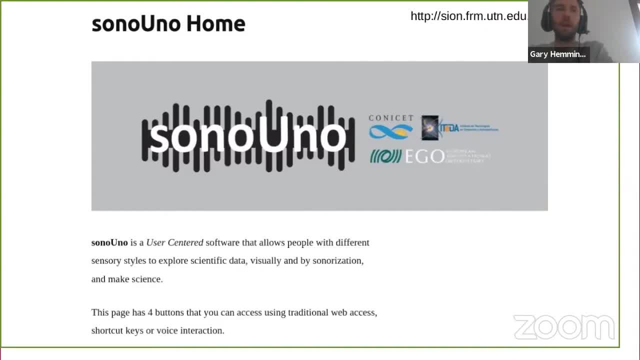 not just in the terms of ticking boxes. let's say so: um, we are, we are looking to, to, to, to make what we, we, uh, we- provide as accessible as possible, because we believe that that is the most effective way of us being able to reach our, our project goal. So 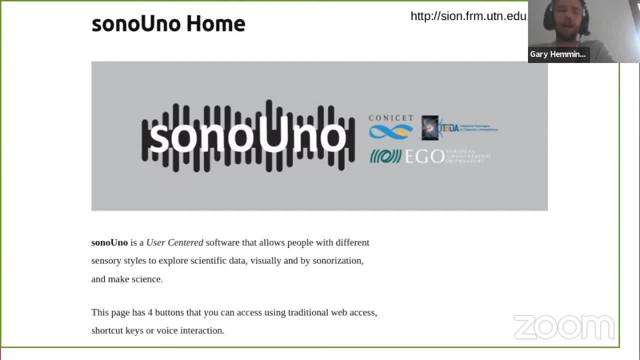 accessibility, the idea of accessibility as being uh imperative for some, but but uh important for everybody, an improvement for for everybody. so, and one aspect of this is the uh, the fact that all of our information which is going to be provided within the zooniverse platform will be all our- 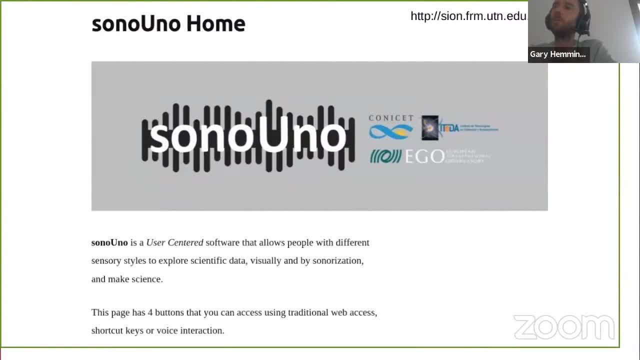 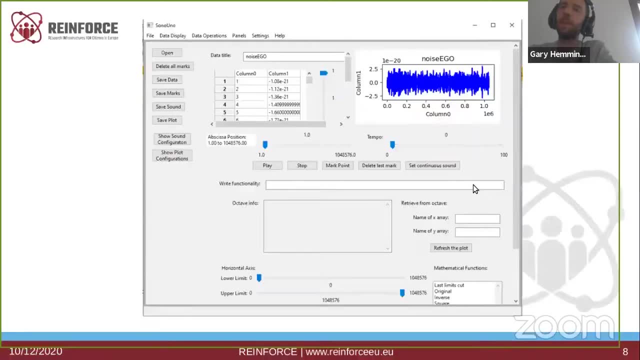 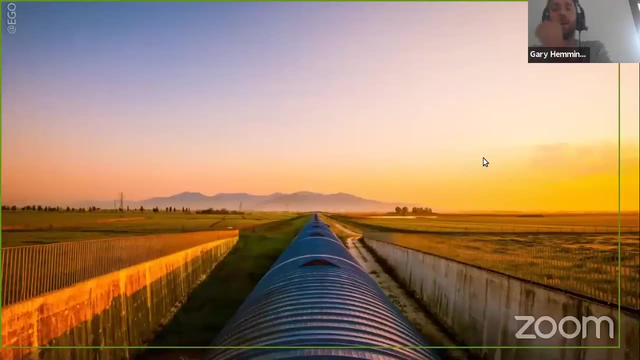 data will be represented in: in in visual formats, but also in uh, in sonified versions, uh via the, the sonowarner software. so there's a quick uh example of the work that beatrice and her team have been have been doing within the project. now, the the individual demonstrators are, we have one. 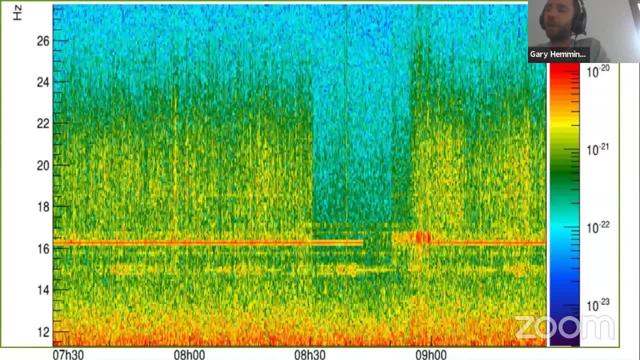 on uh gravitational waves. there you saw virgo uh looking at it to uh on the, the plane of the arno valley near to pisa. and here we see an example of some some of the data that we acquire via our data, uh and uh the. the data that we have is very interesting. you know, we have thousands, tens of 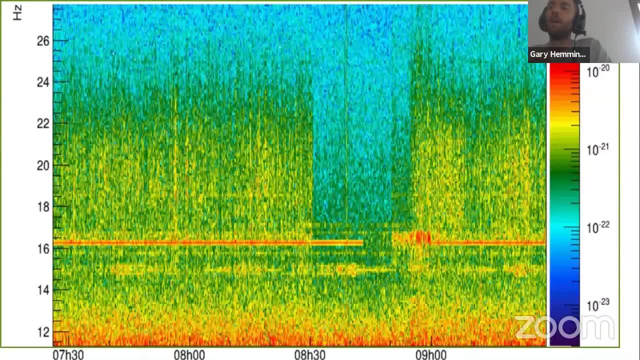 thousands of different channels being acquired at various different sampling rates, and and within within that data, we have a lot of what we term glitches. so, uh, we have to be able to identify these. so what we're going to ask citizen scientists to do is to help us classify the these glitches. 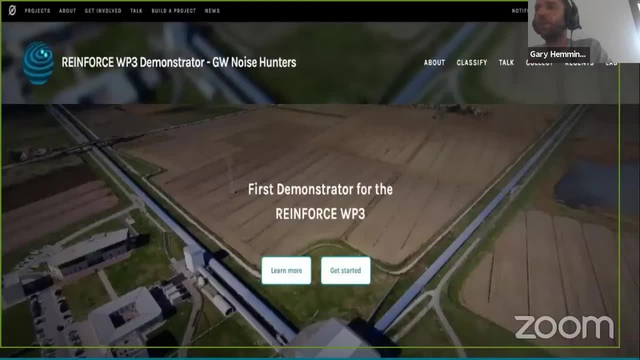 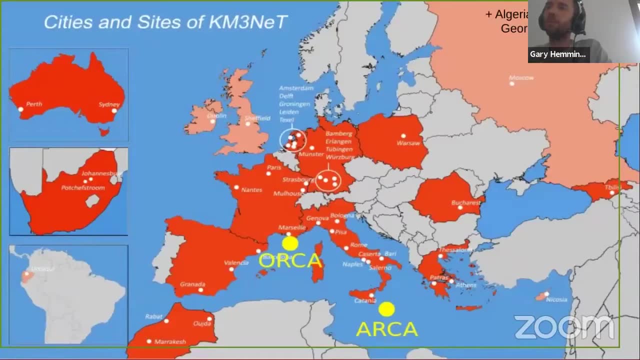 via both uh visual and uh and audio representations of them. uh, beyond the, the first demonstrator we have, as i mentioned in the presentation, uh the the first demonstrator we have, as i mentioned in the before the km3 net team, who are a team of more than 250 uh people based around, mainly around 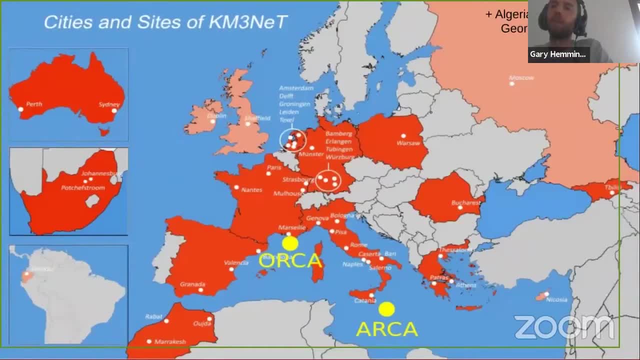 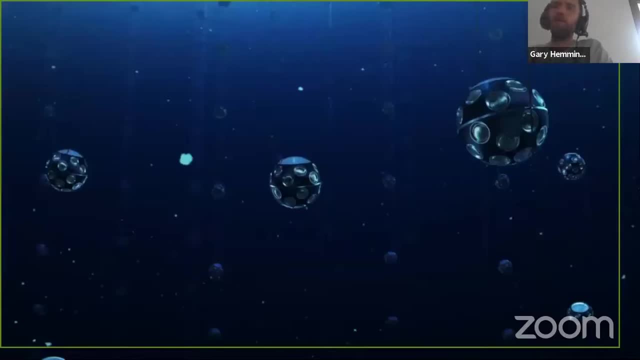 europe, but also elsewhere in the world, uh, with two different detectors, one in french territorial waters, one in italian. and they have these fantastic uh uh neutrino detectors which are dropped to the bottom of the sea and they pick up all manner of bioluminescence, uh and acoustic signals, and 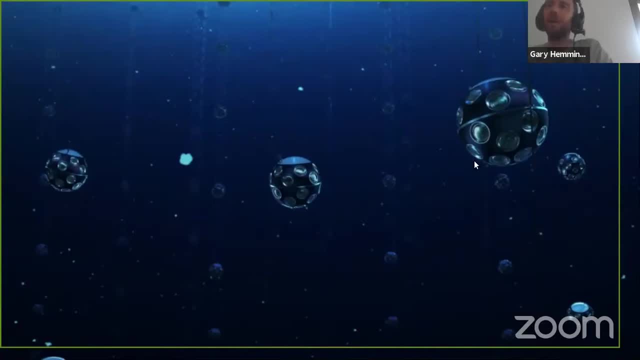 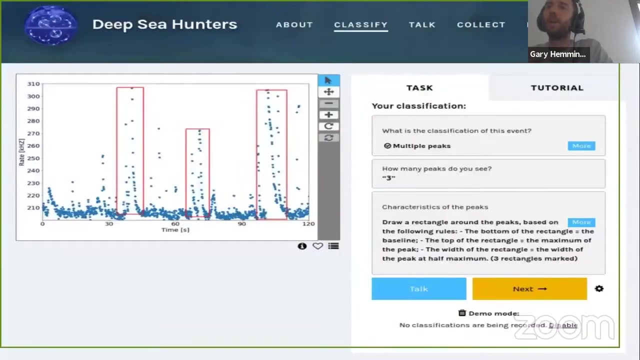 they're quite, they're very uh good. the cam3 net team are very good at uh understanding the uh, the neutrino sources, cosmo, uh, atmospheric and cosmological sources, uh source neutrinos. but they also, by these detectors, pick up uh a vast array of of uh of signals from, from surrounding. 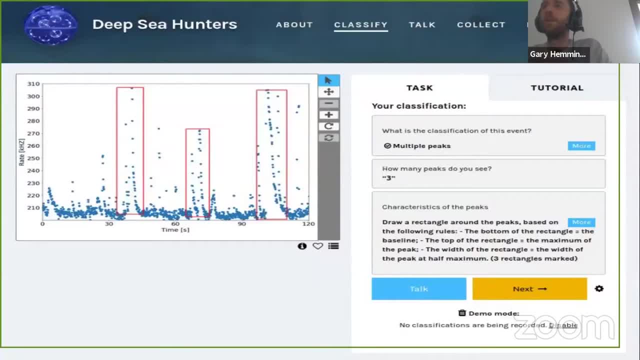 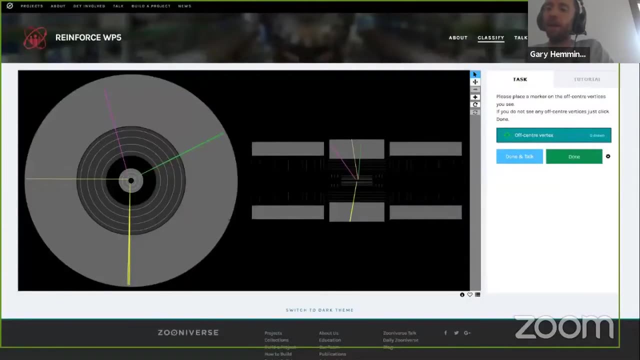 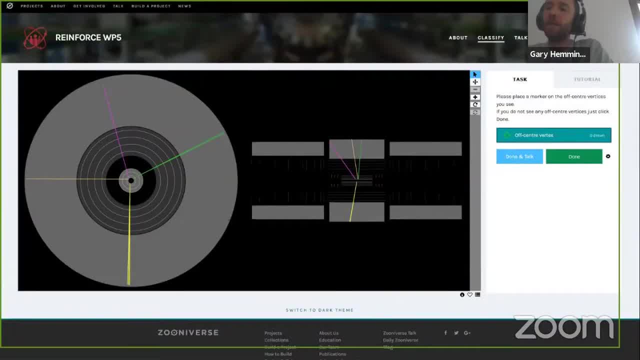 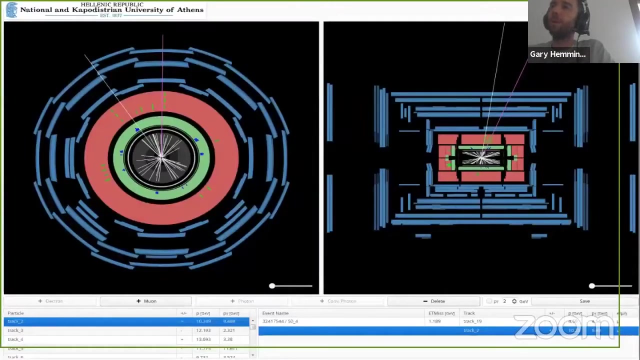 help them to uh, to classify and characterize their, the these, these spurious signals for them. beyond that, we have the, the team at uh, the institute for uh accelerating systems in in greece, and they are, they are using and scientists into the particle identification process. beyond that, we we also have, they have the. 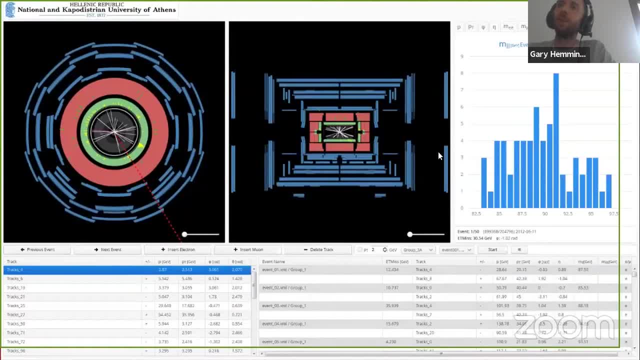 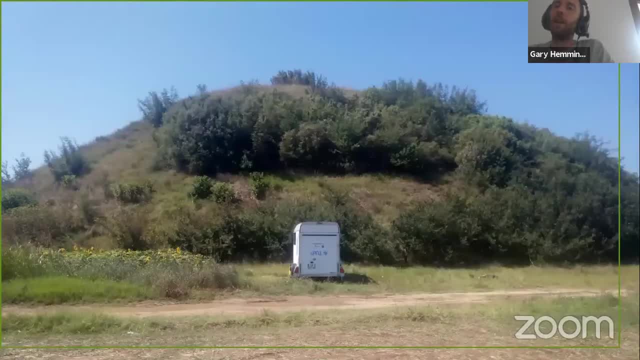 sorry, the three separate stages of the, of the, their procedure, and beyond that we have the muography work package. here you can see a, the, the diaphan diaphane detector, located at a tumulus in in greece. that was at the apollonius tumulus in greece, which was 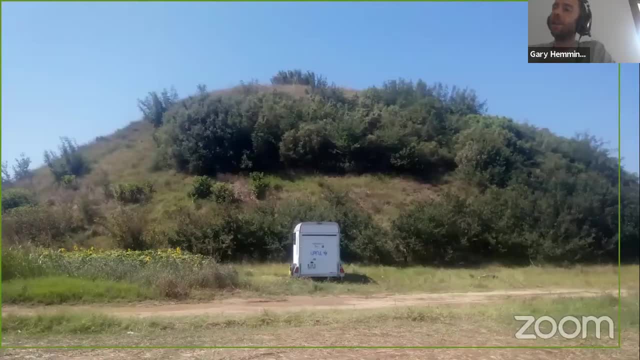 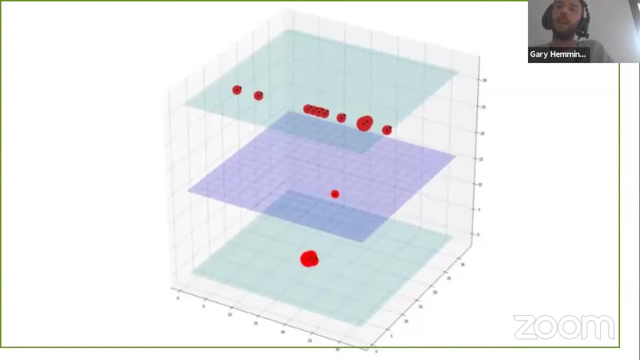 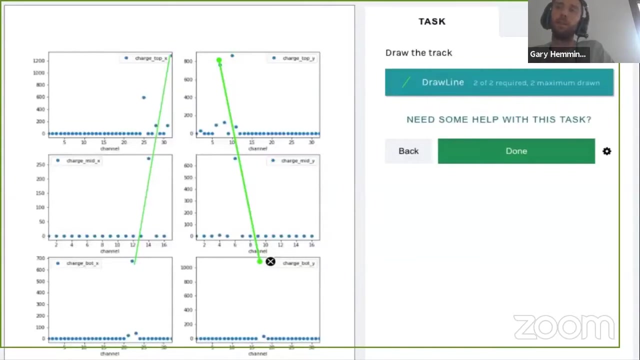 collecting data in 2018 and citizen scientists within this. this demonstrator will be able to to train, first of all, in understanding how how nuance passed through the detector on three across three different dimensions, before moving on to be able to help you to identify uh new patterns and to help to characterize the, the data uh that these uh. 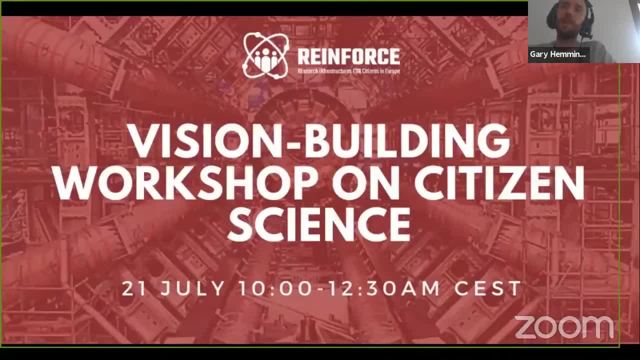 that this team has been collecting over the years. uh, underlying everything, we have a. we're building the project on the principle of participatory design and this is being uh pursued by uh, an organization in greece, ea eleno and germaniki agogi, who are involved in a series of workshops. 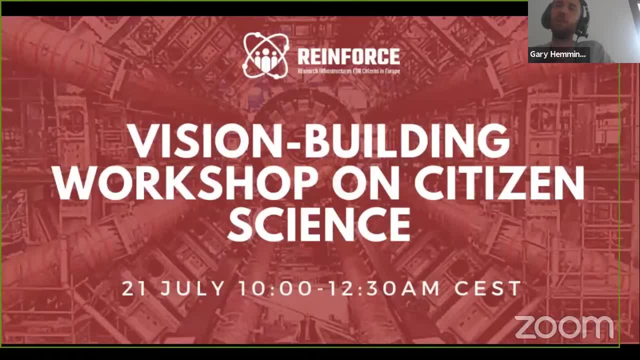 within which these so-called visionary workshops, within which uh um, uh people are able to contribute to, to help to, to shape the development of the project uh and and and its uh general design. two minutes scary, thanks. beyond that, we have a series of uh dissemination activities which 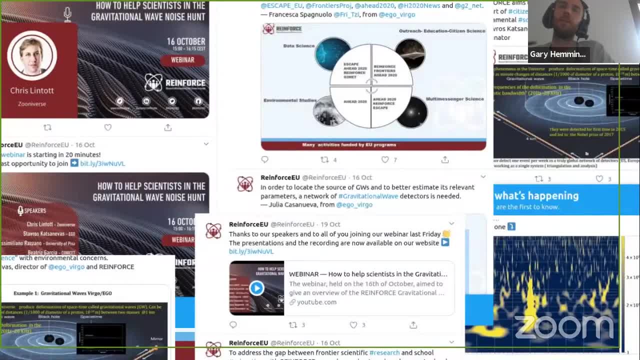 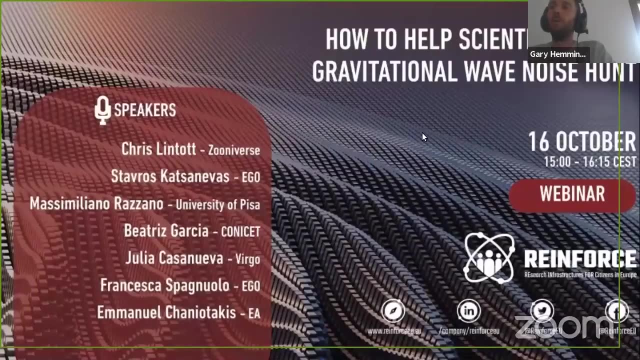 are managed by another partner, trust it, and they're developing a lot of webinars and uh premieres, publicity campaigns and so on. um, there you just see a few examples of some of the things that we've been doing. they've put together a very nice website. we've organized, as i mentioned before. 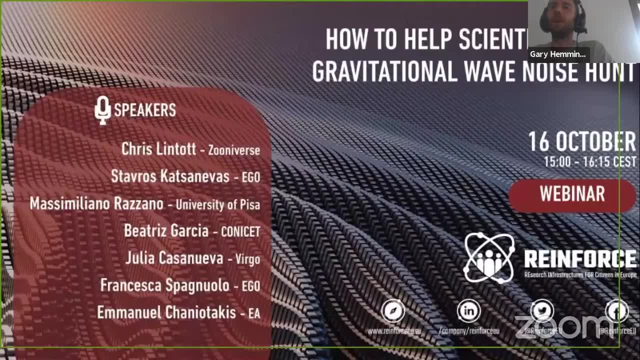 webinars based on building on an episode of the sky at night in which some of the project partners were involved- beatrice's work and uh, wanda diaz-merced, who's also uh in the project as well, uh, and so we've built webinars trying to to dedicate it to to these kind of topics to grow. 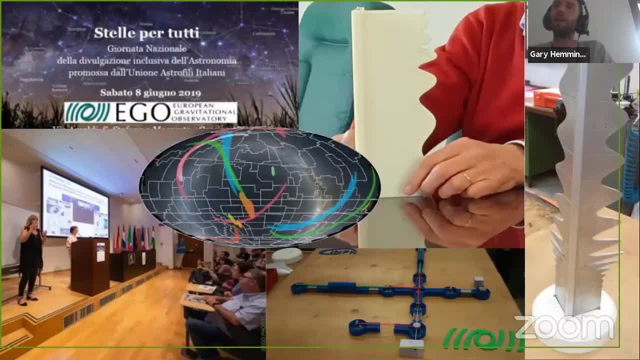 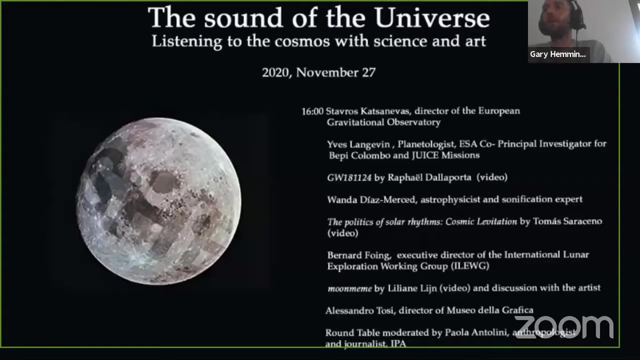 what we're doing. we've got a lot of experience within uh, the, the reinforced collaboration, of making uh, of putting uh together, uh so-called accessible events and making already what we produce uh accessible and we also uh there's a. there's a strong theme of the, of the involvement. 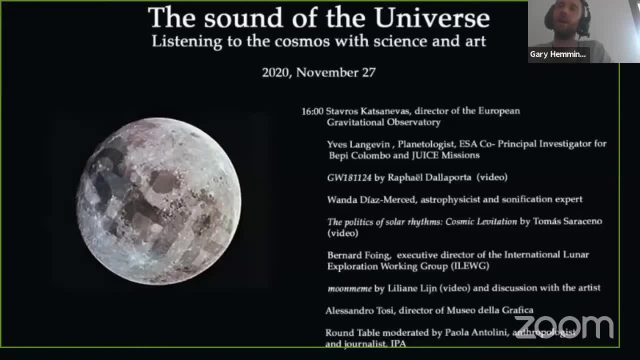 of of the arts in what we're doing? uh. just a couple of weeks ago, we had a uh, a workshop dedicated within the under the, the heading of the european researchers night. uh organized by by ego uh dedicated to this: listening to the cosmos with science and art. so, all to do with the uh, with the sonification of 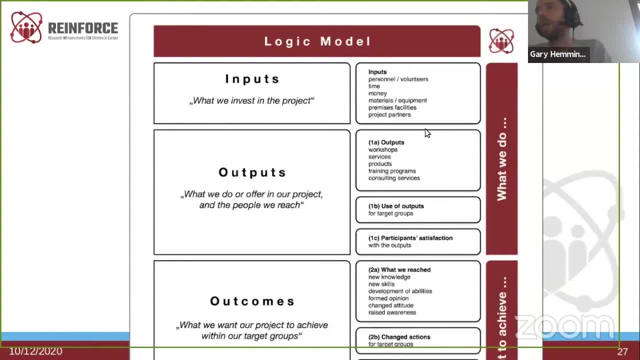 data. well, we have a a very uh complex evaluation model as well, which is being carried on by uh, carried forward by a team in vienna in austria, uh zsi, uh, and so hopefully, uh as we, as we move forward over the coming months. we aim to have these demonstrators on online by the middle of. 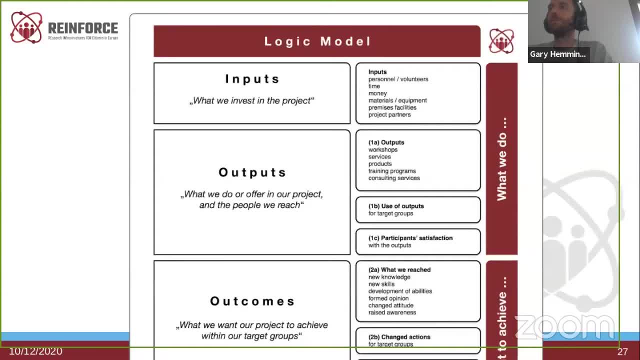 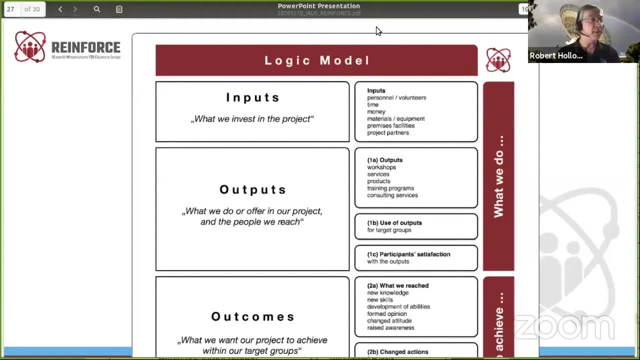 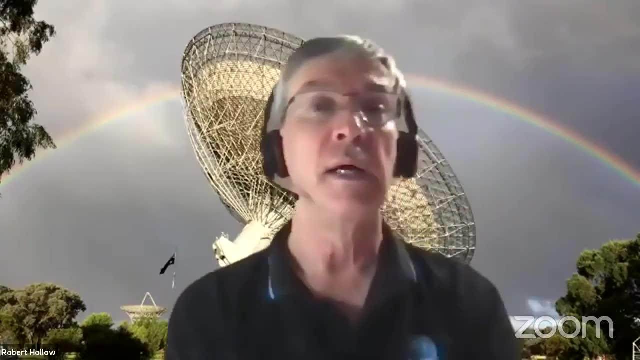 the year and be really be able to look to to produce some results. great thanks very much, gary. right on time. um, so pleased to say. uh, our previous speaker has managed to get online. so, basilio solis castillo. so, basilio, if you'd like to share your screen, and you've got 10 minutes and i'll give you. 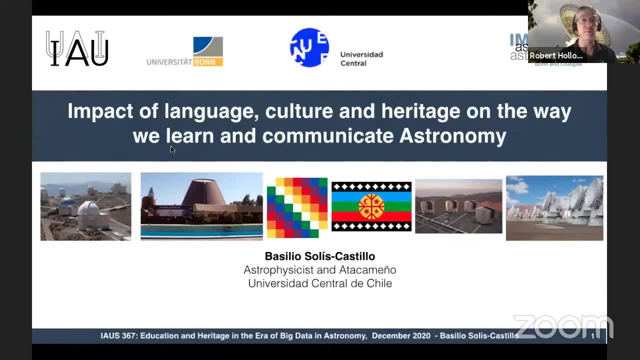 a warning at eight minutes. so thanks, um, thank you. thank you for the the opportunity to to being here and to talk about, uh, something that i consider i i find really, really important. so my name is basilio, i'm from chile and i will talk about the impact of language, culture and heritage on the way we learn and communicate. 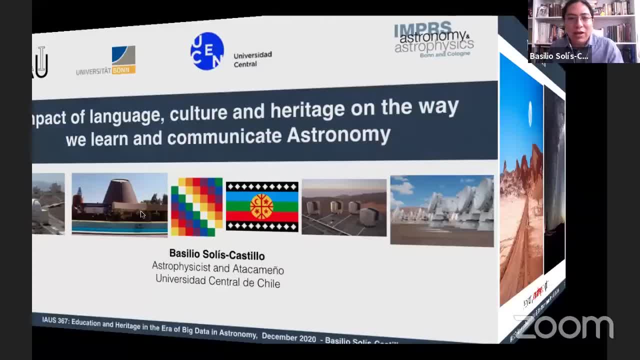 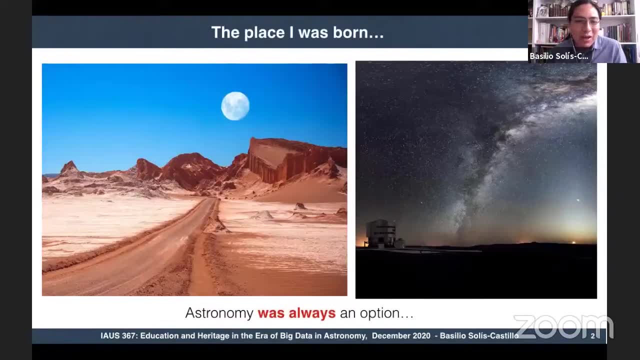 astronomy. um, first of all, as a, as a chilean, uh sorry, as a chilean. i i was born in a place, uh, very, very interesting to learn about astronomy. so for me, astronomy was always an option to to study or to to make my future career studying astronomy. but the thing is from chile. during those 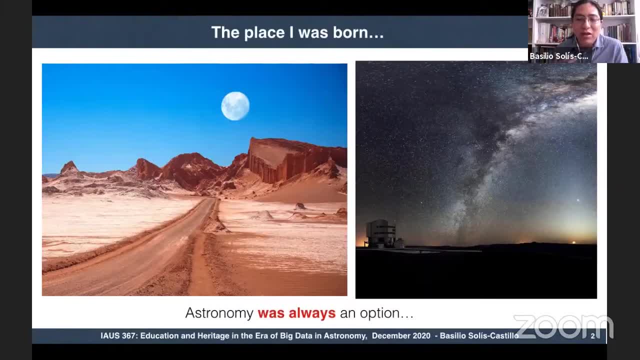 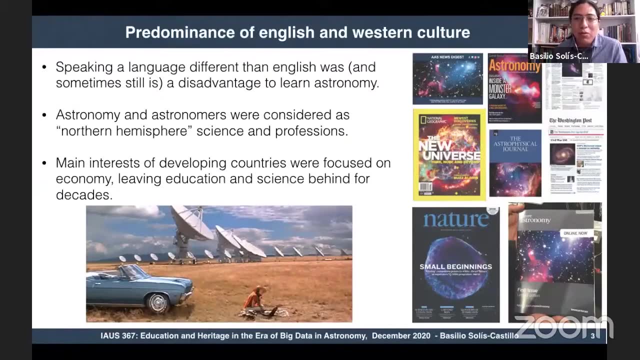 those days was a bit difficult to understand, like what was to study astronomy, like as a career. so normally in the, in the environment, in the world we live in, normally there is a predominance of english and the western culture in in very different things. for example, speaking a language that is different than from english was and 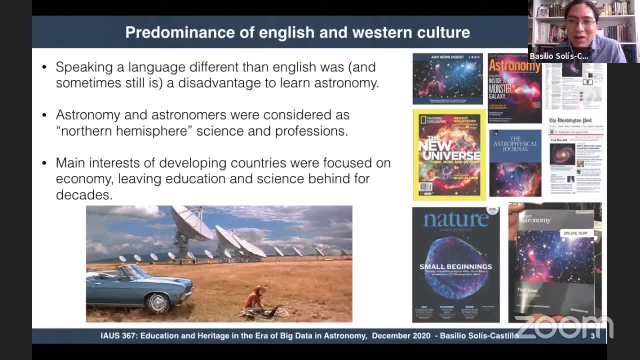 sometimes still is a disadvantage to learn astronomy, because most of the material, most of the textbooks are the most important ones- are in english and of course, the, the, the publications, so the papers we read, normally for doing research, also they are in english. so, speaking a non-english 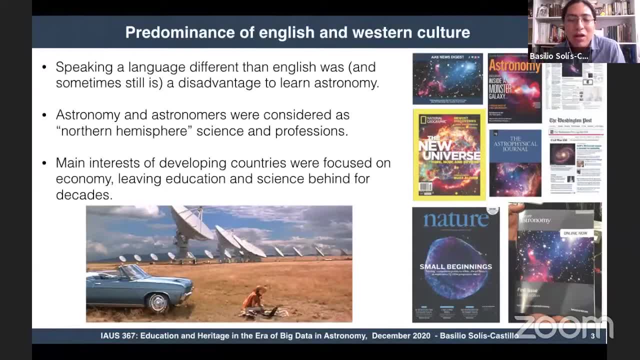 language always affects, in this case to learn like something like astronomy. and in chile a couple of decades, decades ago, astronomy and astronomers were considered something like another hemisphere science or profession. so what was kind of a rear to very strange to find on the street the possibility of having the the to to talk with an astronomer. uh, during those days and and as 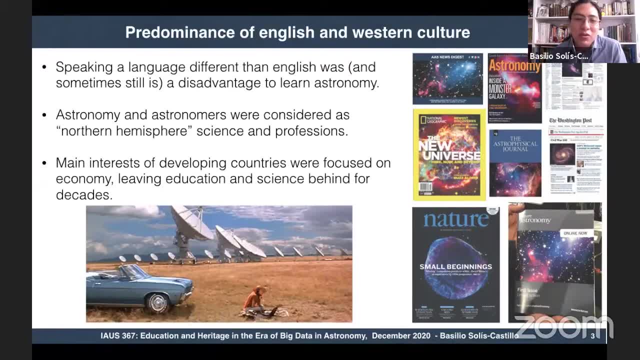 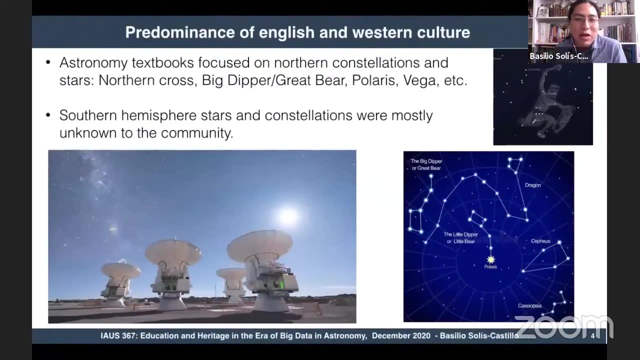 a developing country. of course, the main interest interests of those countries are always focus on economy and leaving education and science behind for for a long time ago. so that was one, one of the things, and other it was like i was talking about the textbooks, so there was a lot of science. 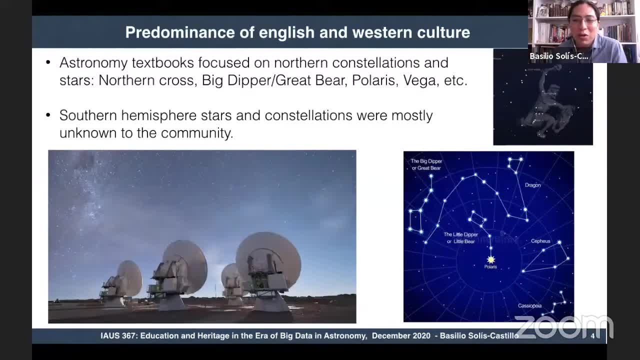 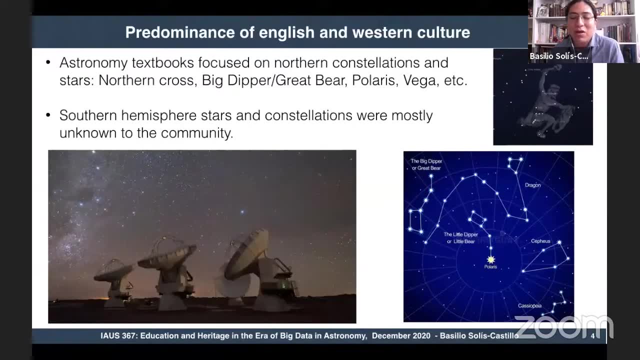 about the textbooks. So when I started to study astronomy, it was difficult to find something in Spanish. of course, Most of the things were related to English. Another thing: they were focused on another: constellations and star, For example, the another cross, the Big Dipper. 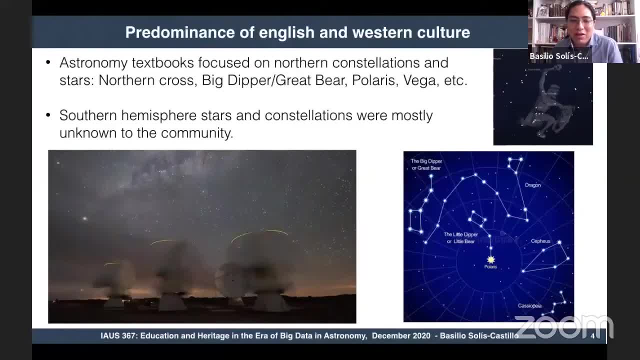 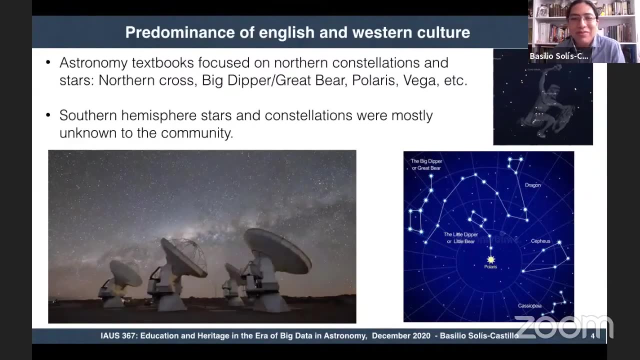 Polaris Vega. So when you find a textbook and later you start to read, you always find this constellation, this star, but they are from the northern hemisphere. So some things like Orion from the southern hemisphere. you can see it upside down, for example. 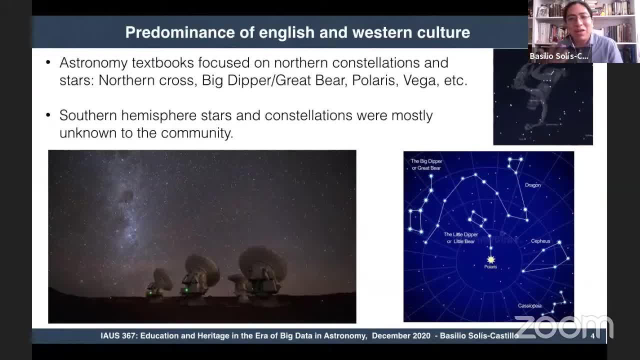 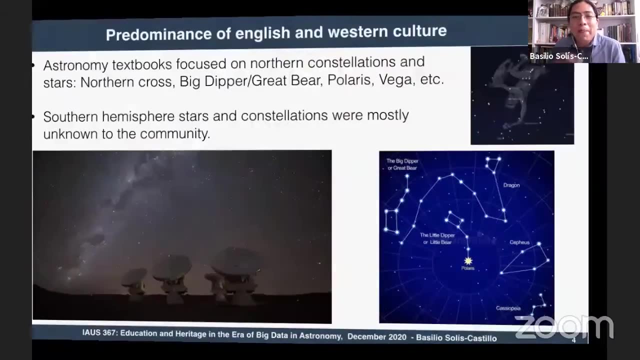 So it was kind of difficult to relate to these things you can find in a textbook And from the southern hemisphere most of the constellation you read on the literature was difficult to find So they were mostly unknown. But during the 60s in Chile 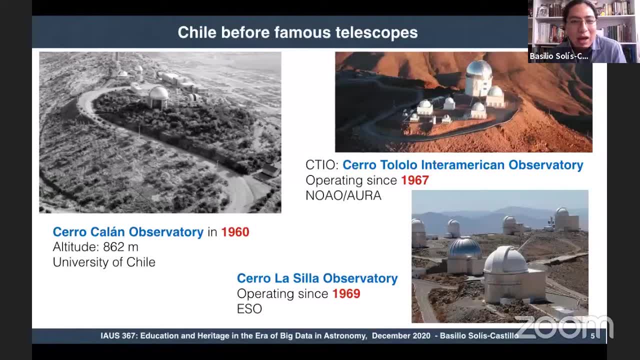 we started to have like a couple of observatories that were installed for the first time. So we started to have, like this change of environment, So we had the possibility to meet a lot of astronomers and starting to get in touch with other people. So there's a lot of different ways that you can get astronomy. 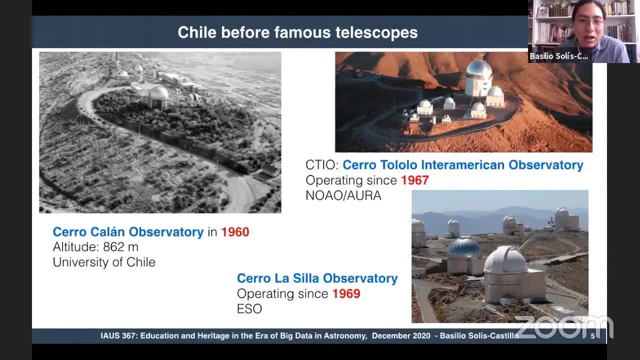 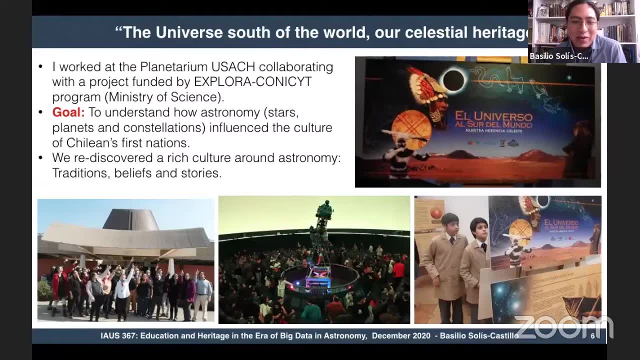 other than just magazines and television programs. So my place in this story, that my contribution is started to work in the planetarium. So when I finished my master I started to work in a planetarium like a mostly outreach institution And getting in touch with people. I find out that 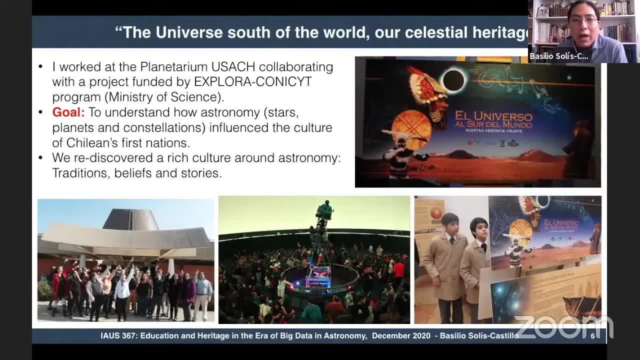 there are other approaches to astronomy and, working in an exhibition called the universe south of the world- our celestial heritage, we started to find out that there are. there are a lot of astronomy knowledge coming not from the western world, was was coming from other regions in this, in this case from the indigenous population, so the Chilean first nations. 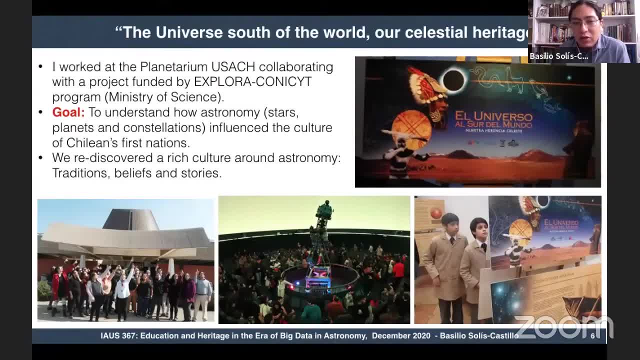 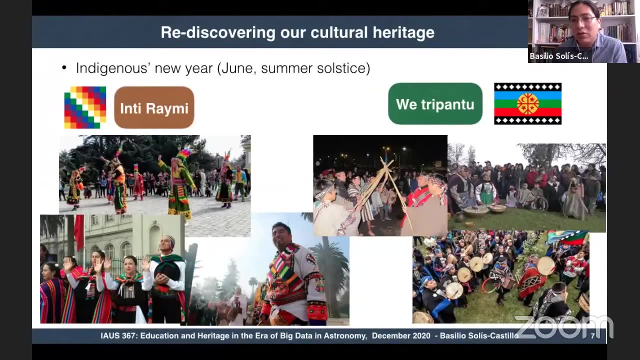 and so we rediscovered like a rich culture around astronomy, so a lot of traditions, beliefs and stories, and this came up like in a time when in Chile is starting to get in touch with a lot of indigenous traditions, so there there was like a growth and in interest of the society to get in. 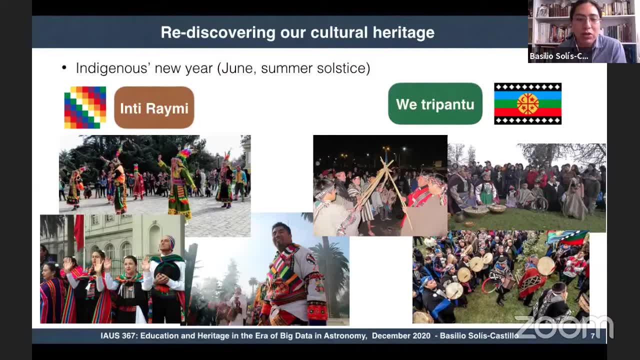 touch with the indigenous traditions and indigenous traditions and indigenous traditions population. so now, for example, the we have, like the new years, the indigenous new year. that is in June, normally, for this this the summer solstice, and we celebrate like the new year nowadays. so that's, that's the way the things have changed in Chile and related in relation with the how we 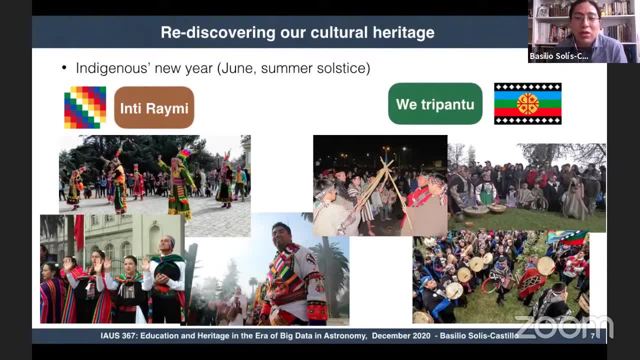 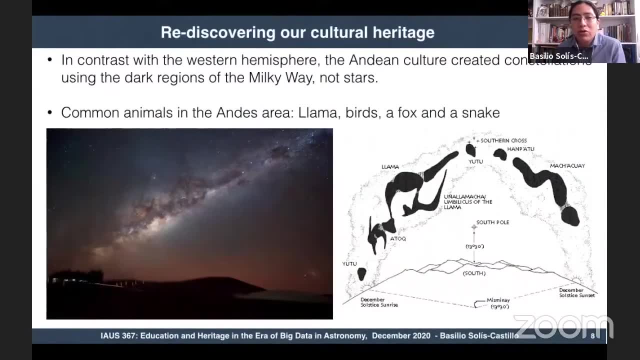 we see our indigenous population and indigenous tradition that now we have. and why I'm talking about that? because in contrast, in contrast with the western hemisphere, the Andean culture. so, from the northern part of Chile, they created, for example, constellation not using star, they were using the 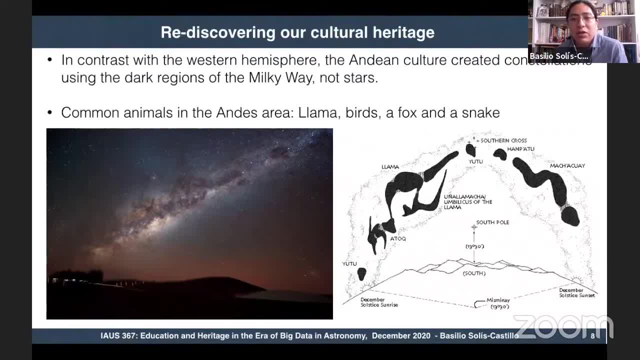 dark region of the Milky Way, for example. so the constellations, the, the, the inhabitants of the Andean region was related to the dark regions. so the, the non-present, the no presence of stars, instead of uniting stars, Like forming, like a figure. and they, these, these people they use like common animals in the Andean. 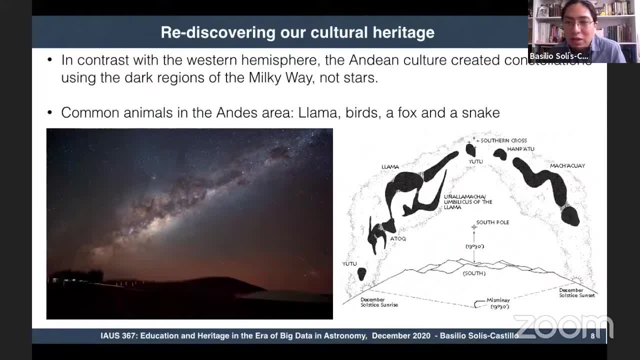 area like llamas, birds, foxes and snake, in order to like um to, to share, to explain the universe they were living in. so they, they started like um, these, these findings. they were like a lot of people really separate toys in order to have that in their history. so then, when likeءing in place'. 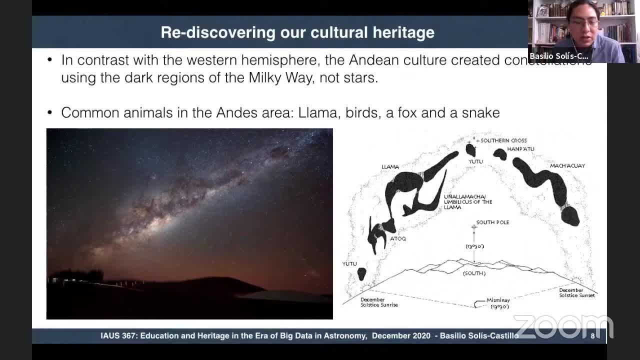 to be able to create them. suddenly they are looking around, thinking won't be necessarily, you know, the first one coming up, or would be like an obsession, because the the character which that to rediscover this ancient, ancient culture. so, for example, we have the jakana, that is. 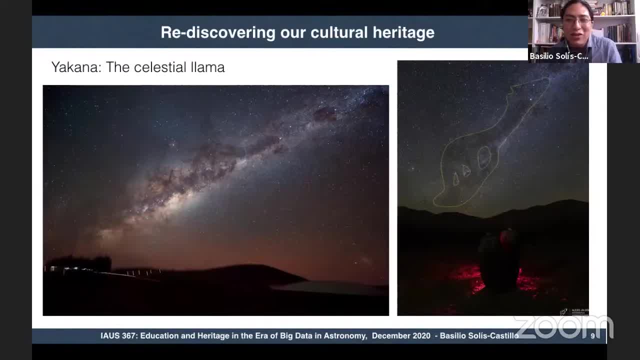 the celestial llama that is in the sky and in on the left side you can see, like the, the, the drawing of this llama. so they use this part of the milky way, the dark regions of the microwave, of the microwave, to depict this celestial llama. so, but also there are the 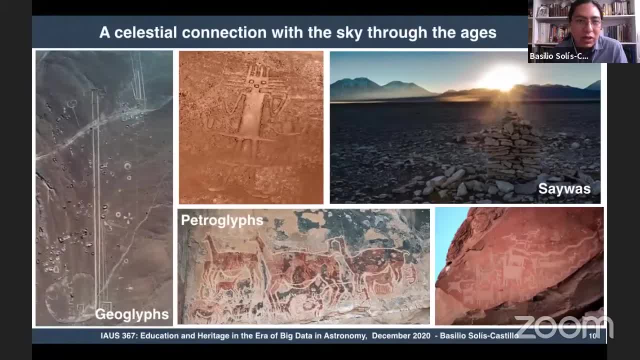 we find out that there is like a very interesting connection with the sky through the ages. so we found some monuments, some some um petroglyphs, so so, or on and geoglyphs on on different parts of the northern part of chile and they were showing the same. so they were. 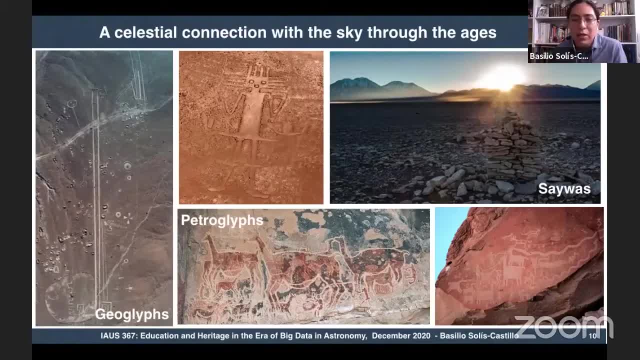 using this, this, the somersault is the um, so they were talking about the like, this is the, the change of seasons, and they use this change of season and this, these alignments, to build their calendar and the petroglyphs and the helioglyphs they they were using to explain what they were. 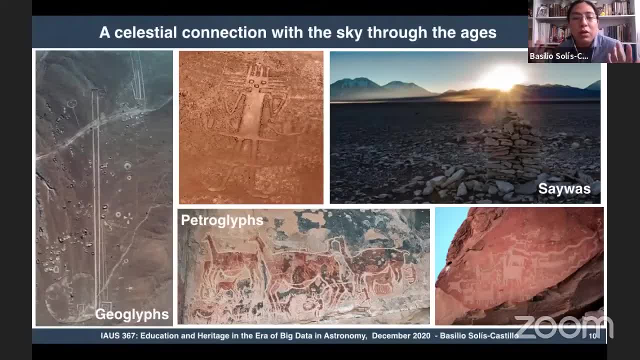 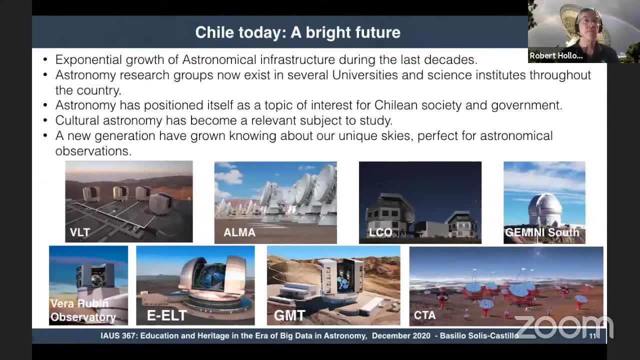 watching in the sky, so they were reproducing what they were. uh, what it was in the sky. and two minutes, thank you. and well, chile today is very different place from like a couple of decades. decades ago, so we had like exponential growth in astronomical infrastructure. during the last decades we have 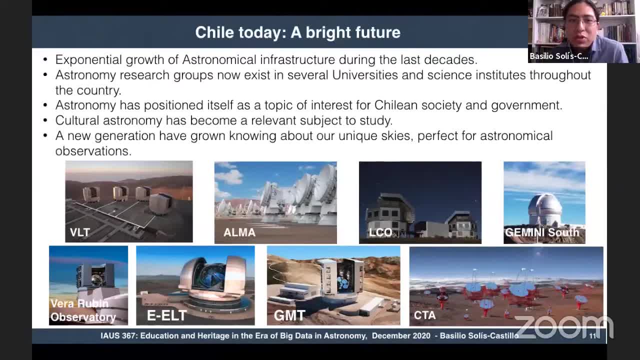 now a lot of astronomy research, research groups like working, several universities, science institutions, and now the astronomy has positions itself as a topic of interest for chilean society and government. now the is talking. uh, it's not. it's not really strange to see one astronomer talking in the television. 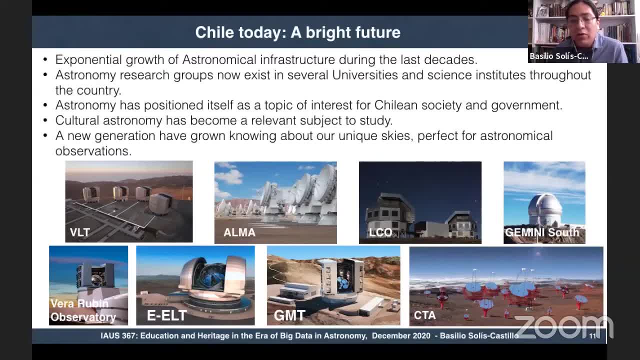 so uh, and now uh, i could say the last decade we had like a very uh- the cultural astronomy. so the the culture around astronomy has become a relevant subject to study and a new generation of chilean have grown, have grown knowing about our unique skies, and that is perfect for astronomical observation. 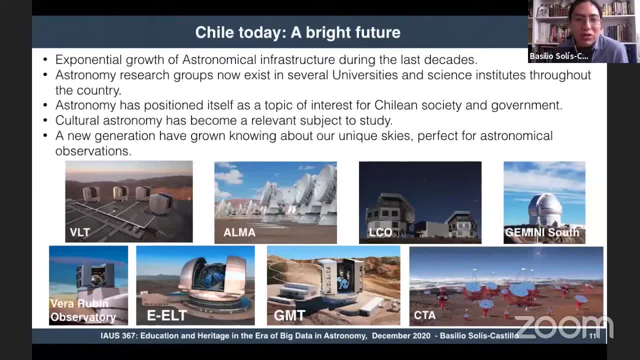 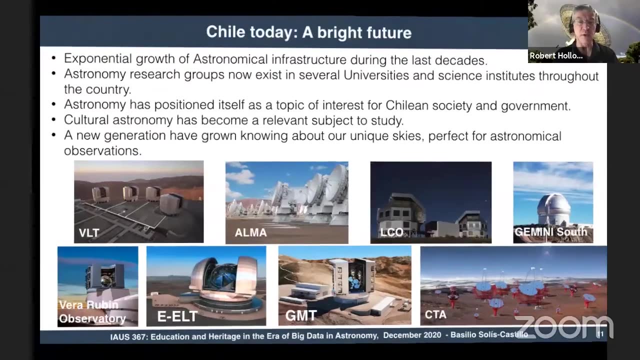 and nowadays, to become an astronomer is not so so strange. strange as as it was like 20 or 30 years ago. thank you for the time great. thank you very much, basilio. uh, and it's great to see um as somebody here in australia. it's nice to see some other southern skies. 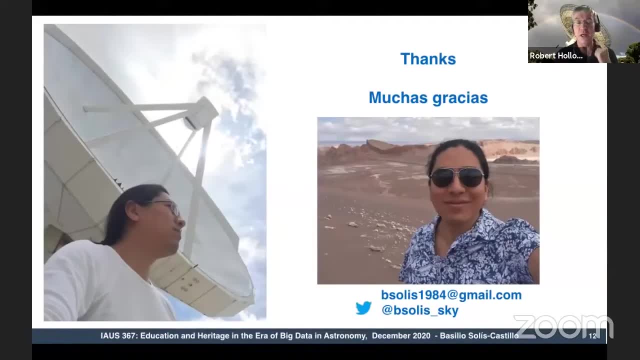 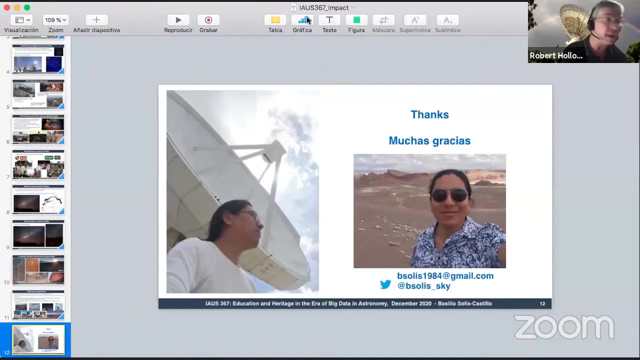 i'll point out that uh, the llama, uh in chile becomes the emu to many of our indigenous uh astronomers here in australia. so our final speaker for this session, uh, will be sutapa chattopadhyay. i'm sorry if i've pronounced that incorrectly, so if you'd like to share your screen, please, yes. 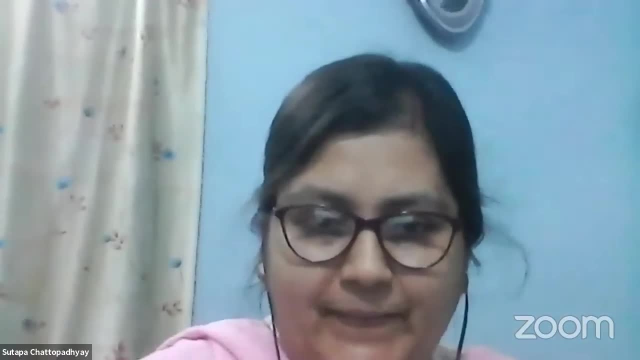 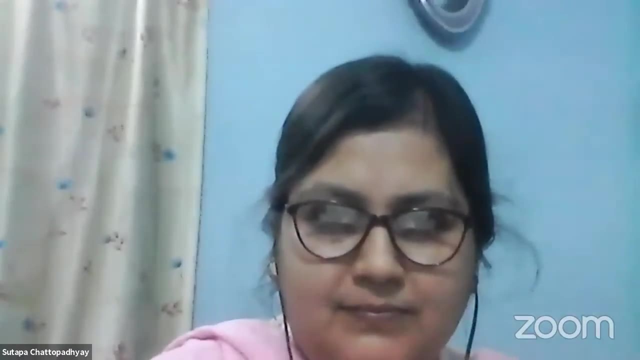 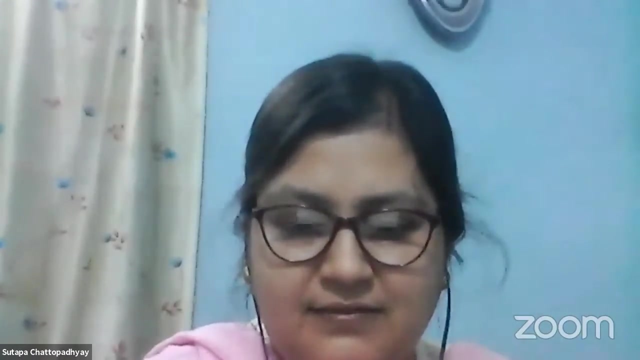 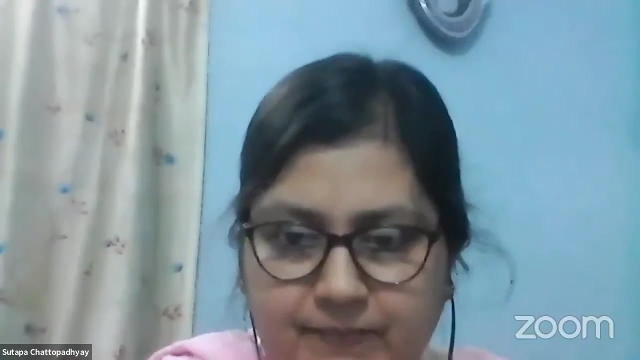 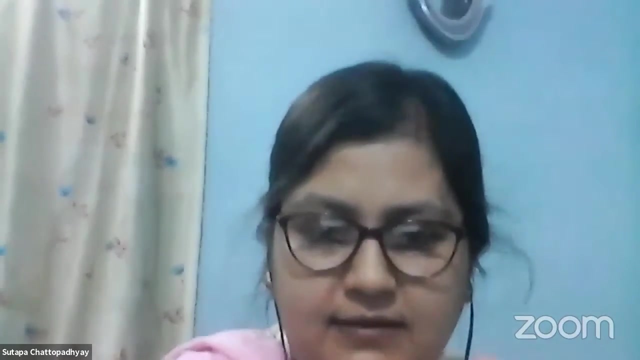 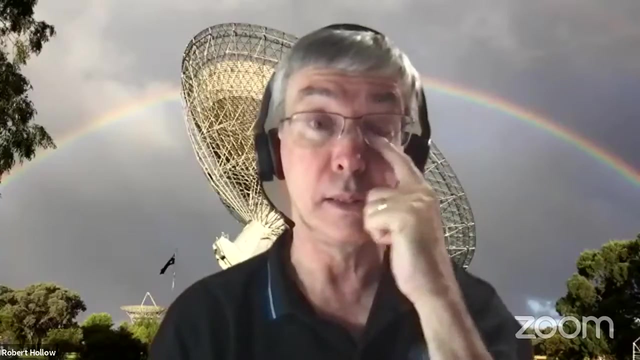 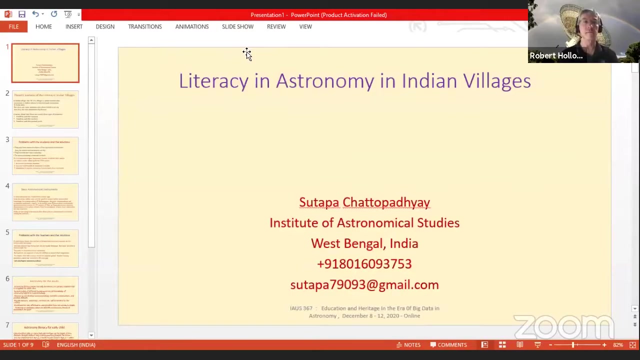 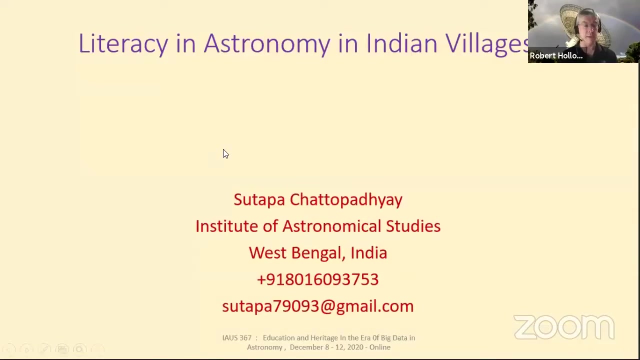 i'm starting in a moment, that's right, okay, can you see my presentation? not yet. let's try again. just a moment. i'm sharing my screen. is it visible now? can't see it. Hang on, something's coming through now. I think now it's visible. Yes, Yeah, Thank you, Yeah, great. 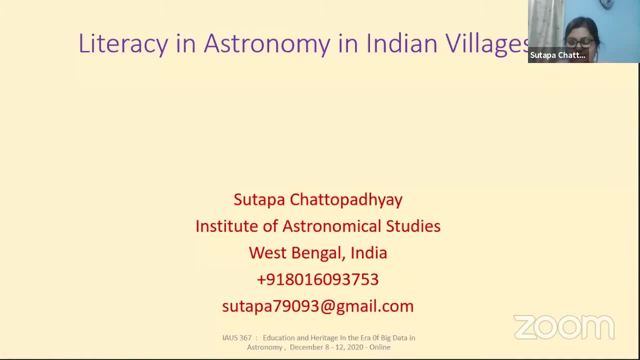 Hello, I am Shrutapa Chattopadhyay. I am from Institute of Astronomical Studies, West Bengal, India. I am a primary school teacher and an amateur astronomer and educator. I'll be talking about literacy in astronomy in Indian villages. Let's introduce our institute in this prestigious 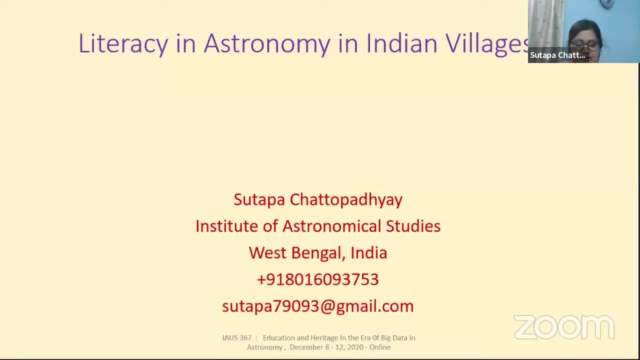 platform of IAU Institute of Astronomical Studies conduct workshops for primary and secondary school students with low-cost or no-cost materials. In their classrooms. students are able to make star trackers, maps and maps of the world. They are also able to make 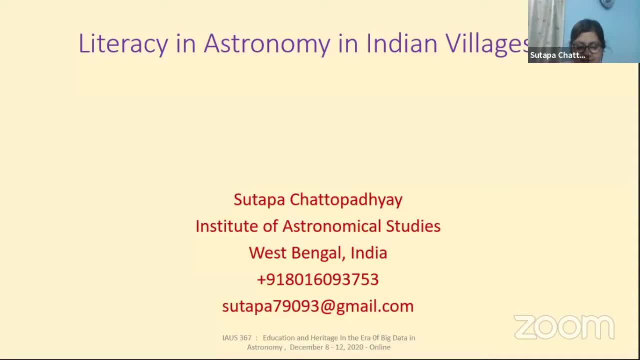 pinhole camera sundial by themselves. In the evening they observe sky with our portable telescope. We have arranged a short course, six-module course to initiate astronomy and motivate them for science and technology careers. For the teachers, we are arranging online. 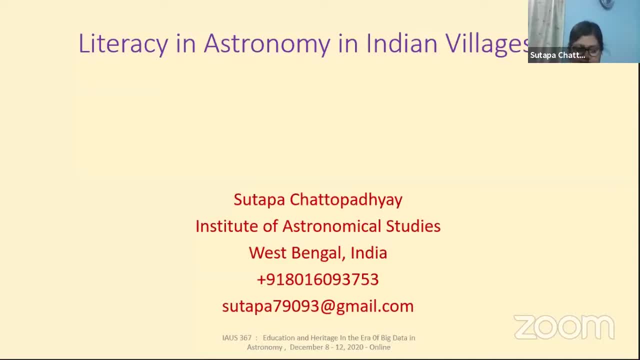 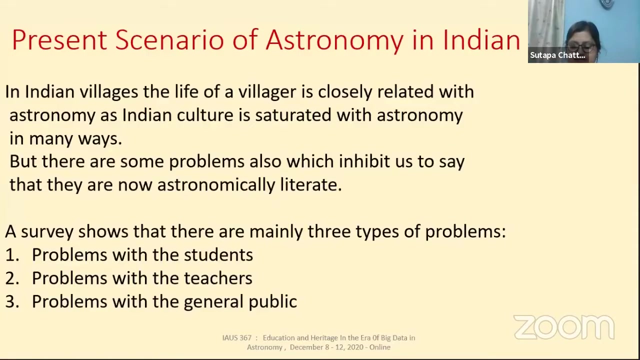 teacher training courses and two workshops in 2021.. The object of this training is to motivate students through them. Thank you. In a pilot project, we select six schools and, till now, we get average response. in this pandemic situation, Let's see the present scenario of astronomy in Indian villages. 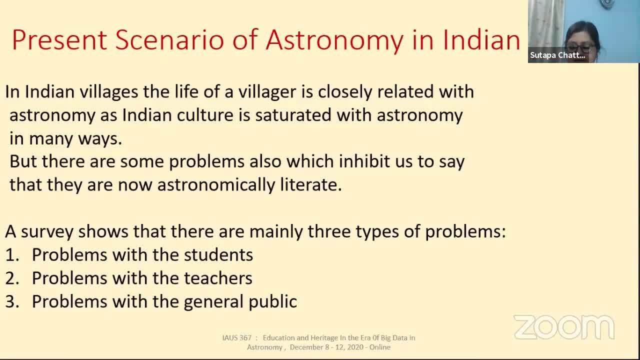 In Indian villages. the life of a village is closely related with astronomy, as Indian culture is saturated with astronomy in many ways. Indians have many occasions, rituals etc. which have come and gone. They have come and gone. They have come and gone, They have. 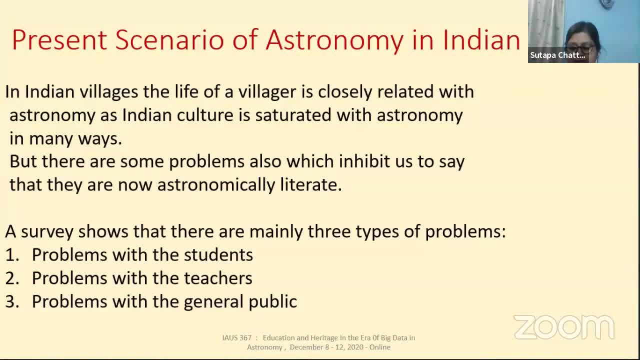 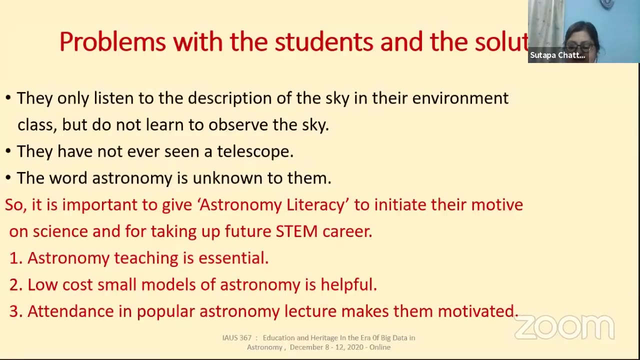 come and gone for the full, observe the sky. The second problem is that they have not ever seen a telescope. and last of all, the word astronomy is unknown to many of them. So to initiate their motive on science and for taking up future stem career, it is important to give astronomy literacy by a class-wise. 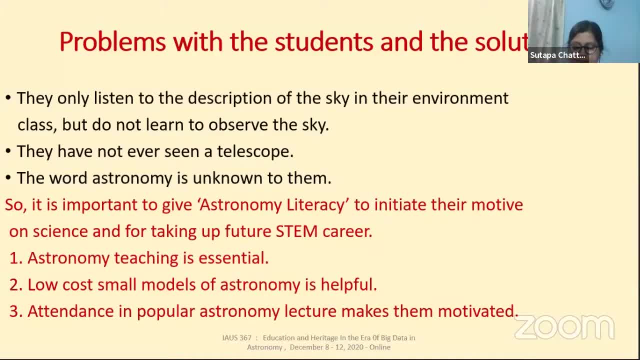 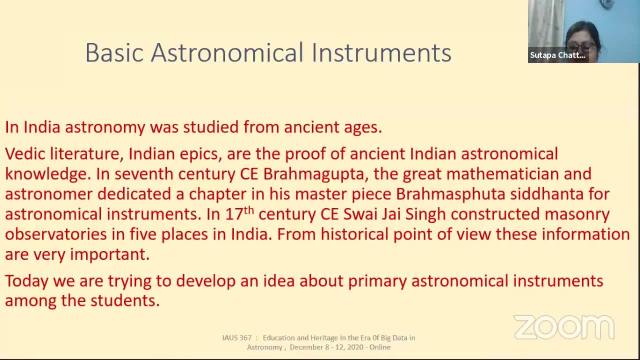 short astronomy course which we are trying To initiate astronomical literacy. they have to know about basic astronomical instruments. In India, astronomy was studied from ancient ages. Vedic literature, Indian epics, are the proof of ancient Indian astronomical knowledge In 7th century CE. 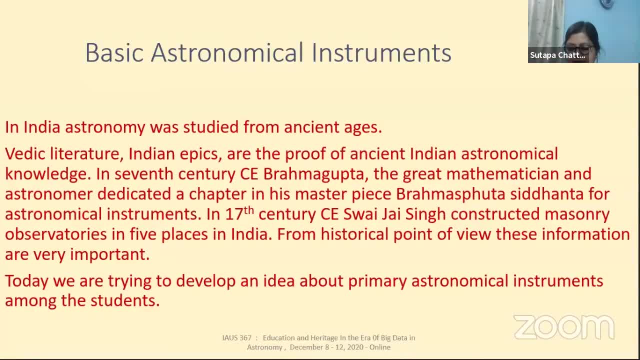 Brahma Gupta, the great mathematician and astronomer, dedicated a chapter in his masterpiece Dambhashputa Siddhanta for astronomical instruments In 17th century CE. while rejoicing constructed mathematics, Motionstruetuses use stationary observatories in five places in India, that-is in Jaipur. 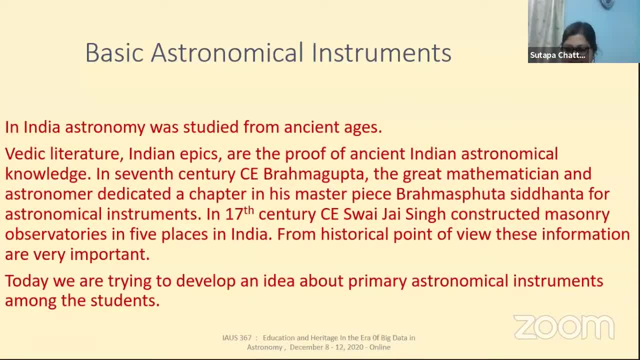 In Varanasi, in Delhi, in Mathura and Ujjain. These overwhelm-observatories play an important role in astronomical literacy. Today we are trying to develop an idea about primary astronomical instruments among students. We have a plan to introduce telescope in schools which are selected as the pilot project. It will be focused on the bombarding science, diamonds, with geosショepers to study the calabash- сторону rush and with a small group of school�the个''žípçonалы'Śğcipister. the Iastri'ţs, With the help of any school subject, did this BIG8. a cruise307 was started. It came from the National Observatory in India, that is, in Jaipur, in Varanasi, in Delhi, in Mathura and in Ujjain. 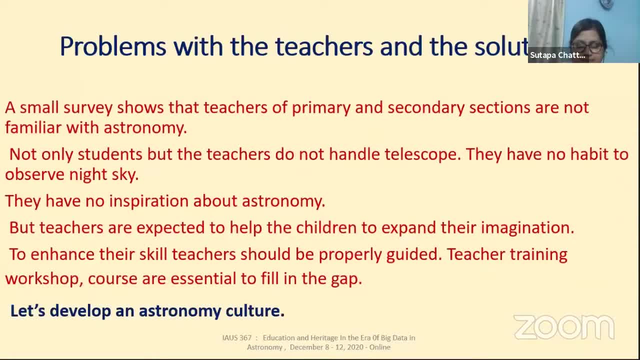 possible if we get sponsors. Now let's come to the problems with the teachers. Most of the teachers of primary and secondary sections are not familiar with astronomy. They do not handle telescope, nor have the habit to observe night sky and have inspiration about astronomy. 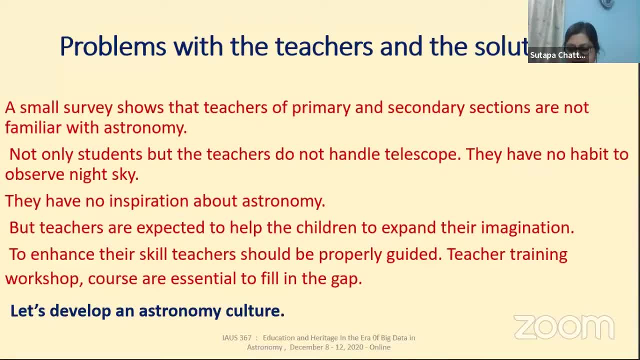 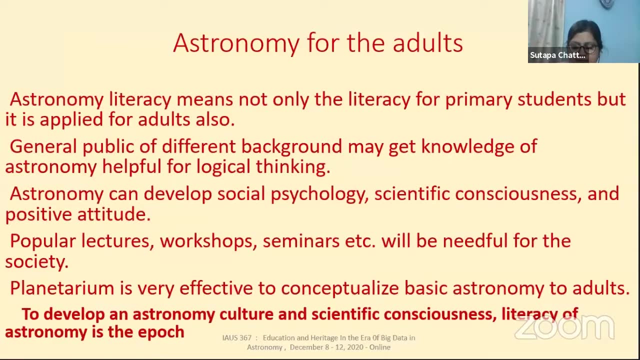 But they are expected to help the children to expand their imagination. So to enhance their skill. they should be guided with teacher training workshops, astronomy courses, etc. Let's develop an astronomy culture. Now let's talk about astronomy for the adults. General people can think logically if they get. 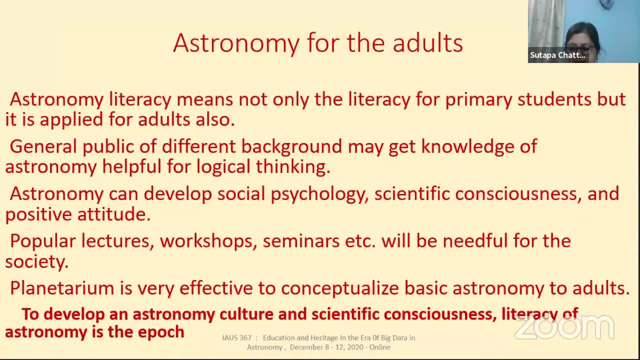 knowledge of astronomy. It develops social psychology, scientific consciousness and positive attitude. Popular lecture, workshops, seminars, visit to a planetarium and heritage astronomical sites will help them to get literacy in astronomy, To develop an astronomy culture and scientific consciousness. literacy of astronomy is the epoch. On behalf of Institute of Astronomical Studies, we want to promote 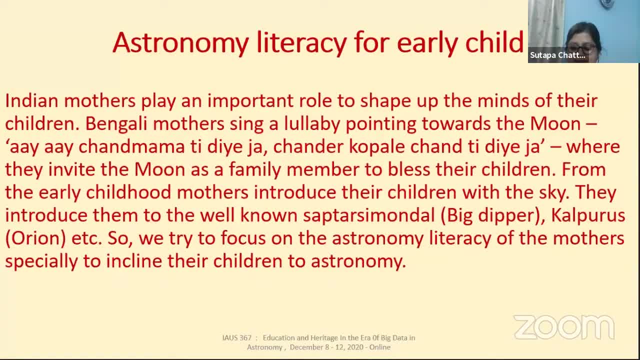 astronomy literacy for early child. Indian mothers play an important role to shape up the minds of their children, And partly mothers sing a lalabi pointing towards the moon. That is: aye, aye, chandmama tee die jaa, chandher kaupalaya, chand tee die jaa. Thus they introduce their 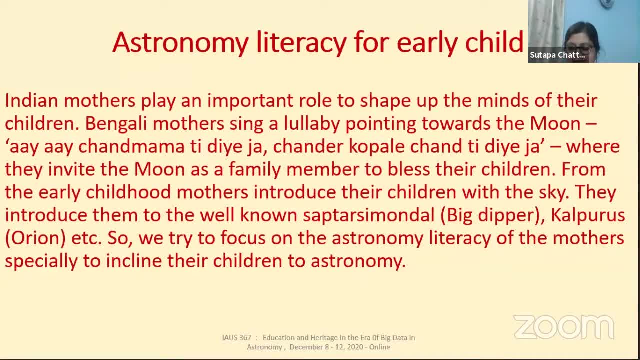 children with the sky and moon Years later, with Shaptoshi Mandal, that is the Big Deeper, and Kalpuruja, that is the Orion. So we try to focus on the astronomy literacy of the mothers, specially to incline their children to astronomy. 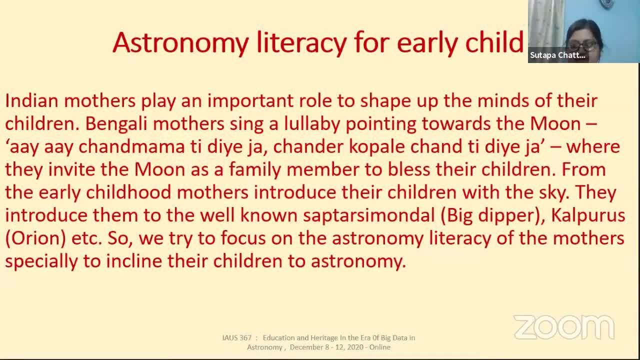 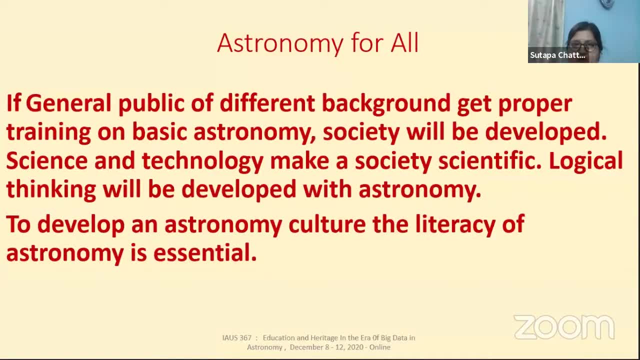 A mother can influence her children like no other can. that we think Our call is astronomy for all. If general public of different background get proper training on basic astronomy, society will be developed. Science and technology make a society. scientific Logical thinking will be developed with astronomy To develop an astronomy culture. 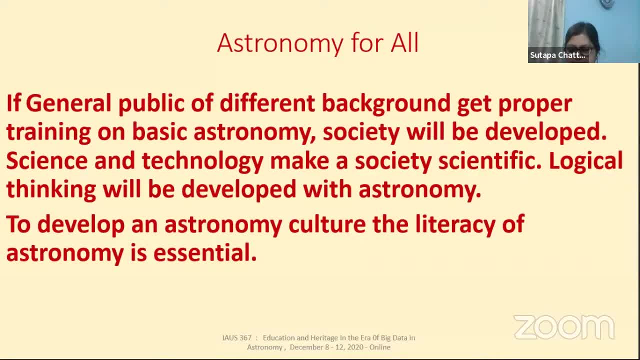 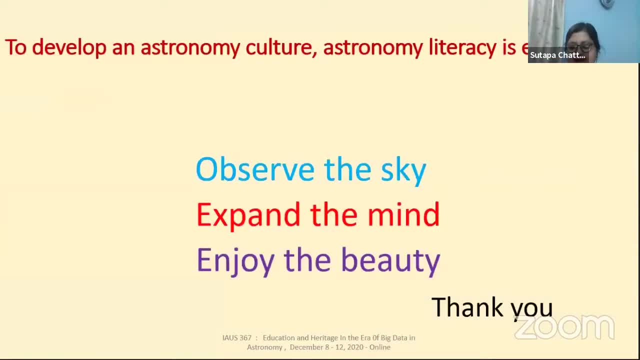 the literacy of astronomy is essential. Institute of Astronomical Studies believes it from heart and we say: observe the sky, expand the mind, enjoy the beauty and celebrate life, Thank you, Thank you very much, Suttapa. So we've got plenty of time for questions. I think we've had five. 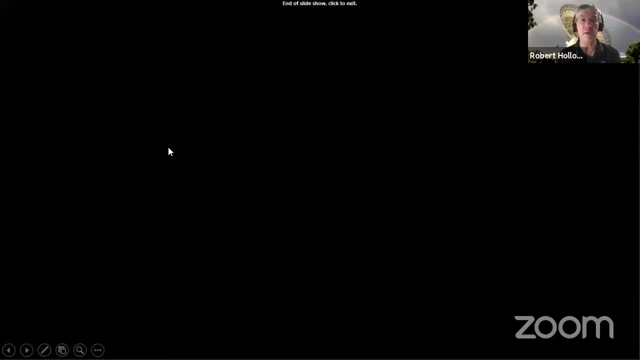 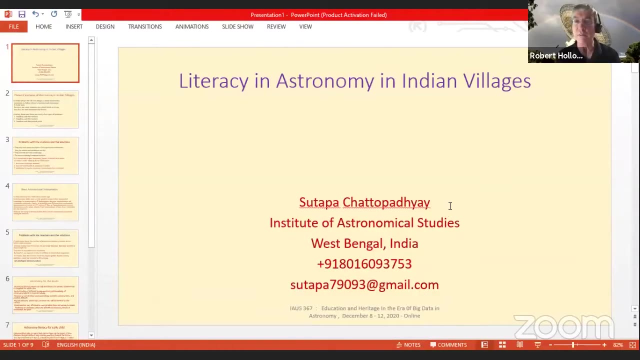 all very different, diverse and excellent talks. I've been trying to keep on top of the chat and the Q&A. I know some of the questions have already been answered, but I've got one here for Basilio. You mentioned a planetarium show. 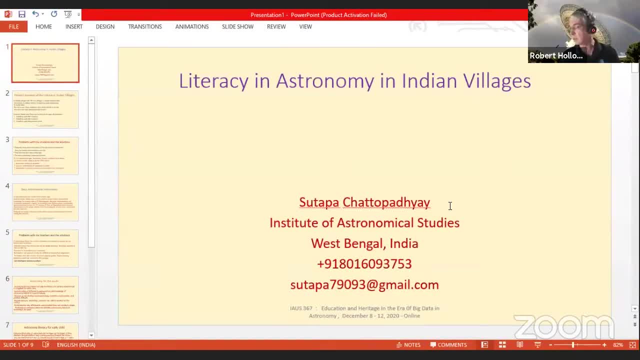 and Beatrice wanted to know if that was available for all. please, Sorry, Please repeat the question, So that one was for Basilio. Can you repeat the question please? The question was the planetarium show you mentioned. Is that available? 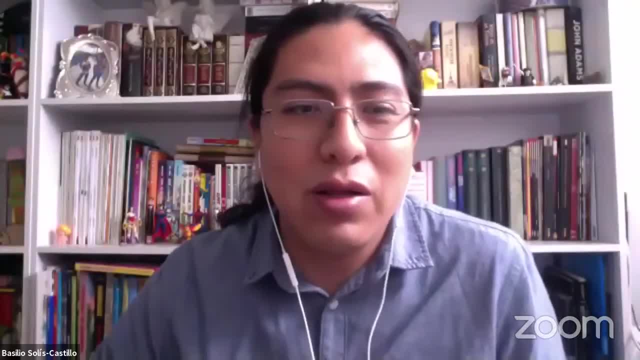 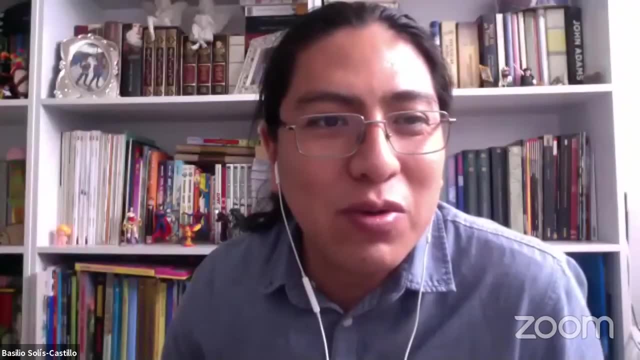 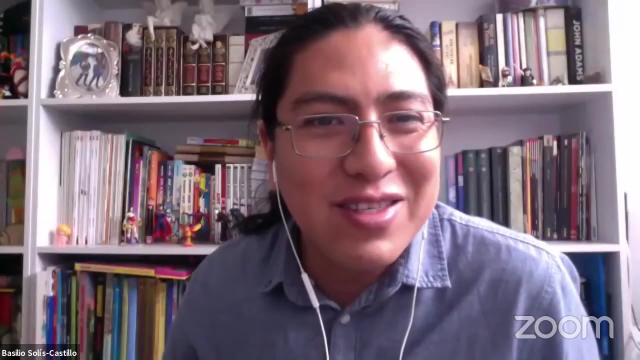 Okay, Yeah, yeah, It is well nowadays, for the sanitary situation is close, but it is possible to we have this old card size projector from the 70s and it's now it's united with all the digital systems. 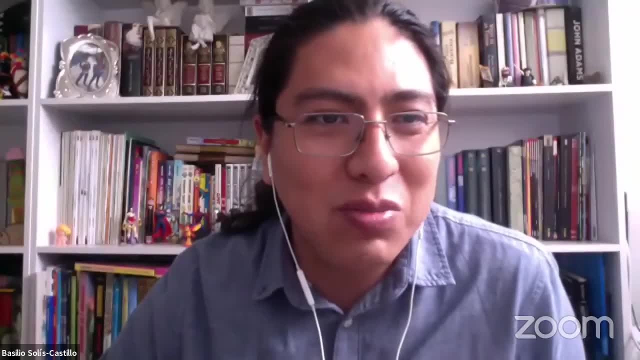 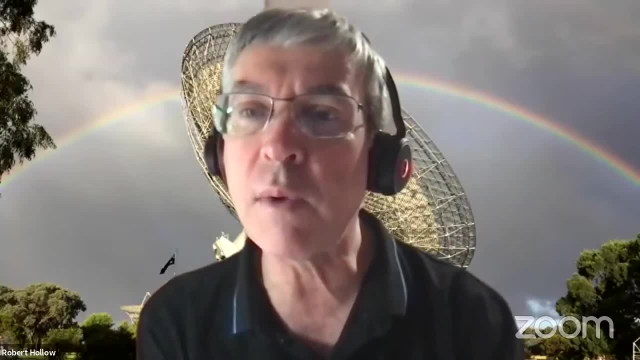 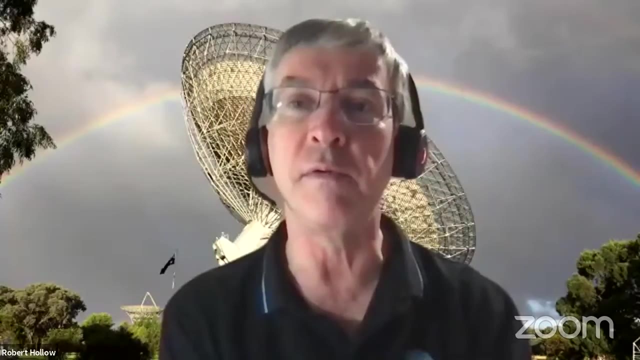 So I think it's really interesting experience to go to this planetarium. All right, Okay, I'm just trying to see We've got a few others here. So one of the questions came up about your talk, Franz, stressing the value of the history of astronomy. 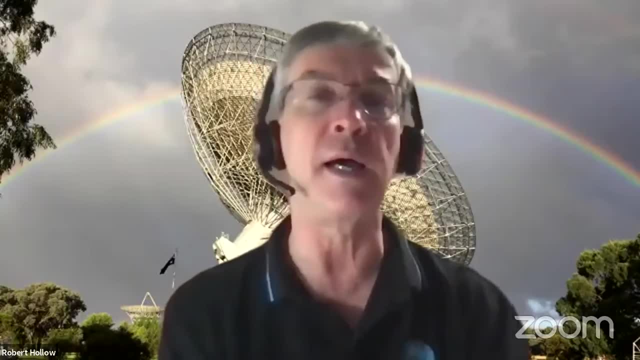 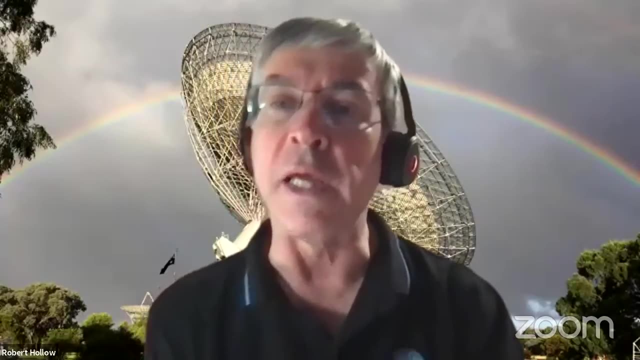 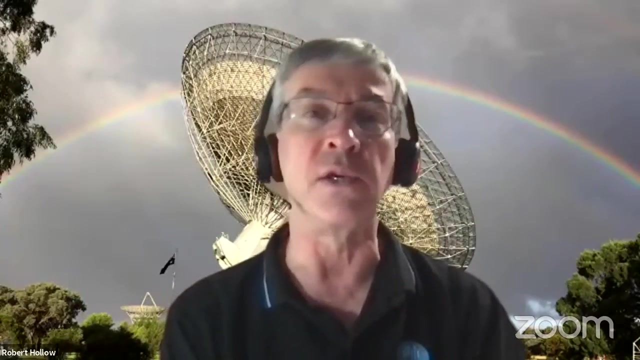 but it also then mentioned the fact that astronomers- well, a lot of the hang on, I'm just trying to get it Here it is- The historic observatories are being forced to redefine themselves, And so they're losing that knowledge as the staff move on. 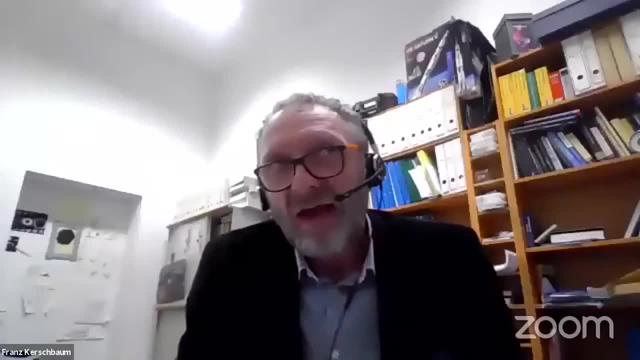 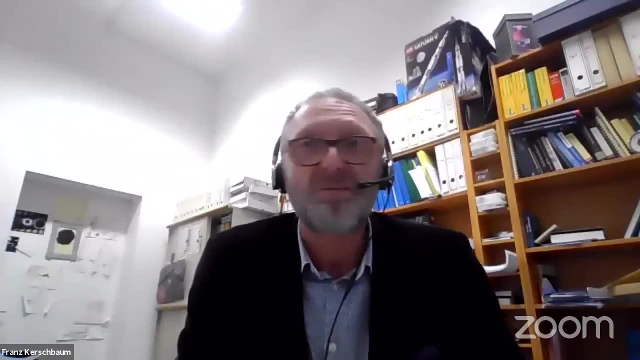 And I'm wondering if you've got any comments around that, Yeah, we had. we had over, I have to say, over decades- the discussion. if we leave the observatory, it would be better to go to a central campus area together with other. 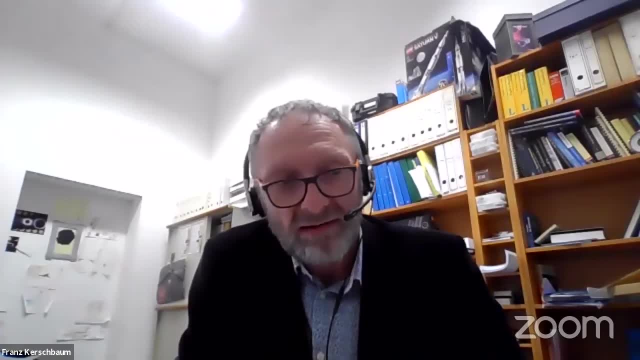 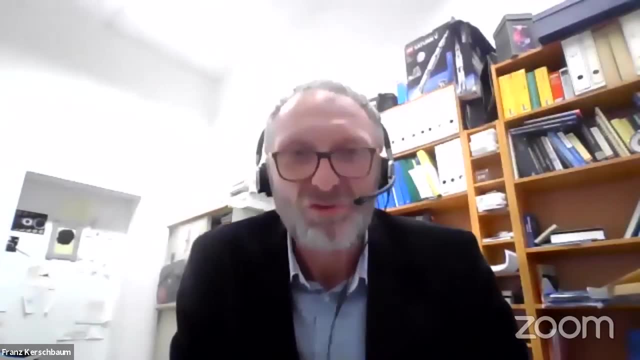 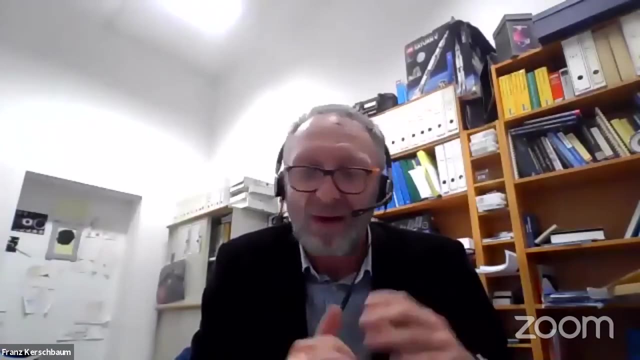 with other sciences and so on, And in the end, of course it turned out that it's better to stay here and we got the observatory renovated because here we can combine, And of course this was the result of many exhibitions and public events. 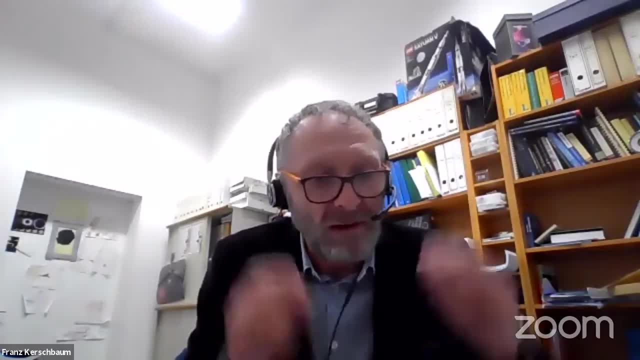 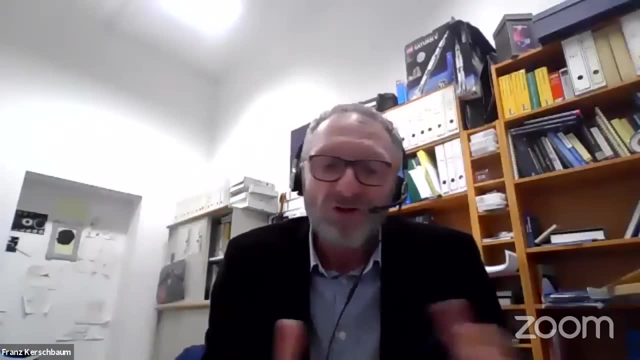 with thousands of people visiting our big observatory, that we can stay here and get it, got it modernized here. So it's not completely finished yet And it's a constant struggle, of course, with the historical instrumentation and so on, but in the end we can could. 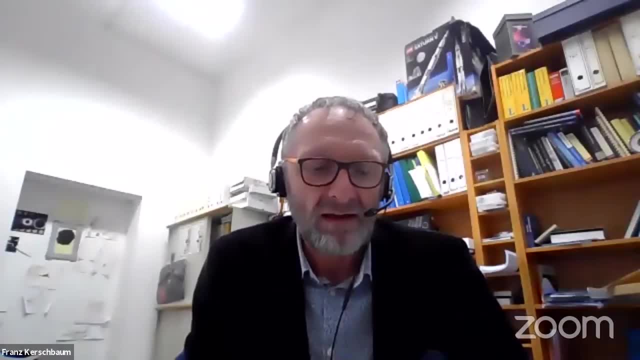 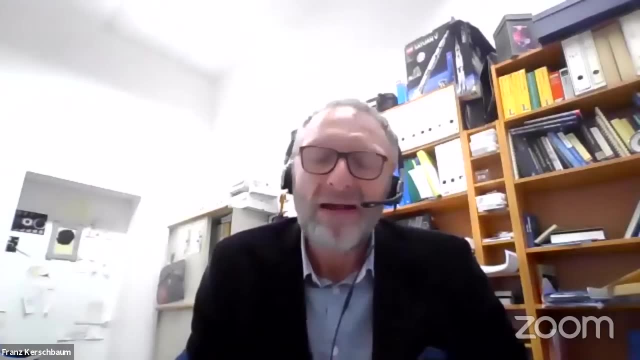 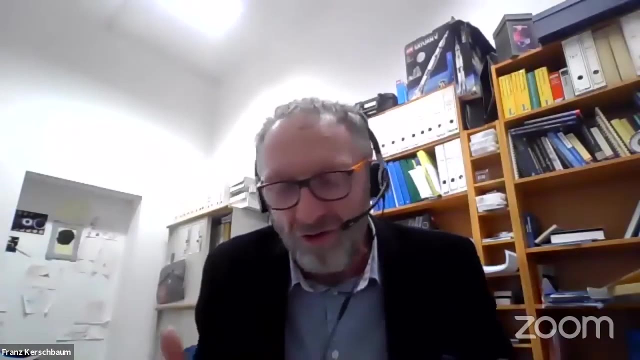 could convince the university that such a big observatory is a value by itself because it shows this historical perspective. And, as I wrote in my answer, you know we have books of all authors, We have first editions of Kepler, Copernicus and so on here and display. 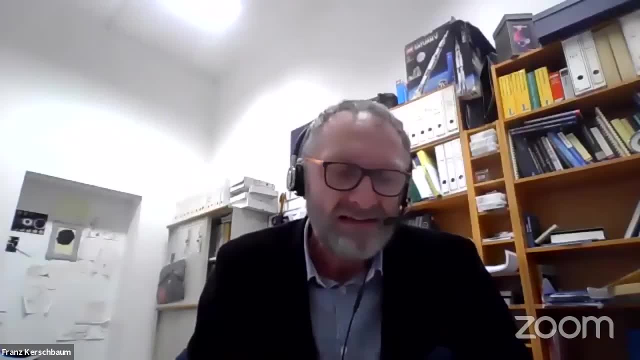 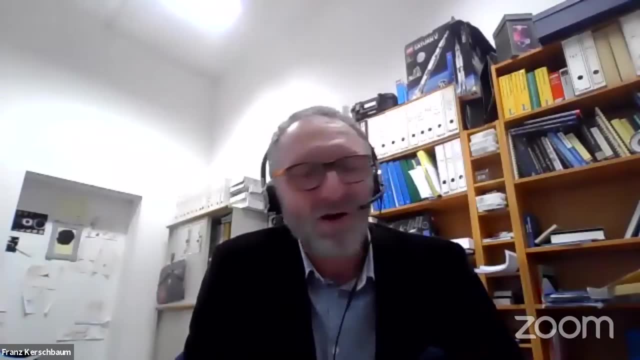 in our museums and so on, and old instrumentation. So the combination of modern science and you know I'm doing I'm doing a lot of space projects- That's my most of my work is is is building space telescopes. 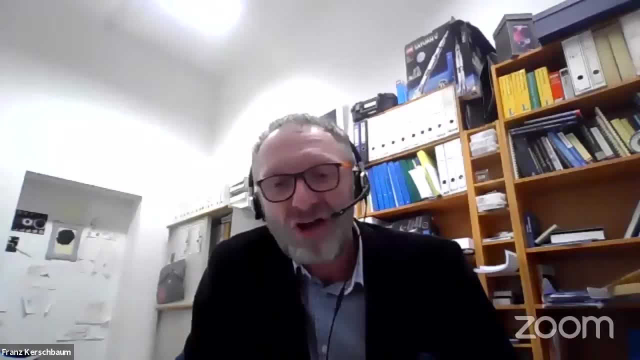 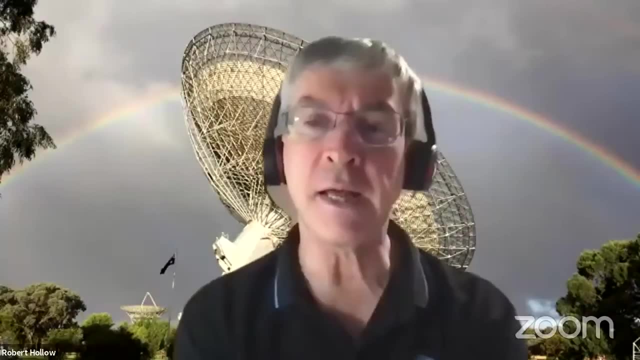 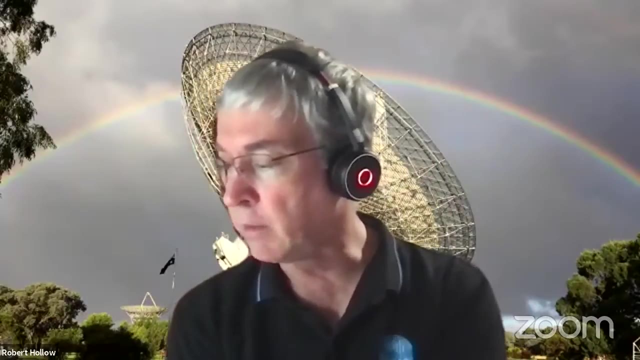 This combination is a good one and it attracts the general public and show that we are standing, to cite something, on the shoulders of giants. So I think that leads into a couple of themes of sort of picking up on. So I know, Basilio, you were showing the spectacular Atacama and the 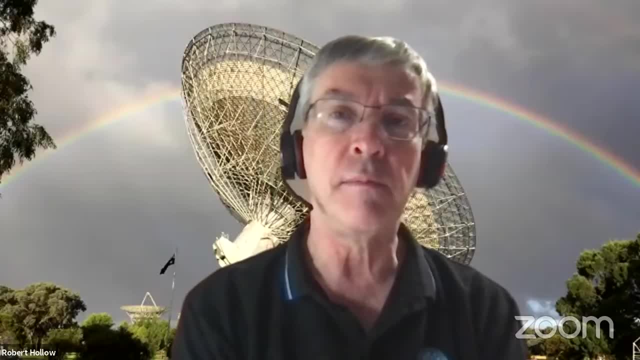 the culture in Chile. But I wonder what do you, what do you see skills and practical skills that there seen now so far to � geopolitically expand our human routing and research account? No, I wouldn't say that any of that. But I think one of the most consistent, 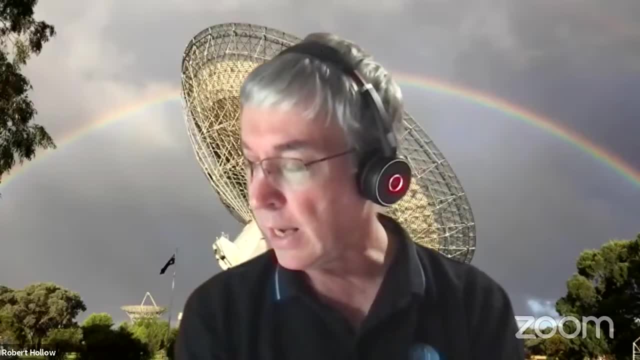 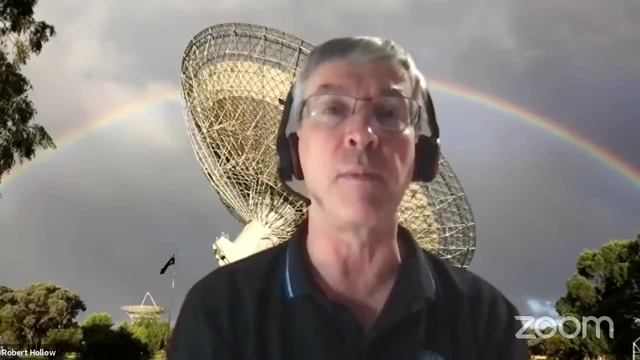 I think the biggest lesson that we've had and also you know what I've heard on the effort with Research Academy over the plenty of field näje and and uh, the the relationship of the Lyndon people with. 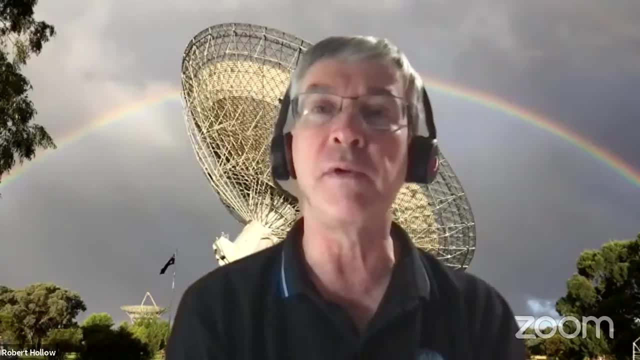 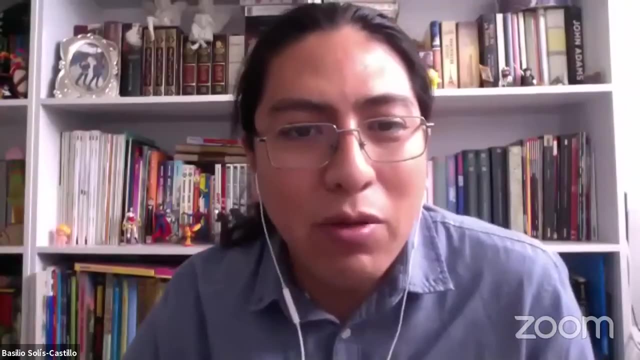 you know mass and used gebe kind of group of aliens in in you know for over a period of time. So that's having done, Yeah. well, my comment is is connected to the how to reach like society or how to do astronomy outreach. 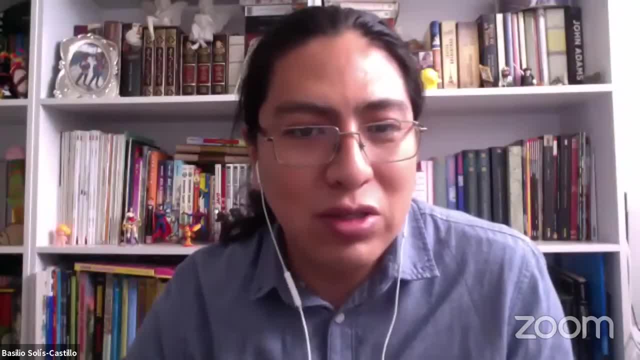 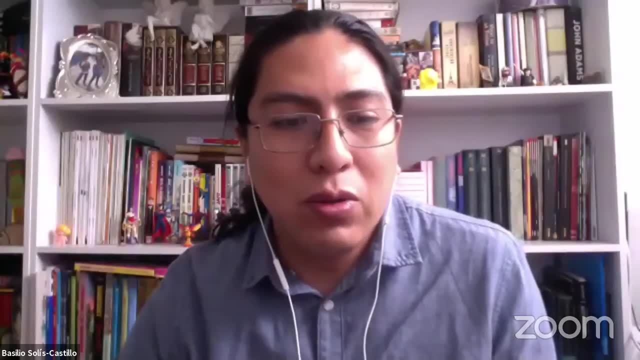 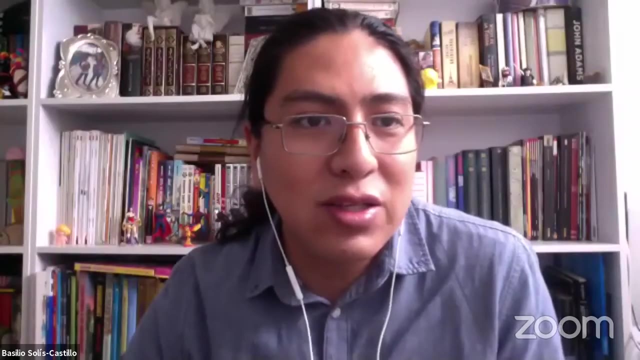 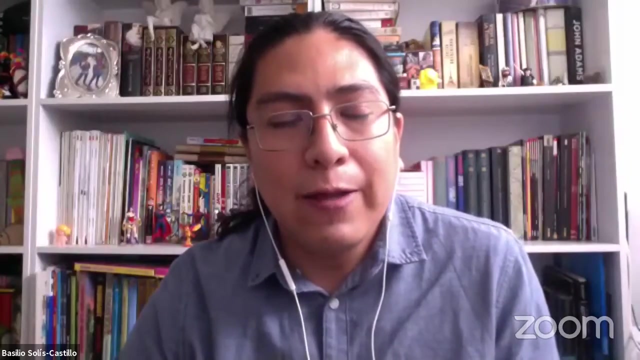 you know. so, talking about, like indigenous tradition and indigenous culture, we, we have this connection with people that is easier for them to to understand, for example, nowadays, astronomy. so i think to rescue this celestial heritage we have is, is is helping us to to reach more people in order to they can. they can reach science in a different way, in a different approach. 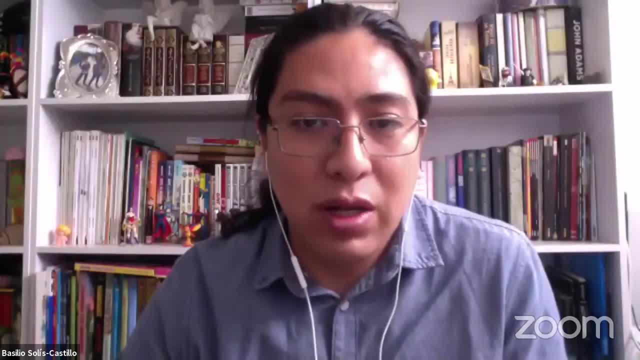 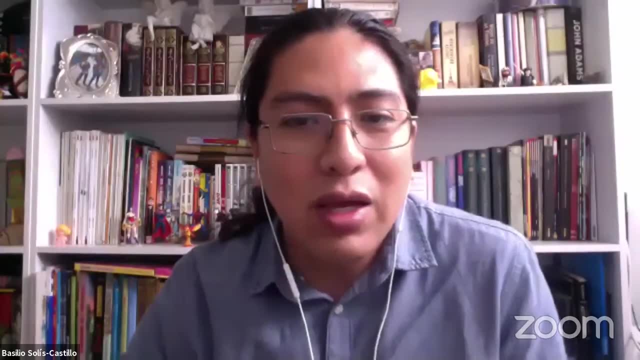 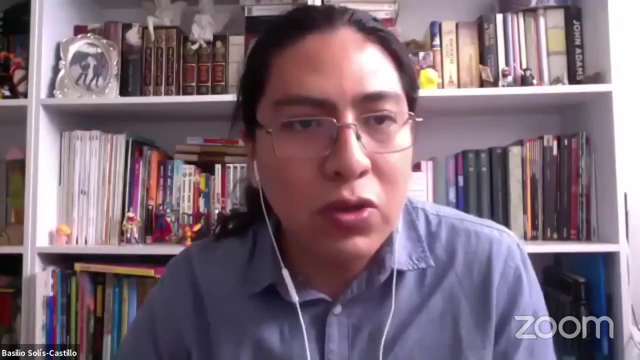 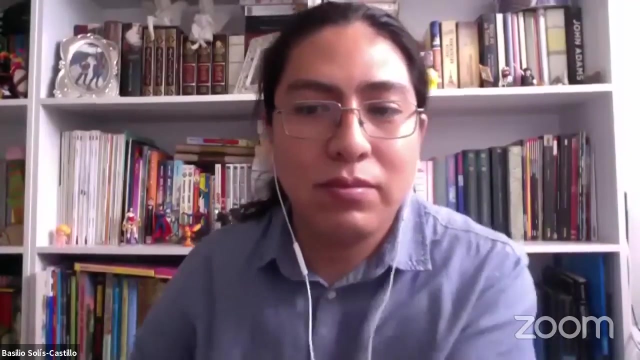 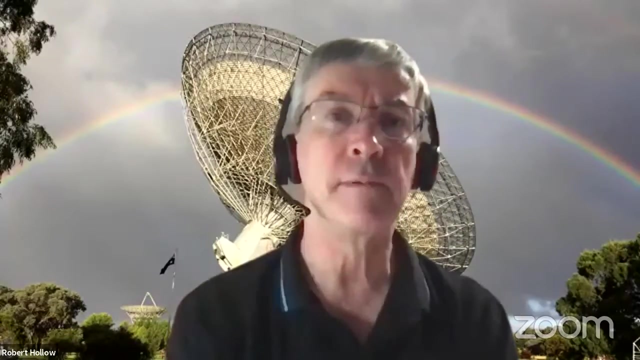 and, of course, they are more interested, like in science, like in other cases. so i think it's a win-win situation. so we learn from our culture and also the people get in touch like more closely, using these uh, these, these um older traditions we have um satapa. do you have anything you'd like to add there? sorry, uh, would you like to comment on? 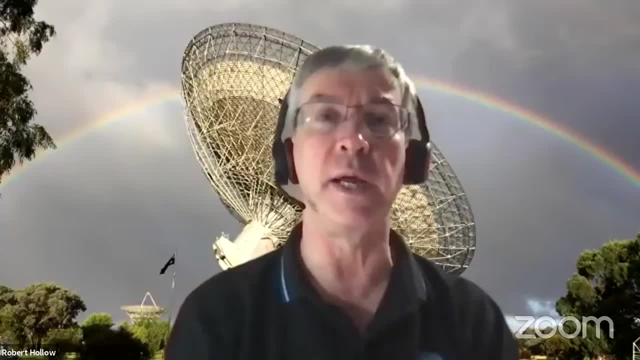 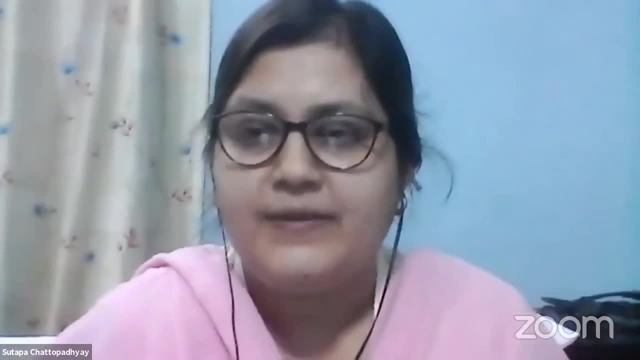 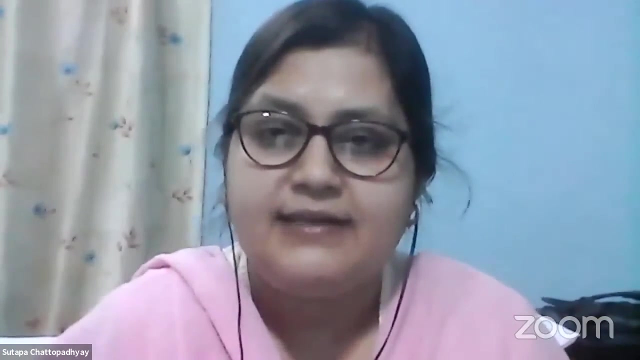 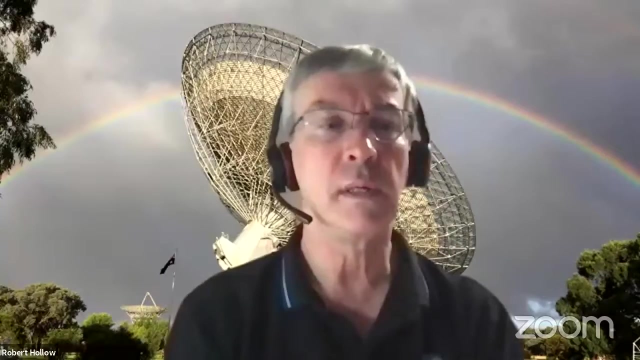 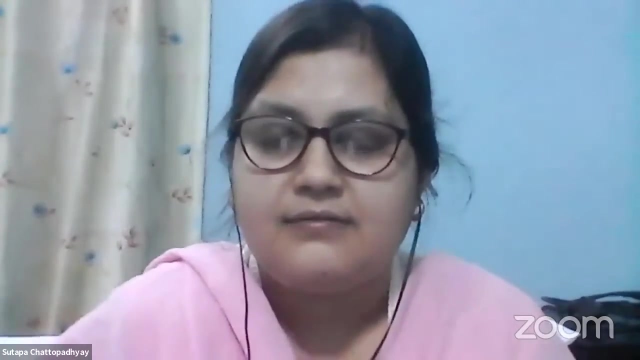 on the, the sort of interplay between culture, history and traditional knowledge. okay, i want to comment. my experience is that the indigenous people have a much knowledge, something they know that we do not know, and by practice, they carry forward this knowledge to their future generation. but nowadays, the, the- what can i say? the tradition is lacking a. 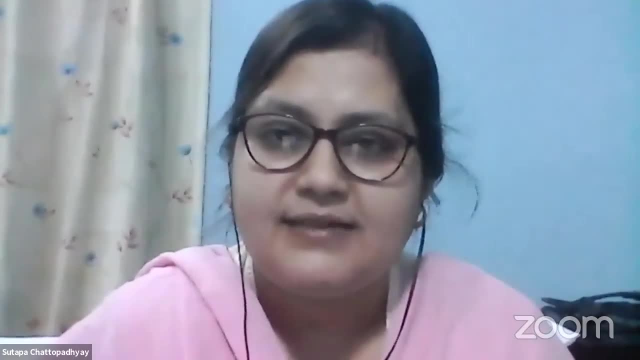 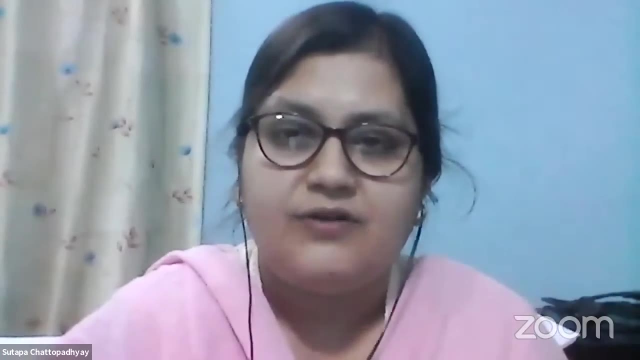 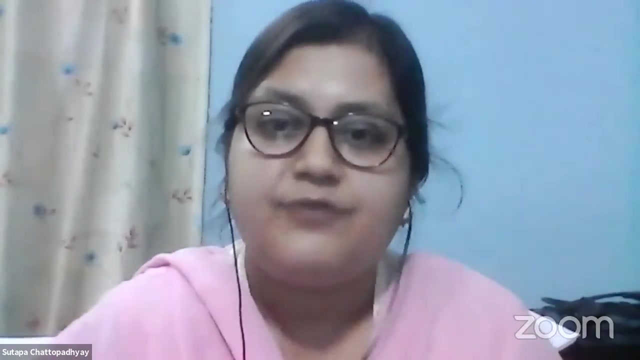 bit, and when we are attracted to modern science, many times we are ignoring our traditional knowledge. i think that's not good for us. we we should try to gain something also from our traditional knowledge and from traditional people's, that i think, and so i said the mothers. 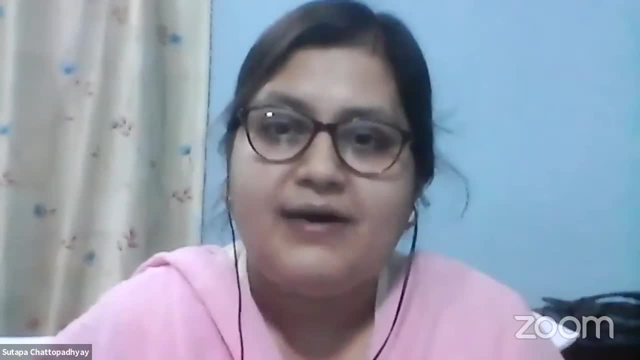 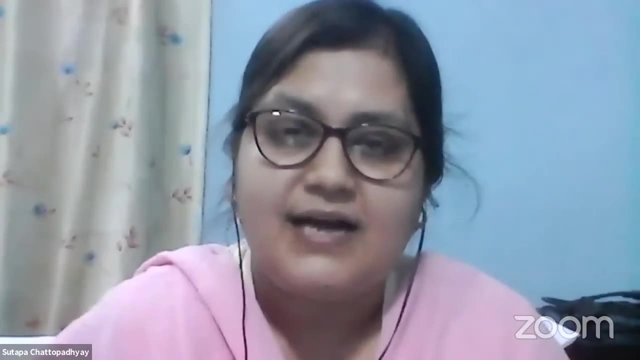 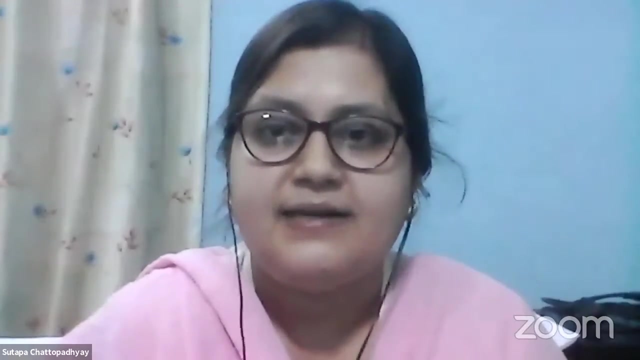 are the great teachers they can. when a mother is knows astronomy, she can train her child to see the sky. as far as i know, that all bengali mothers can do this with their children, and if they can do this, they can also inspire them. inspire them to take future astronomy courses. 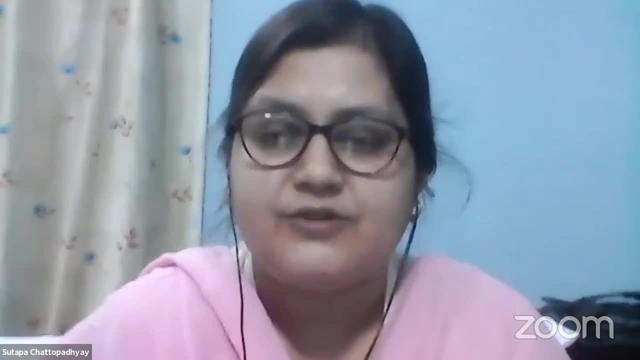 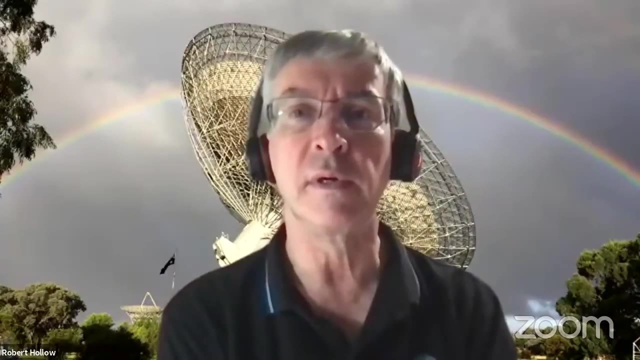 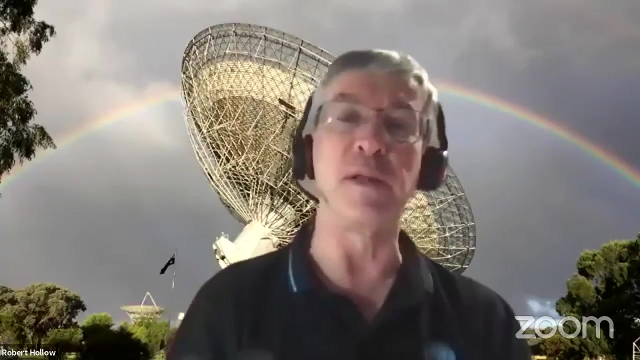 astronomy classes and do something big in astronomy. that i think okay, thank you. um. so, gary, hang on, i'll just. everything just went strange, come back there. um you, you were showing us, i guess, the other end of the spectrum in you know the you know virgo gravitational wave observatories and neutrino. 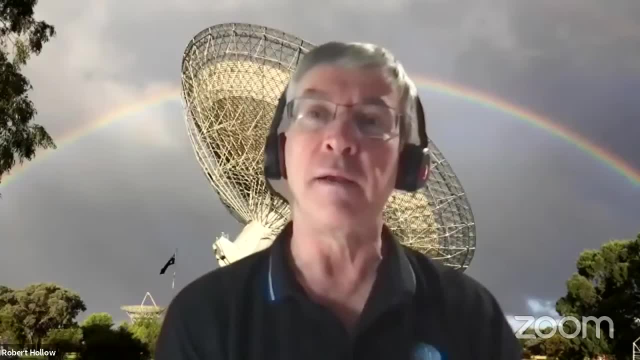 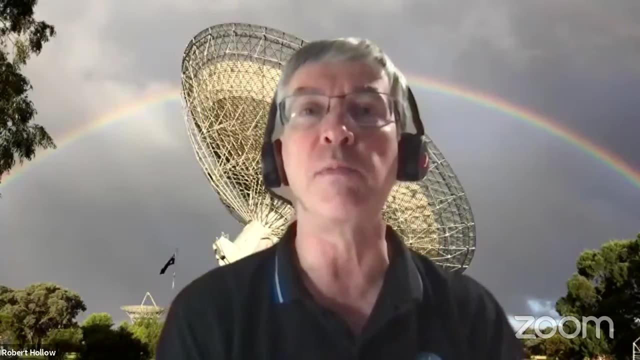 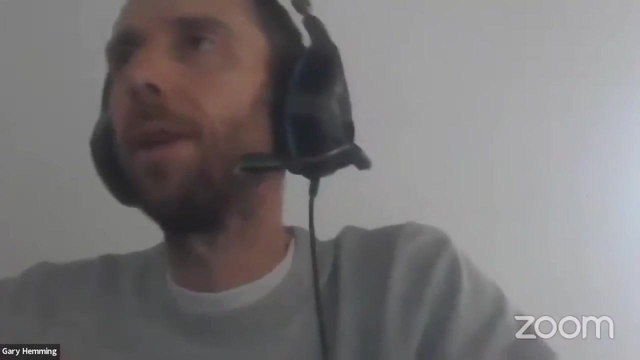 detectors deep in the ocean and, uh, obviously then using citizen science. i was wondering, um, how do you go about evaluating the effectiveness or the engagement of, say, deep hunters or one of the citizen science projects? okay, well, what we're doing in reinforce is- i mean, it's a well-known phenomenon in these kind of online. 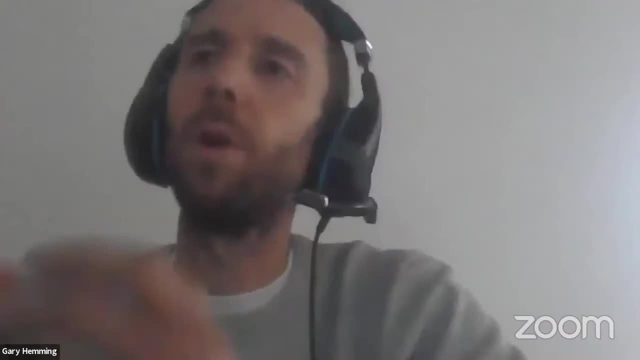 citizen science programs that you will have. when a, when a program is launched, you will have, uh, a significant take-up, uh, and but also a very significant drop-off, um, because inevitably you have, but you end up with a kind of rump core or of users who end up, or of citizen scientists who form your community, uh, and then uh do all of the work. 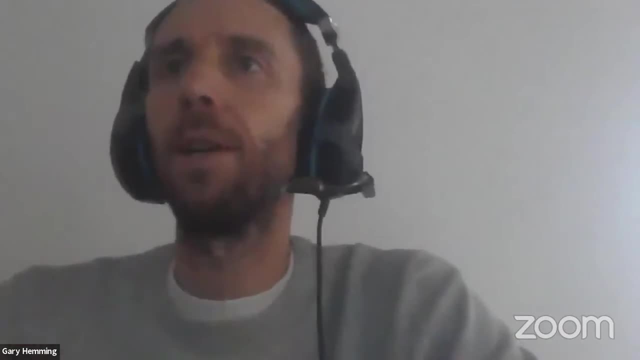 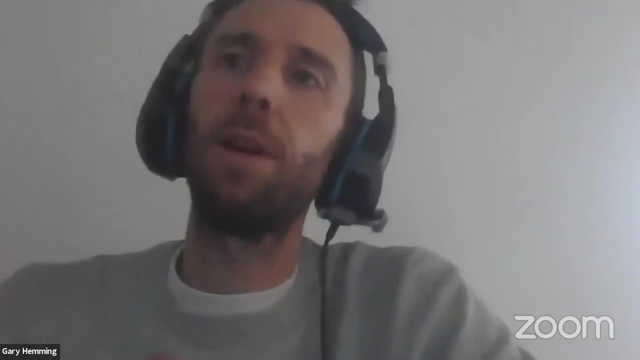 basically, uh, so what we are doing in reinforce to try and help understand this and and understand how we can retain uh, people's interest, is where we have this, this pre and and post sort of staggered evaluation process, where we will be. uh, we, we're already building a community, community of people. 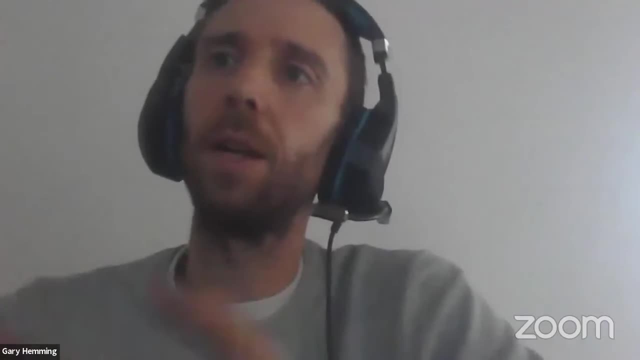 even before we go, uh, with all of the demonstrators online in the middle of next year and we're already sort of pushing people, not pushing them, but we're already pushing people to do things that are going to help them in the future. pushing, let's say, but interacting with people, uh, asking questions, uh, that we can. we can come back. 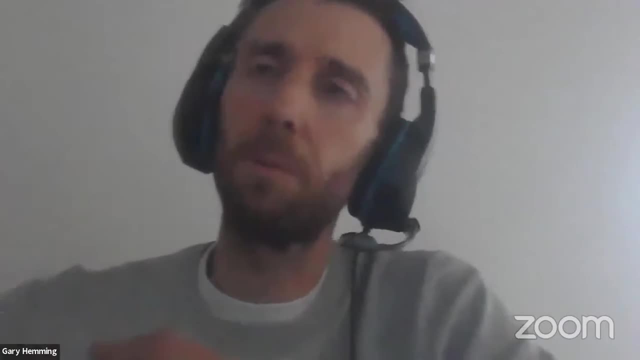 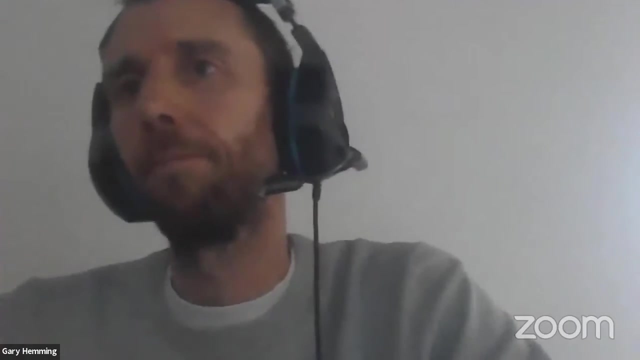 to them again and again and see you know if, even people who drop out of the process and so on. so, um, it's not straightforward, but uh, that's what we're going to try and do. yeah, i think. well, the zooniverse certainly is a great structure for helping with that, and i was involved in radio. 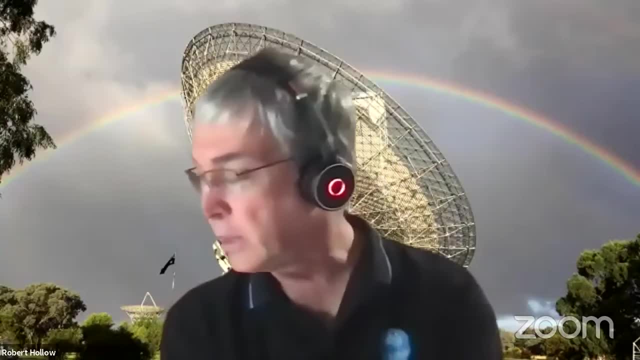 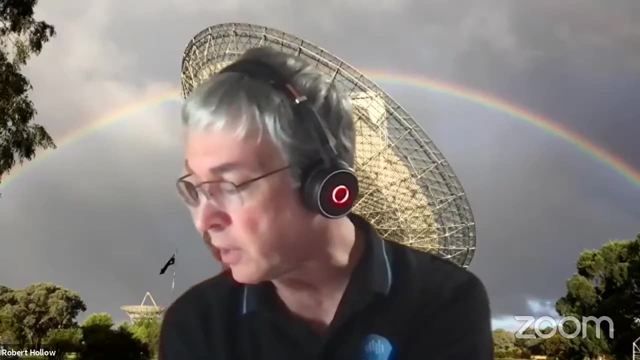 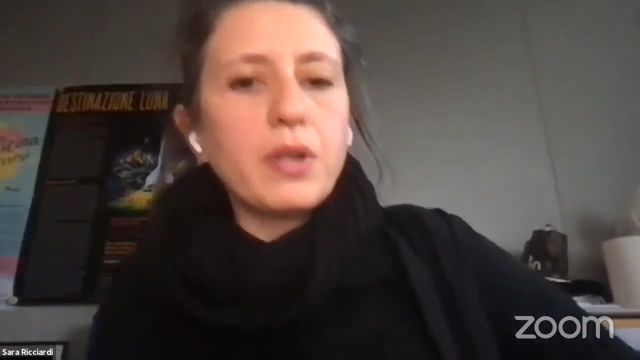 galaxy zoo. um. so, sarah, um, we did have a question for you. i think you may have answered it, but it might be worth sharing more widely. so hugo wanted to know: do you have science theatre in your project? no, actually for the project we work together with Cineteca di Bologna and, uh, it's like a mecca for.